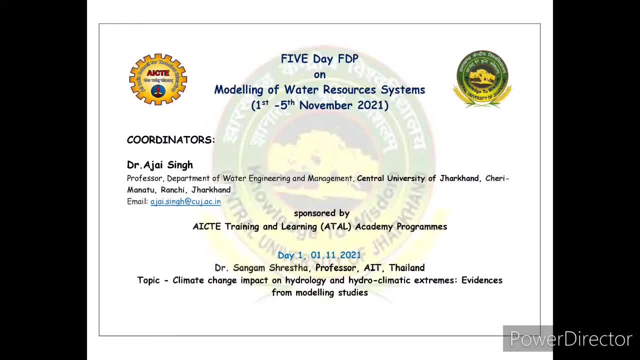 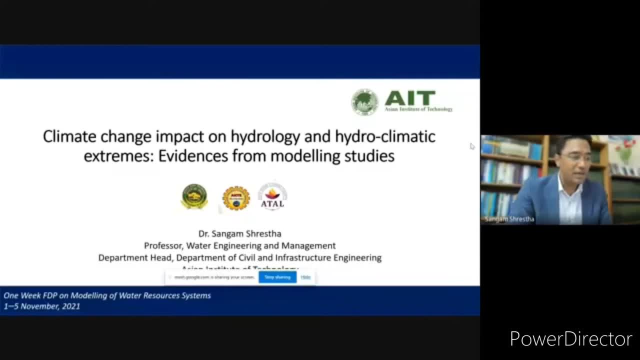 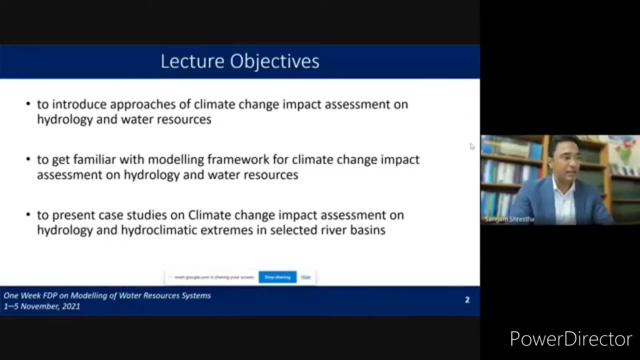 The main objective of this lecture is to introduce what are the approaches available for the climate change impact assessment on hydrology and water resources And also I will try to introduce the modeling framework to assess the climate change impact assessment on hydrology and water resources through a few case studies that myself and some of my students they have 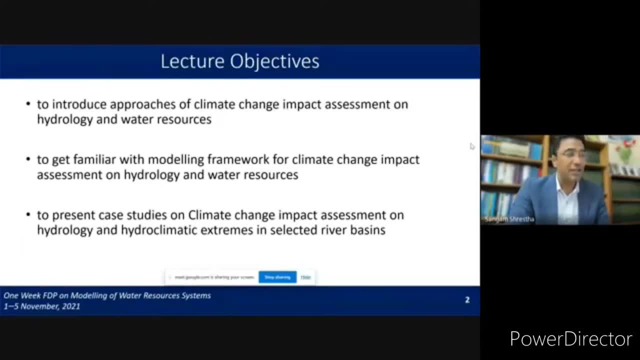 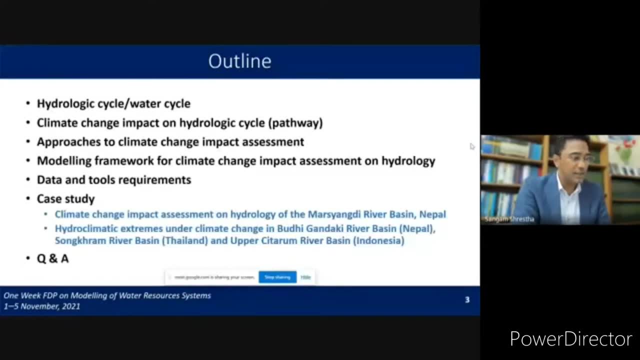 conducted in master's and PhD thesis and some of my project works. So this is the outline of my lecture today. You can see that I will be explaining brief on the hydrological cycle or water cycle. what is the pathway of climate change impact on hydrology and hydrological cycle? 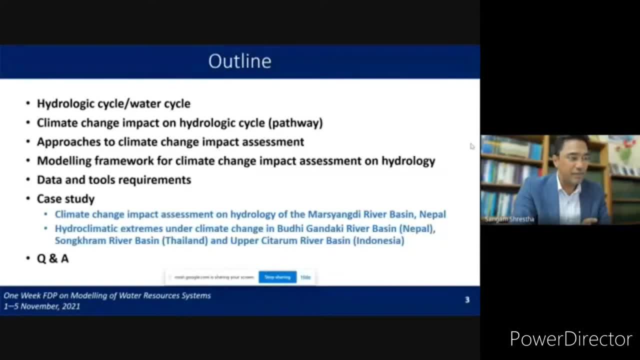 Then I will briefly describe about what are the approaches available for climate change impact assessment on hydrology and water resources. I will also explain about the modeling framework for climate change impact assessment on hydrology and water resources, And probably all the participants would also be benefited from the explanation of what are the data and tools. 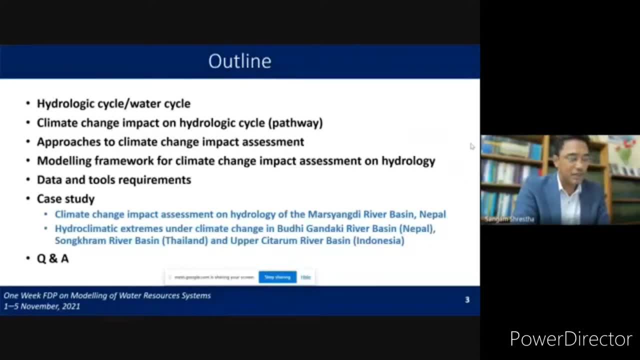 required for climate change impact assessment on hydrogen water resources, And I will finally present the two case studies. One is climate change impact assessment on hydrology of one of the river basins in Nepal called Murshendi River Basing, And the other case study is on: 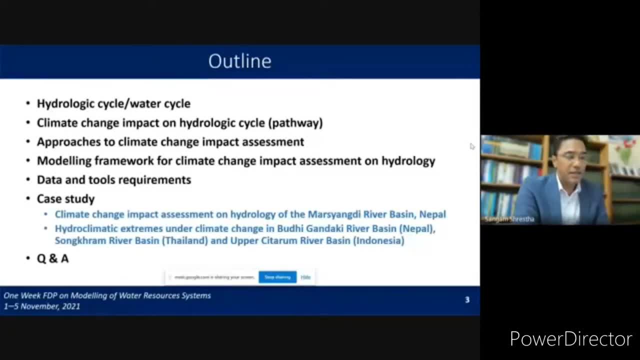 climate change: impact on the hydroclimatic extremes under climate change in Gurigandari River Basin of Nepal, Songkran River Basin of Thailand and upper Sitaram River Basin of Indonesia. Probably I will stop after some of the contents to have more discussion session. 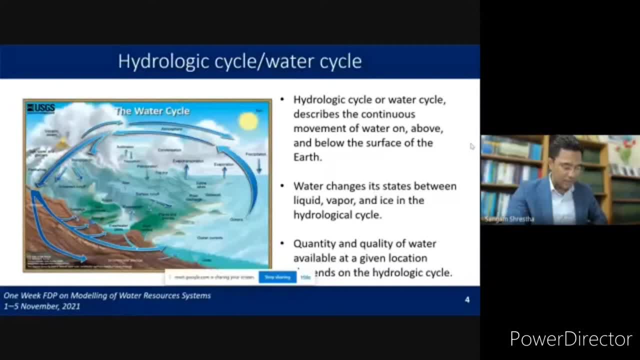 So let me briefly explain about the hydrological cycle or water cycle, because it is very important to understand what is the meaning of the hydrological cycle or water cycle, because the climate change impact on water resources is basically from the impact on the hydrological cycle. 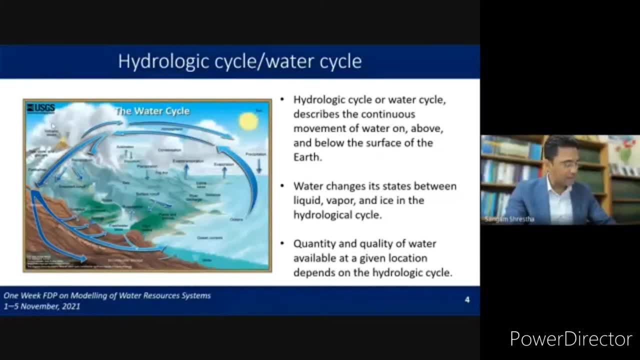 So, as I mentioned to you that it is very important to understand about the hydrological cycle or water cycle, to understand how the climate change impacts the environment. So the hydrological cycle is also called as water cycle and it describes the continuous movement of water in our earth and the water changes its states in the hydrological cycle. 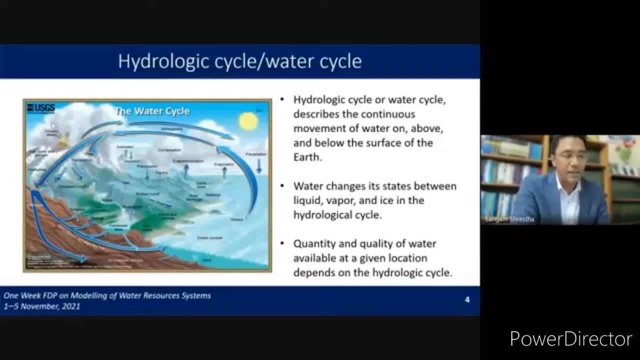 For example, water change its state from A liquid state to vapor state and also the vapor state to liquid state, similarly from liquid state to the solid states in the hydrological cycle. So it means that the water moves from one storage to another storage through various 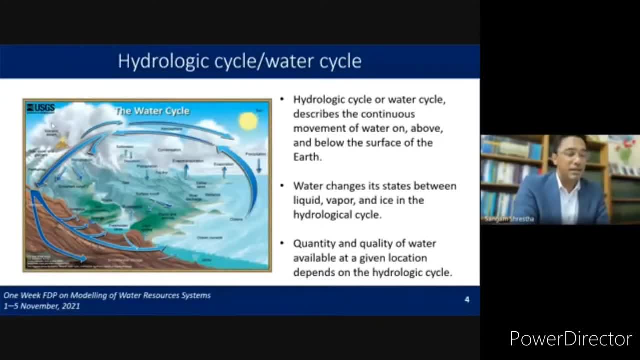 hydrological processes, and these processes are, for example, the evaporation, condensation, etc. The precipitation, the surface runoff, infiltration, groundwater and finally it goes to the ocean, and the cycle repeats continuously. So the availability and the quality of water in any location depends on the hydrological 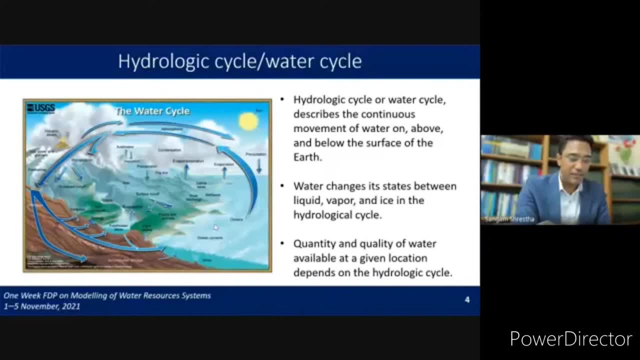 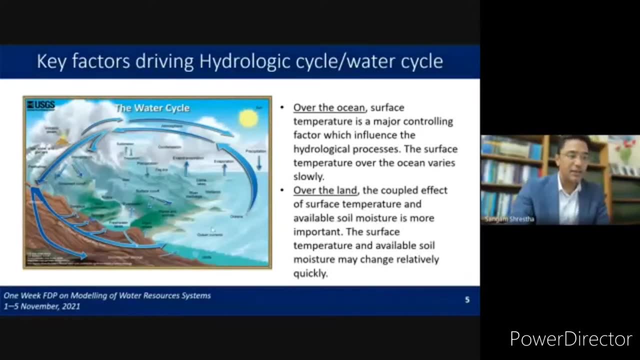 cycle of that hydrological cycle. Okay, So let's get into the hydrological unit. There are two key factors that drives the hydrological cycle or water cycle in our earth. So over the ocean, the surface temperature is a major controlling factor which drives. 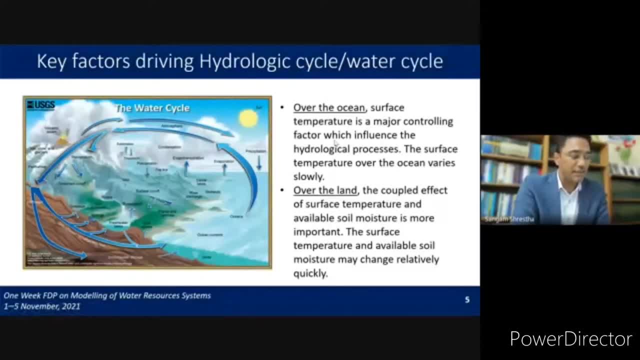 the all hydrological processes and the surface temperature over the ocean varies very slowly. Over the land there are two effects that drives the hydrological cycle or water cycle. One is the surface temperature and the other one is the available soil moisture And, unlike the over ocean, the surface temperature and available soil moisture may change relatively. 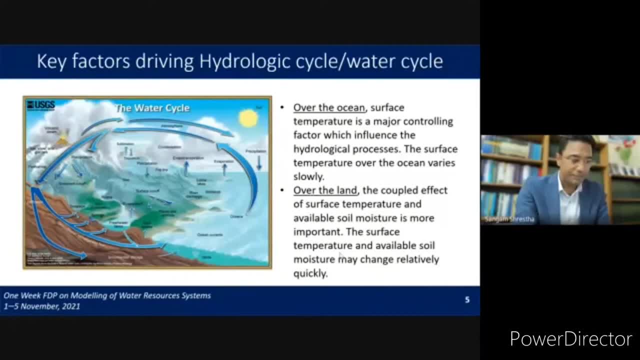 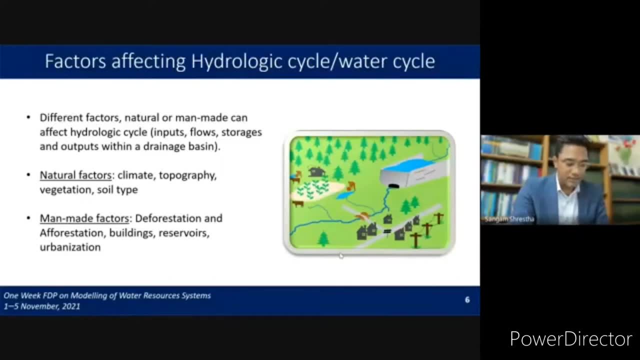 quickly compared to the over the ocean. Okay, Okay, So basically there are two factors affecting the hydrological cycle or water cycle, And they are natural factors and man-made factors. So the natural factors include the climate, topography, vegetation and soil type. 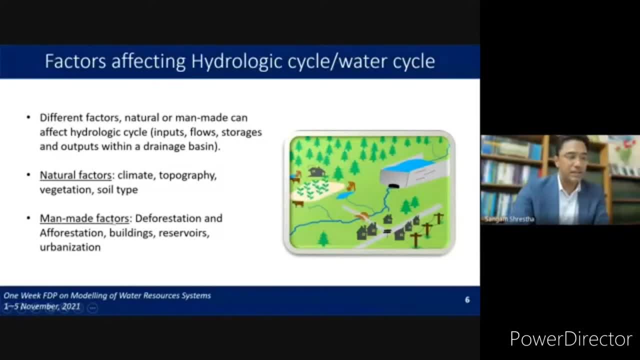 And the man-made factors which affects the hydrological cycle are deforestation and afforestation, construction of the buildings, construction of the reservoir, land use and land cover change such as urbanization. So, since the topic of this presentation is more on climate change impact on the hydrology, 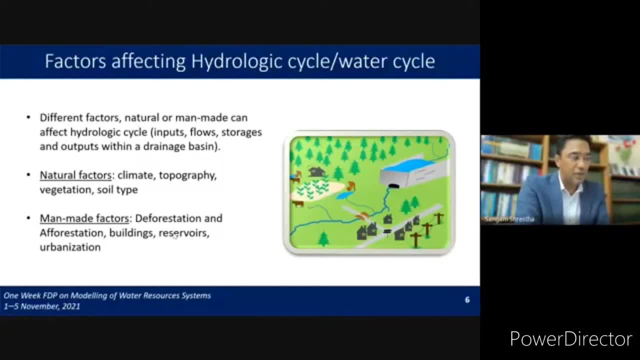 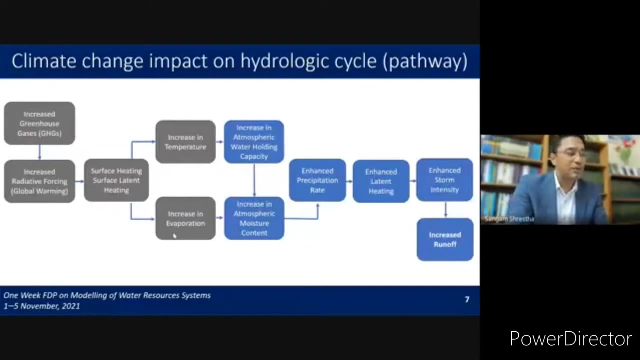 and water resources. I'll be talking more on how the climate change impact the hydrology and water resources of a given river basin, Okay, Okay. So first of all, I'd like to talk about the impact of climate change on the hydrological 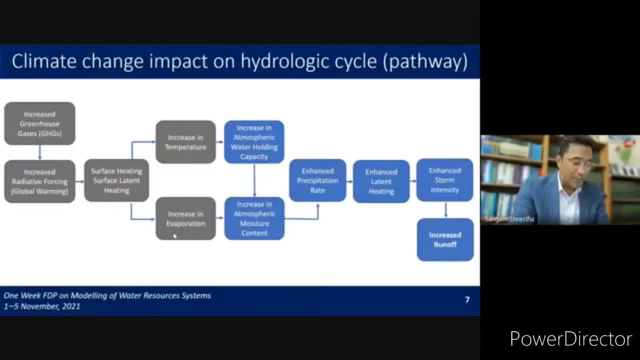 cycle or water cycle. So before that I want to explain a little bit on what is the pathway of climate change impact on the hydrological cycle or water cycle. So all of you know that there is increase in the greenhouse gas emission And with the increase in the greenhouse gas emission there is increased concentration. 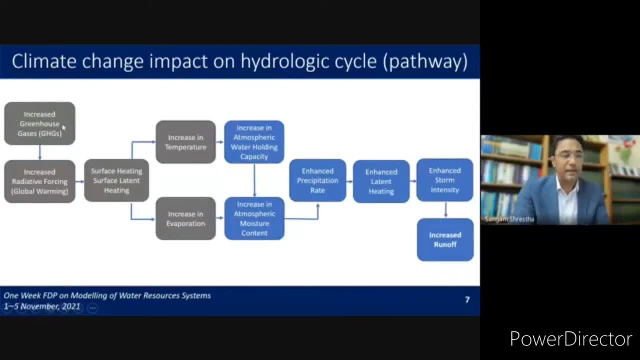 of the greenhouse gases in the atmosphere, such as carbon dioxide, nitrous oxide, sulfur dioxide and so on, And because of the increase in this kind of concentration of the greenhouse gases, there is increased in the radiative forcing of the earth, which is also called the global warming. 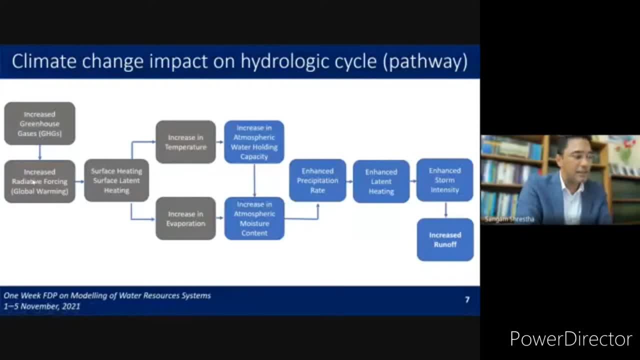 And because of this global warming there is heating of the atmosphere And also the increase in the surface latent heating, And because of this process there is increase in the temperature of the atmosphere And because of the increase in the temperature there is also increase in the evaporation from. 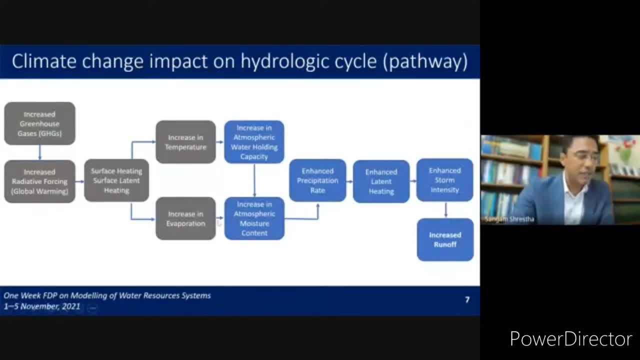 the ocean, land surface and also the vegetation. So there is a physics behind it, Okay, And you know the temperature change and then also the atmospheric water holding capacity. So if there is an increase in the temperature of the atmosphere, it also increases the atmospheric. 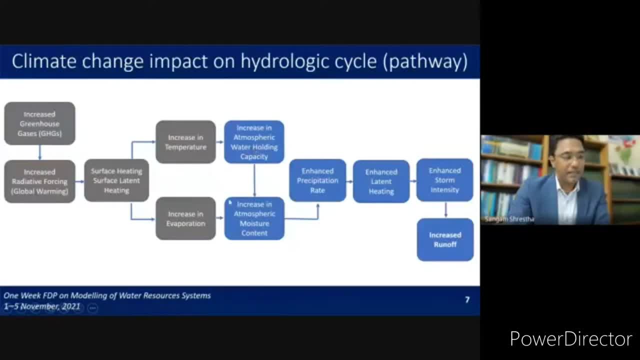 water holding capacity. And with the increase in the evaporation there is also increase in the atmospheric moisture content. So higher the temperature of the atmosphere, Higher the moisture holding capacity of the atmosphere. and all of you know that atmosphere cannot hold more water for more than five or six days. then it has to discharge water. 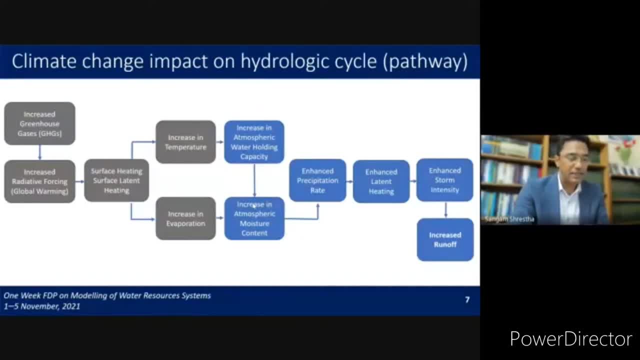 either over the ocean or land surface and vegetation. So it means that with the increase in the temperature of the atmosphere, the hydrological cycle Speed up is occurring And that will, you know, enhance the precipitation rate. Again, there is more moisture available in the atmosphere. 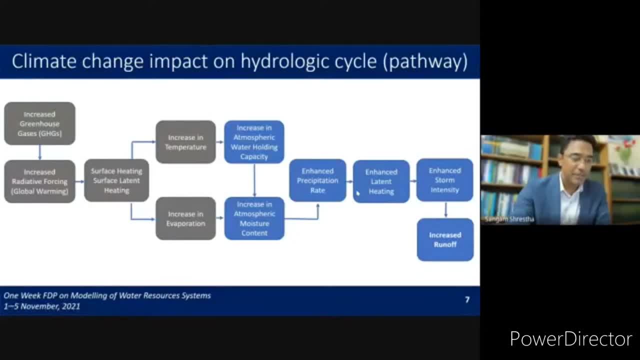 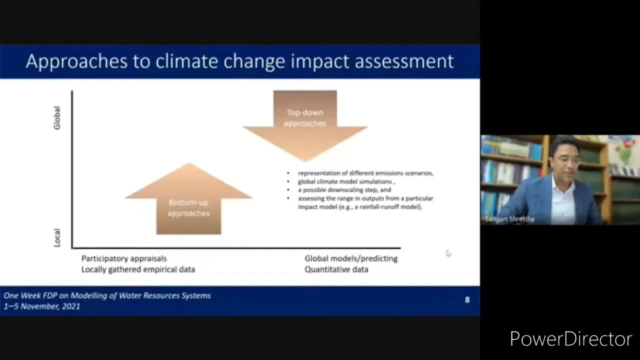 And again, you know this process continuously happens And that will also influence the hydrology or water resources of any given location. So, as I mentioned that Climate change impacts the hydrology and water resources of any given location, It can be watershed. 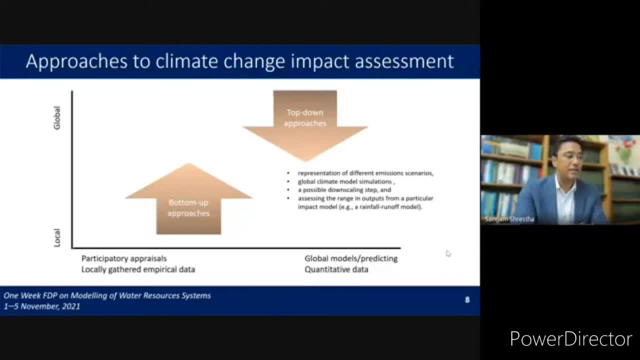 It can be river basin and so on. So there are basically two approaches available to conduct climate change impact assessment on the hydrology and water resources, And these are two approaches. One of the approaches is called top down approach And the The second approach. 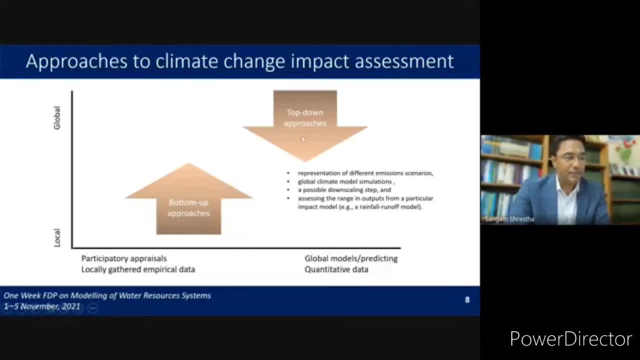 Is called the bottom up approach. So in the top down approach this is basically, you know, take stop study, where different type of emission scenario will be constructed And then those emissions scenarios will be fed into the climate models, basically general circulation models or global climate models. 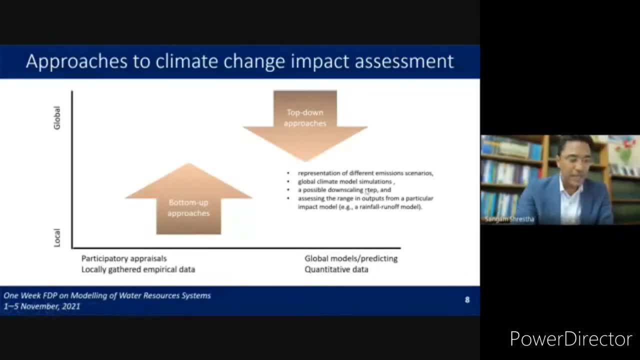 And from there We construct the future climate scenarios. And these future climate scenarios are fed into the hydrological model or any other you know water resources systems model to assess the impact of climate change on hydrology and water resources. So this is a approach called a top down approach in the climate change impact assessment. on 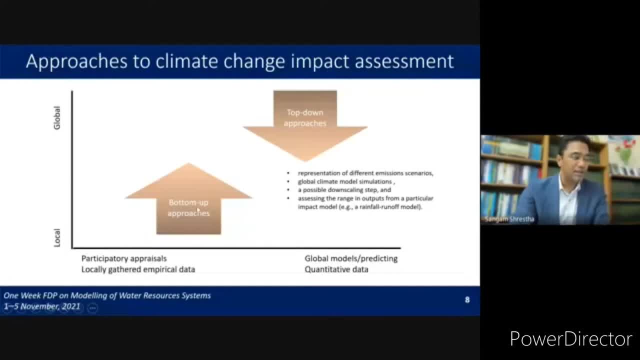 the hydrology and water resources. On the other hand, there is another approach, Called bottom up approach, and this bottom up approach is basically, you know, participatory approach, where we try to find out what are the risks to the water resources systems. 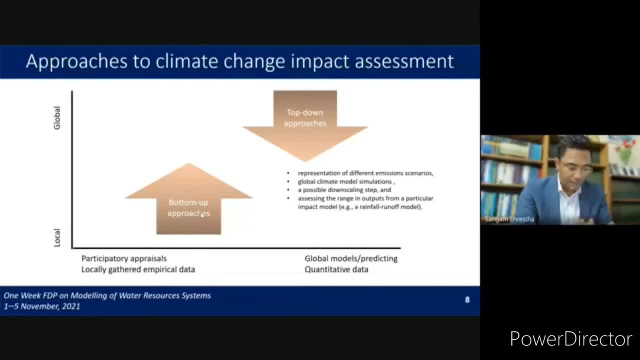 And we try to, you know, take the information given by or available in the particular area. then We use those information to assess the climate change impact on the hydrology and water resources. Unlike the top down approach, this bottom up approach is widely used by the communities. 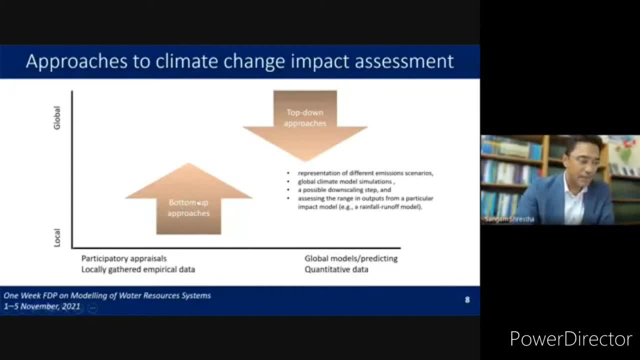 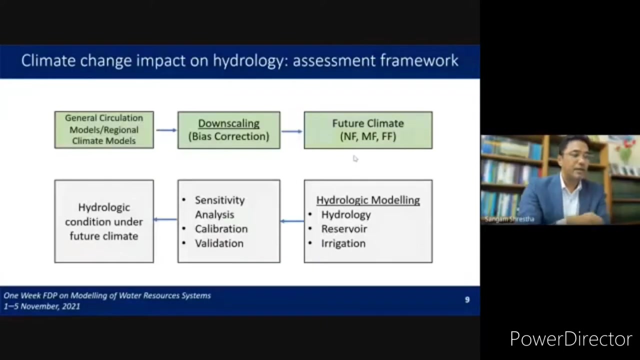 which are conducting the climate change vulnerability assessment or climate change adaptation assessment. So in this study, I will focus more on the top down approaches for climate change impact assessment on the hydrology and water resources. Okay, so this is the general modeling, the framework for climate. 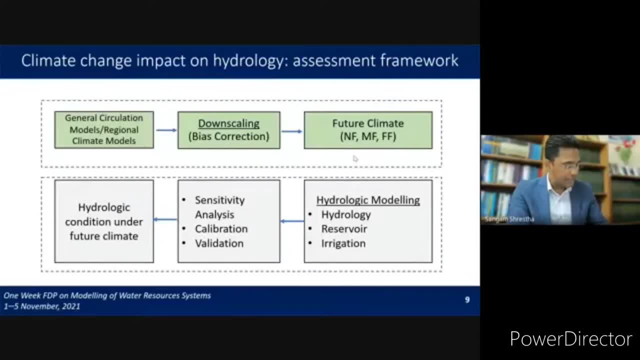 Actually, This is a two step process. In the first step, we generate the climate change scenario. Okay, Professor, as I can, you hear me? Yes, not clear. Okay, I think my internet connection is not stable, So you can hear me. 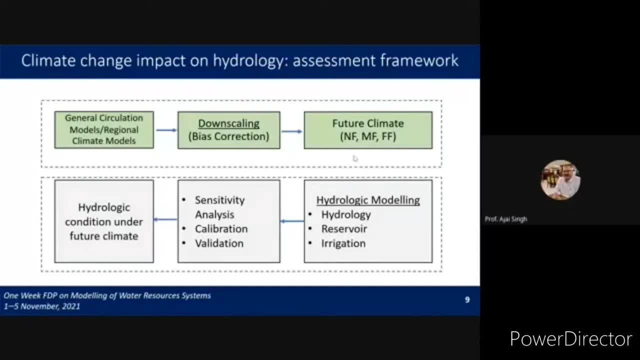 That's fine. Yes, Okay, so the modeling assessment framework here is a two step process. In the first step, we construct the future climate scenarios, Or in other words, we try to forecast or we try to project how the climate will change. 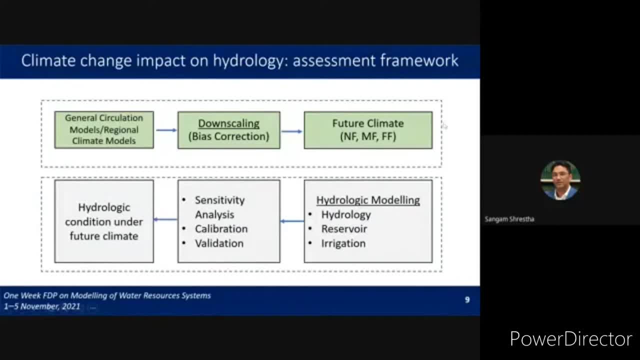 in the future, For example, how the temperature will change, how the rainfall will change and how the other you know climatic parameters will change in the future, Because these future climate is necessary to assess the- you know- climate change impact. 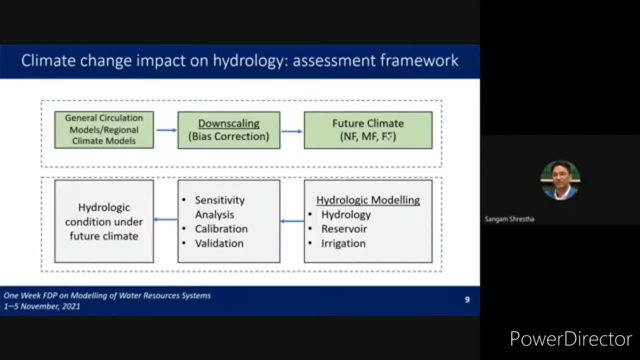 on the hydrology and water resources. So in the first step, we construct, we project or, you know, we create the future climate scenarios. So there are several again techniques to create the future climate scenarios And one of the techniques is use the data of the general circulation model or regional. 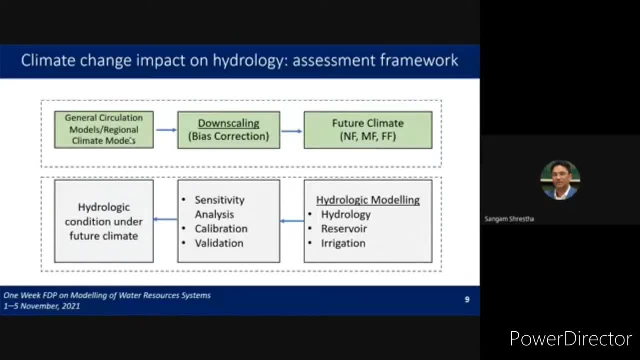 climate models Because these are the main source of the future climate data. So these climate models have future climate data up to 2100,, 2200, even 2300. Okay, Okay So, but the climate data from the general circulation models or regional climate models, they cannot. 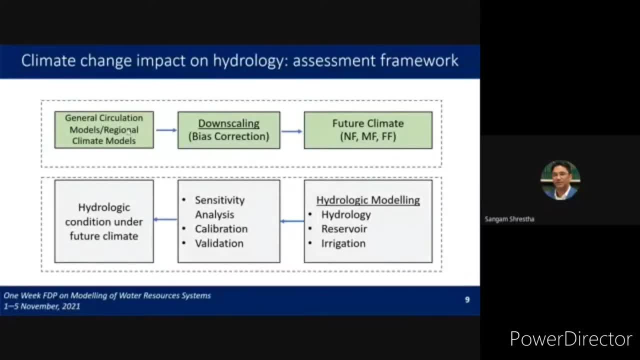 be used directly to assess the climate change impact on the hydrology or water resources at the local scale or the basin scale. So what we need to do is we need to, you know, translate the data or climate data of the general circulation model, GCMs or regional climate models, into the local scale by a process. 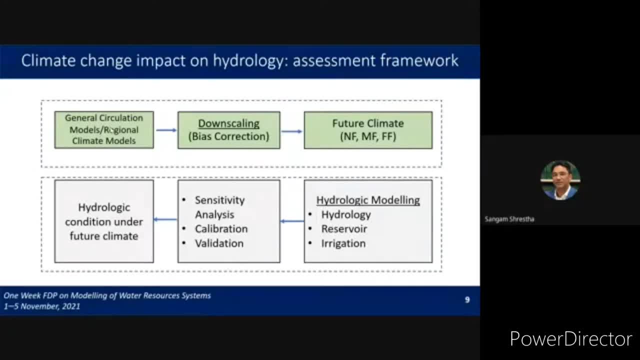 called downscaling or bias correction, Because the general circulation models or regional climate models. they usually projects the climate data at the very, you know, bigger scale and also the coarse resolution. But the impact assessment is still in progress. Okay, Okay. 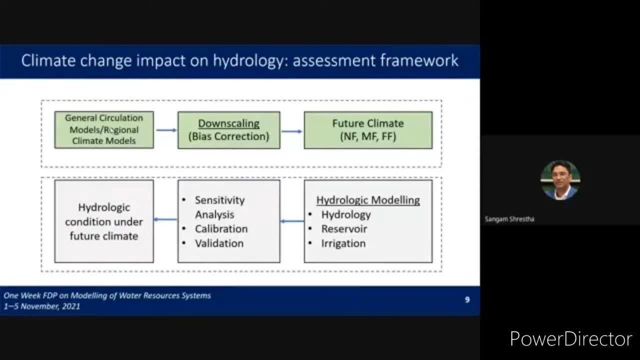 So we can use these to understand how the local level climate data is going to affect the local level climate data. So, for example, the studies are mainly conducted in the local level Right. So, for example, watershed level or, for example, basin level. 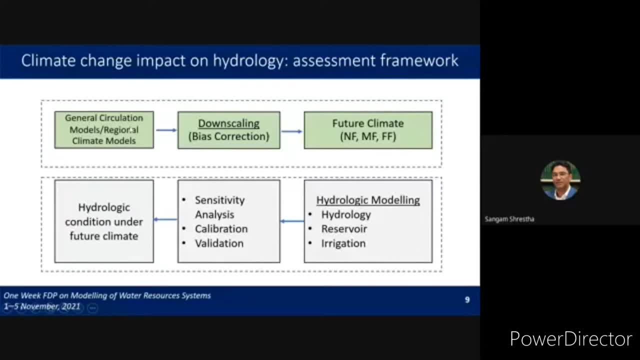 So these climate data should be translated into the you know local level And we can use the process called downscaling or bias correction, And there are several techniques of the downscaling and bias correction. So, depending on the you know the, the you know climate data, 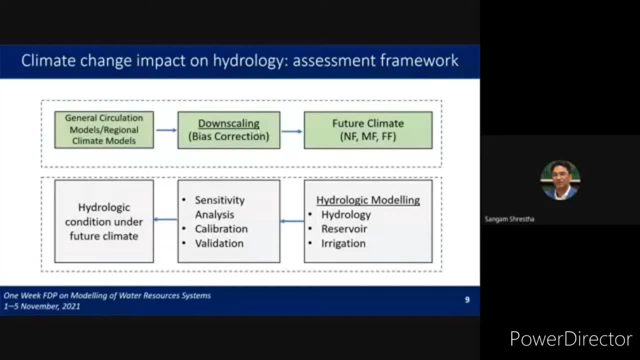 the availability of the data, depending on the skills of the researcher. we can use any of the methods to downscale the climate data of the general circulation model or regional climate models to the local level. So once we have the future climate data, the second step consists of using this future. 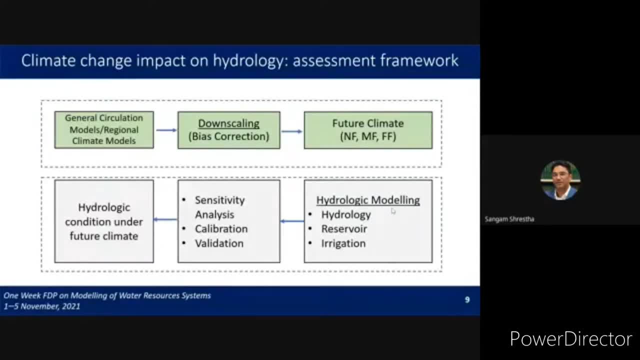 climate data to the hydrological models to predict what could be the hydrologic conditions under the future climatic conditions. So there are several hydrological models or hydrological tools available for the hydrological modeling right. But before we use the hydrological models, 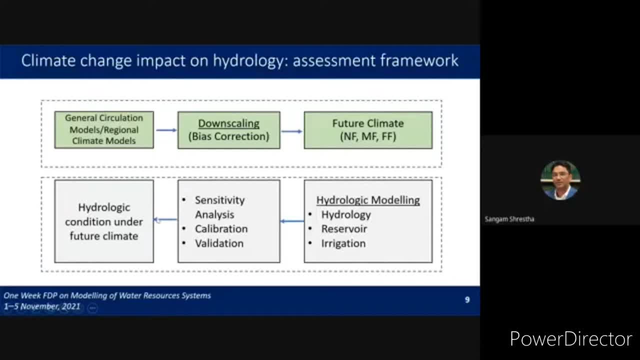 Okay, We have to, you know, calibrate or validate these hydrological models to see whether they are really capturing the hydrological processes of the given watershed or the given river basin, to simulate the climate change impact on the hydrology and water resources. 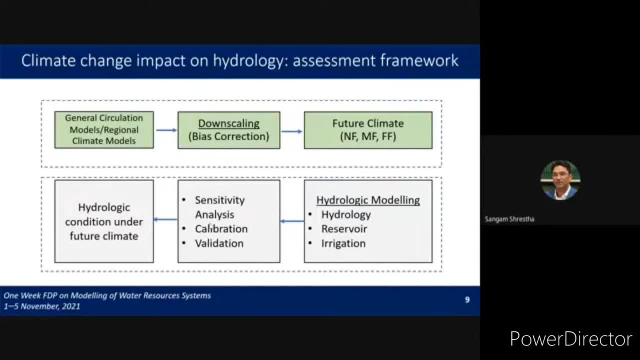 So this is the general, you know modeling framework to assess the climate change impact on the hydrology and water resources. So this is the general, you know modeling framework to assess the climate change impact on the hydrology. So, to summarize, assessment of climate change impact on the hydrology is a two-step process. 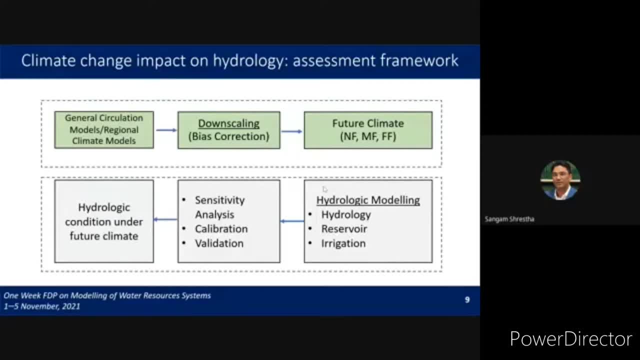 In the first step, we generate or we construct the future climate scenario of that location and we use that future climate data and feed into the hydrological models and we generate the- you know hydrological models, Since theTF低 neuroassessment program is itself. you know water resources systems. 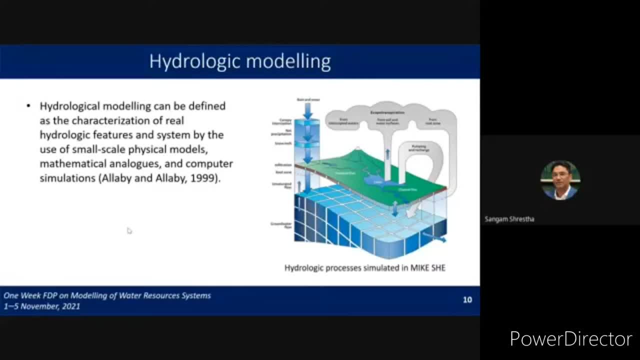 I think there will be several lectures on the hydrological models or hydrological I. I just want to define the meaning of the hydrological modeling here. even more important. and then NASA's software can program services, Because we have Welliterate storage systems. and another overall context is: what do we do? 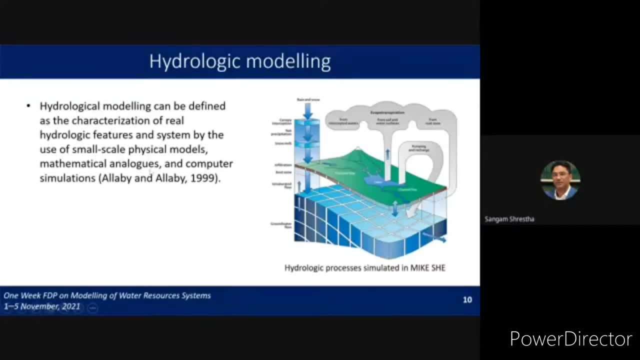 engineering does all these things, that kind of. So the hydrological modeling is defined as characterization of the real hydrological features or the system by the use of small scale physical models, mathematical language and computer simulation. So the hydrological modeling is a creation of the, you know, artificial representation of the real world system. Here the real world system is the hydrological processes of the watershed or hydrological processes of the river basin. 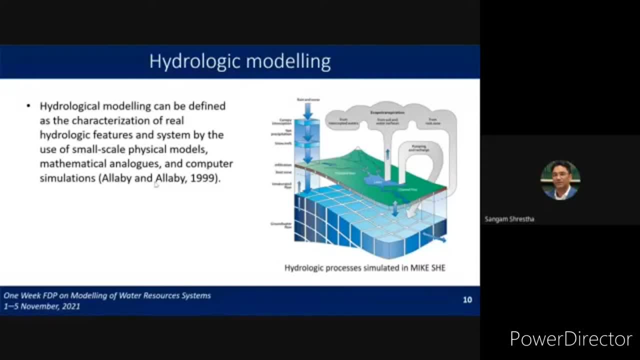 And that artificial representation of the hydrological processes is represented by several numerical equations And once we provide the input into those- you know the artificial representation of the hydrological processes- we can get also output from that- the artificial- you know the hydrological systems in terms of the several hydrological variables such as runoff groundwater flow and 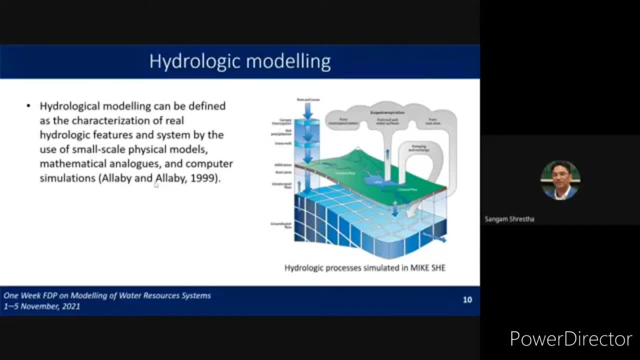 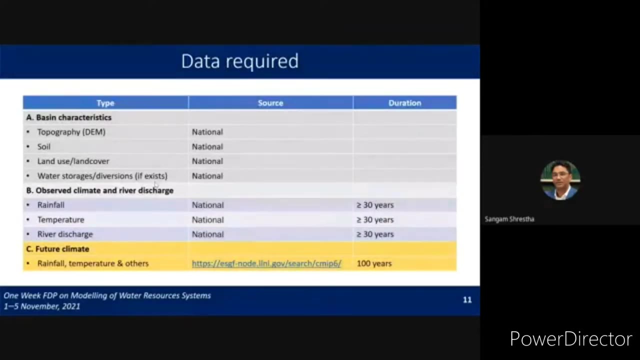 and so on. So we we use several kinds of the hydrological models to to simulate the hydrological processes under the change, the climatic conditions. There are different kinds of the data required for the hydrological modeling or climate change impact assessment on the hydrology and water resources. 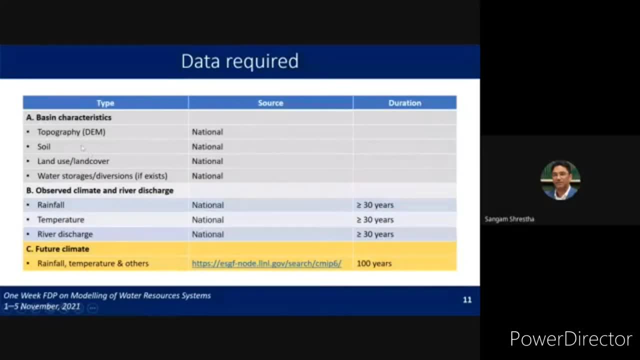 Some of the data I have outlined here. We need the basin characteristics for the watershed, characteristics Such as topography of that location, soil type of that location, land use and land cover of that location And, if there exists, the water stories or what water diversion We also need on those kind of the data. and these data are very essential because 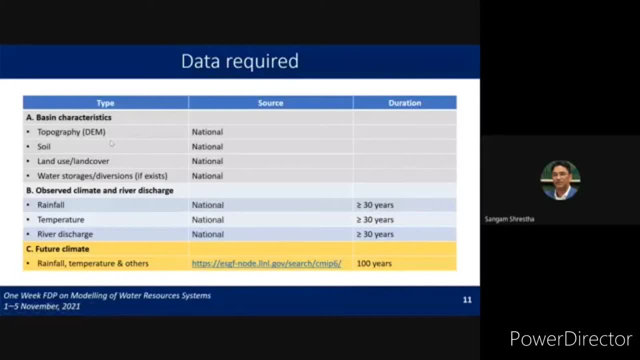 It affects the, you know the hydrological processes of the given water state or given basic. We also need the observed climate and river discharge and these includes the rainfall temperature river discharge. So in the climate change impact assessment studies we usually require the Longer term data of these. 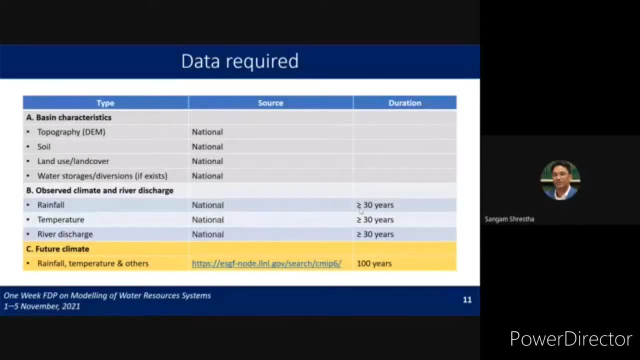 These climate and and river discharge. The minimum data requirement is of at least 30 years- And we also need the future climate data. and then these future climate data we generally, you know, obtained from the general circulation model or the regional climate models, and these are the very reliable source of the future climate data. 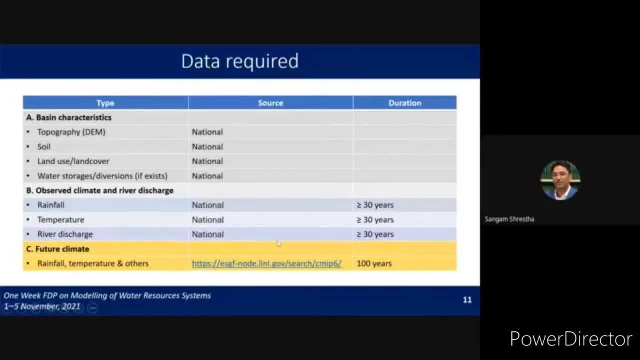 And there are several, you know, modeling centers or there are several climate change research centers and they usually provide these data free of cost. So these data can be freely, you know, downloaded from those kind of centers or the research centers website and one of the link I have given here where we can find the climate data. 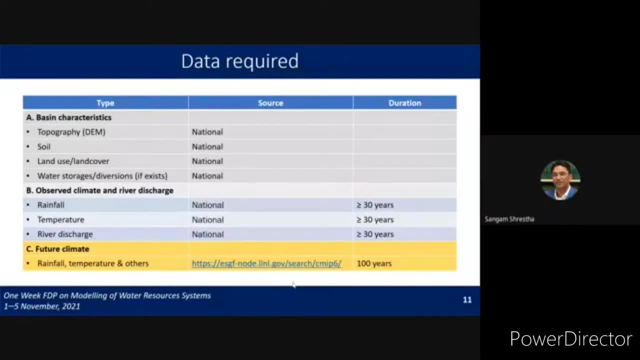 Of at least 100 years from several general circulation models or our regional climate models, And it's always, you know good, to use the national data set, but Many of the times these data's are not available from the respective government agencies, Right. So, 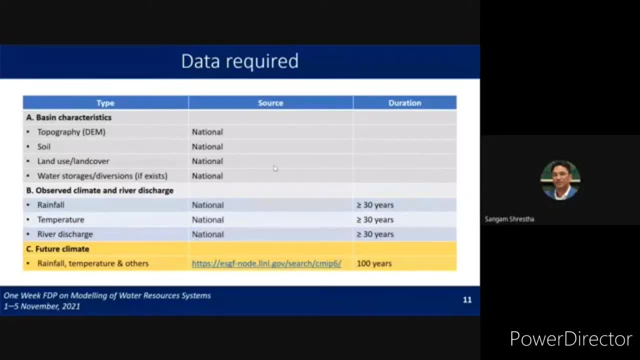 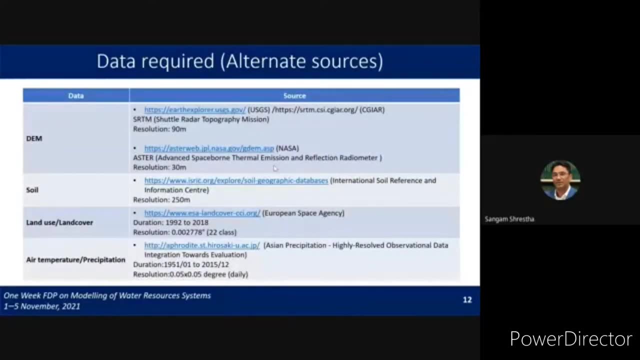 In our, in our, you know, reason: there is always Scarcity of data. So there are some alternate sources of the data, and these alternate sources of the data I have also outlined here, for example for the digital elevation model, which is the topography of the given location, can be downloaded from the 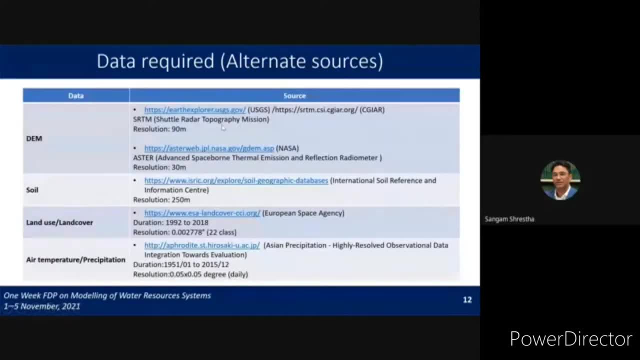 Website of the USGS, or, you know, The NASA. So they have different resolution of the DEM available. for example, from the USGS, the digital elevation model of 90 meter resolution is available. from NASA, the digital elevation model of 30 meter resolution is available. okay, 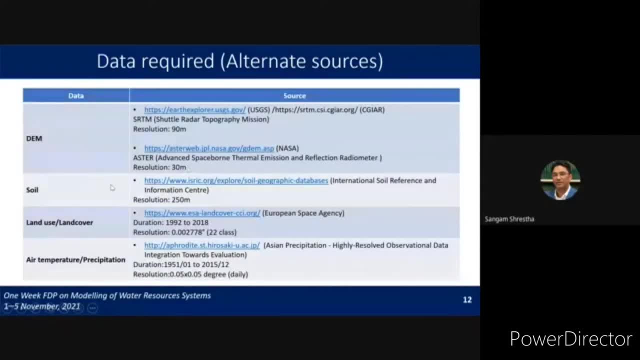 The soil data. There are, you know, Different Center or different website available for the soil data. So there are a number of different websites available for the soil data. Also recently, very high resolution soil data is available from this International soil reference and information center which is off 250 meter resolution. but there are other website where you can also download the soil data, for example food and agriculture organization of the United Nations. But those are course resolution of the soil data. 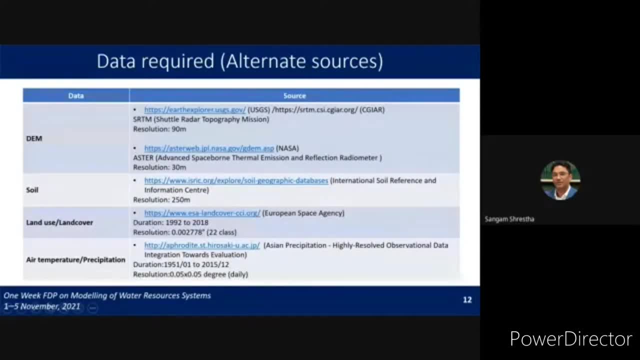 Similarly land use and land cover data. they are also available from several uh. you know the, the website, and also from the projects. for example, the annual land use and land cover data is available from european space agency, esa and the. the duration of the land use and land cover data is from 1990 to 2018. so 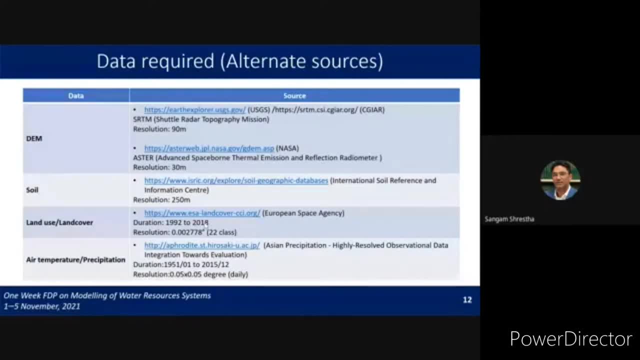 this is annual land use and land cover data available. similarly, temperature and precipitation data are also publicly available. for example, this is one of the you know project called aphrodite, where the the temperature and precipitation data from 1951 to 2015 is also available and these data 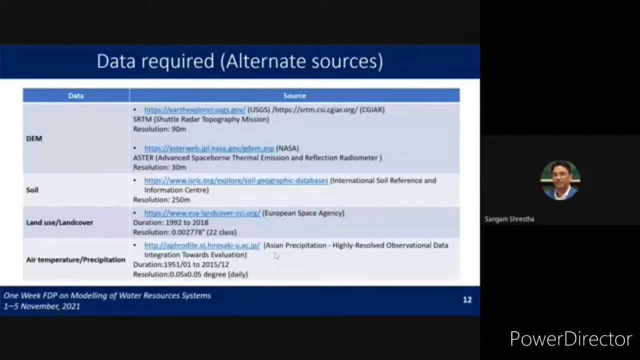 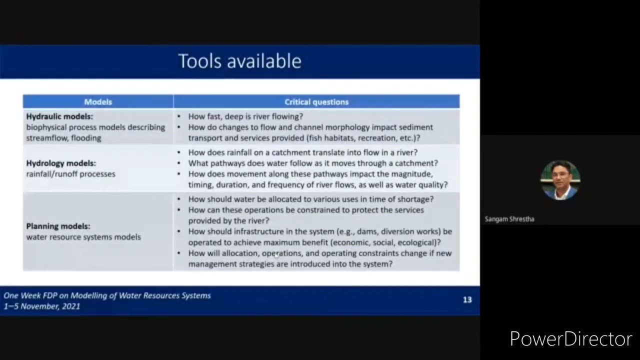 they are also available from the platypsis model, but thus this is a much better alternative for the uh resolution. so these are some of the list of the alternate sources of the data if we do not have the data from the respective government agencies, either hydraulic models or hydrology models or planning models. so, depending 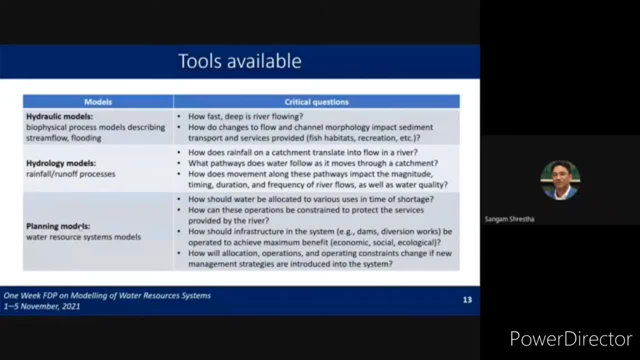 on the the purpose of the climate change impact assessment. we can use either of these kind of models. we can use either hydraulic models if we are interested to assess the impact of climate change and floods, right. but if we are interested in climate change impact assessment on the water balance, or hydrological or 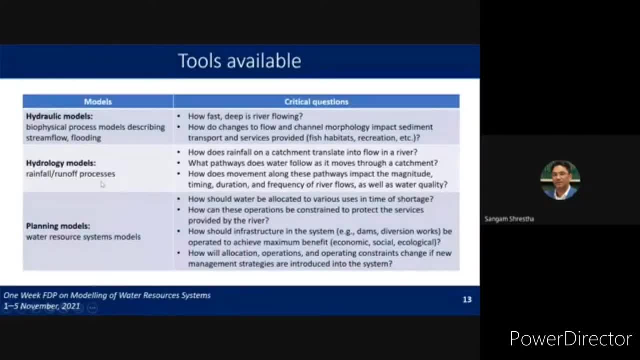 rainfall, runoff processes. then we can use the hydrological models. similarly, there are models called- you know- water resources systems model and these water resources systems models can be used to see how we can allocate the water resources for different beneficial sectors or how do we optimize the- you know- water resources allocation to different. 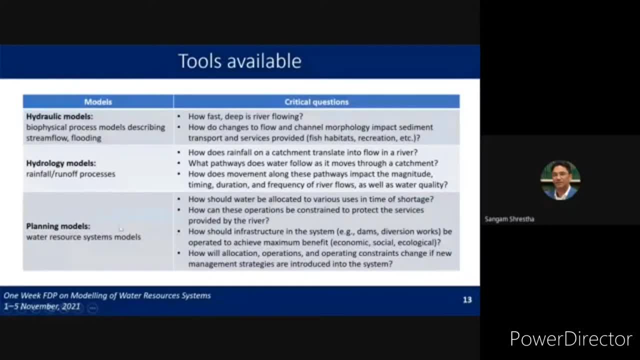 beneficial sectors, so in that case, we can use these water resources systems models. okay, so there are several- you know- models available to conduct the climate change impact assessment on the hydrology and water resources, and the selection of the models depends on the purpose of the climate change impact. 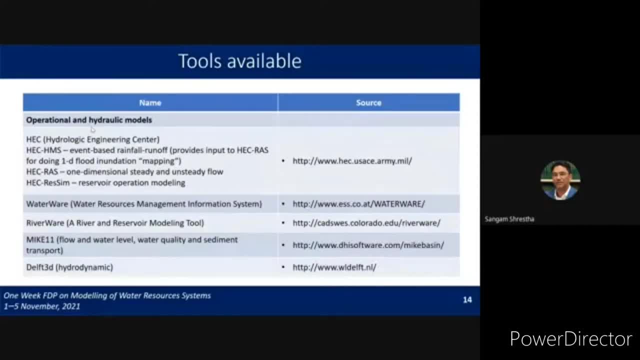 assessment. these are some of the names of these different. you know types of the models. for example, there are the operational and hydraulic models, such as the HEC series. hydrologic engineering center developed these: HEC-HMS, HEC-RAS and HEC-RASim. 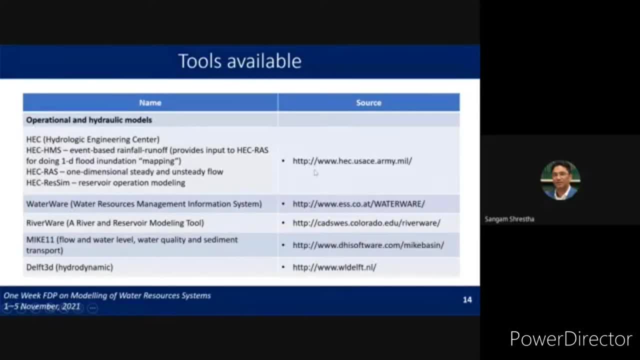 so I have given you here what is the web link to download those model. similarly, there are models called water where river, where Mike 11 and Delph 3d. so some of the models are freely available. we don't need to pay, but some of the models we 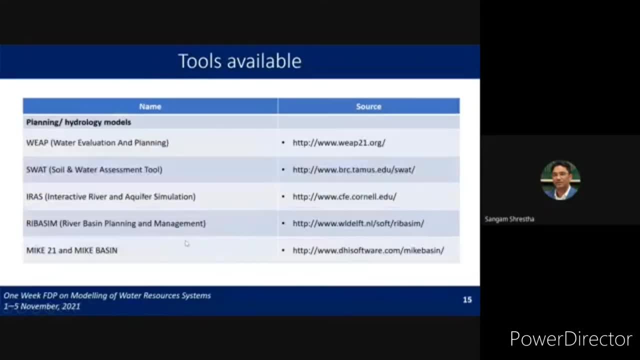 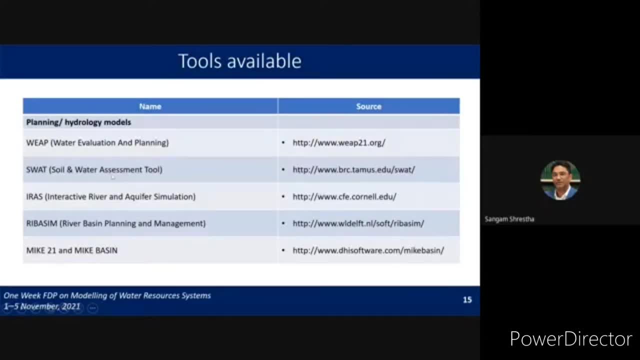 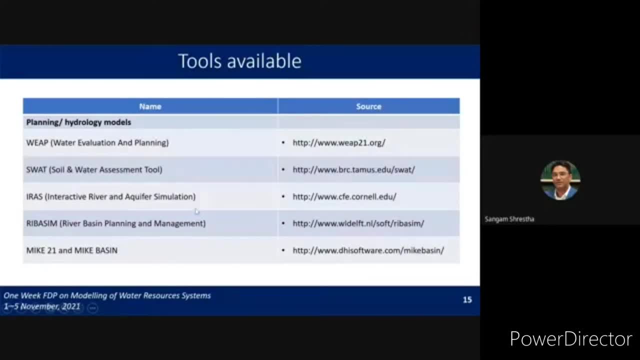 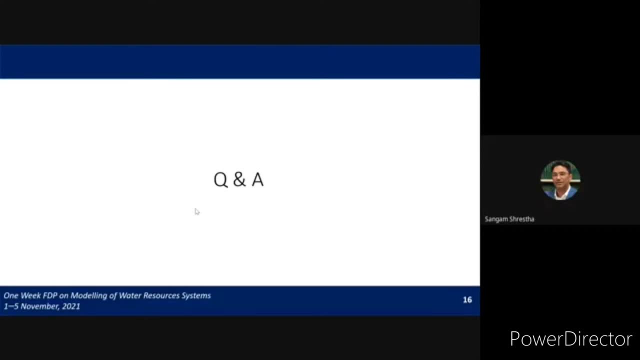 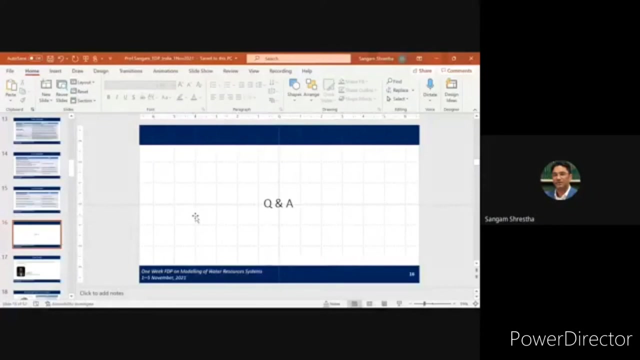 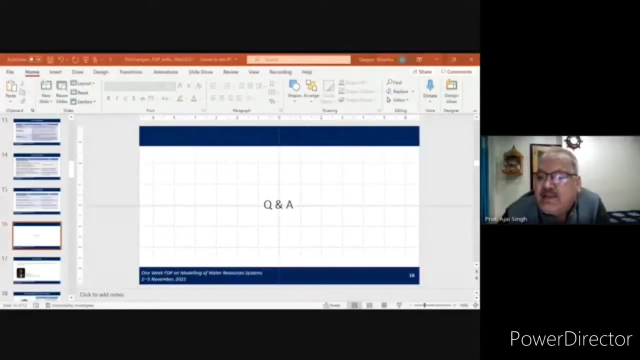 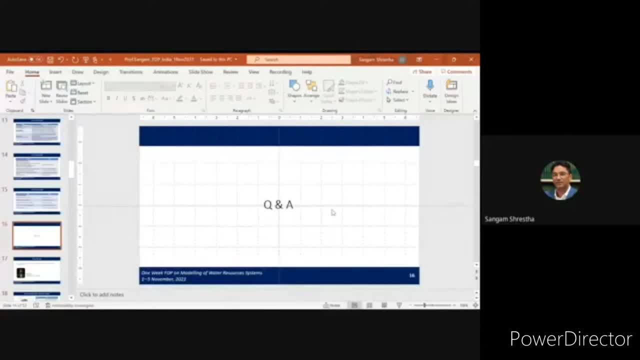 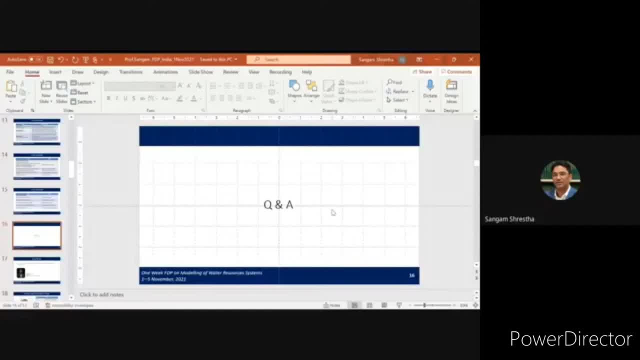 historical observed climate data, and if the climate model simulated historical climate data and the historical observed data is quite similar, then we believe that the model which simulate the historical climate data accurately will also simulate the future climate data accurately. so that's the you know assumptions we have to make. okay, so there are no. yeah, there are no other. 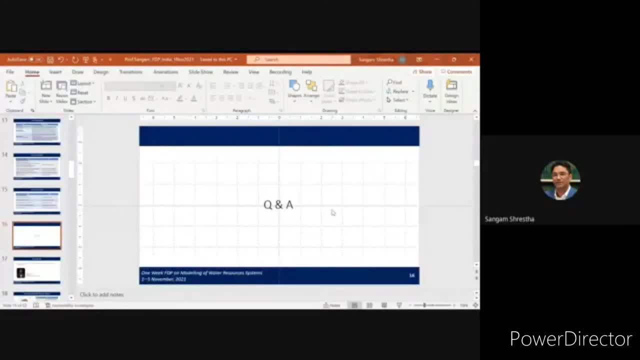 ways to validate the future climate data, because this is happening in the future time period. right, so we have, you know, many generals. we just compare the historical climate data and the historical climate data simulated by the climate models and if they have very good correlation, we assume that this models works well in the future to project the future climate. 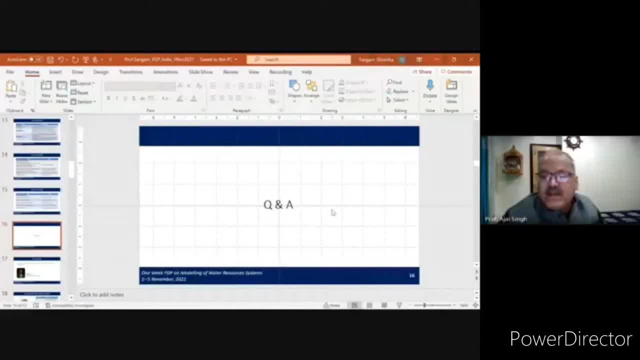 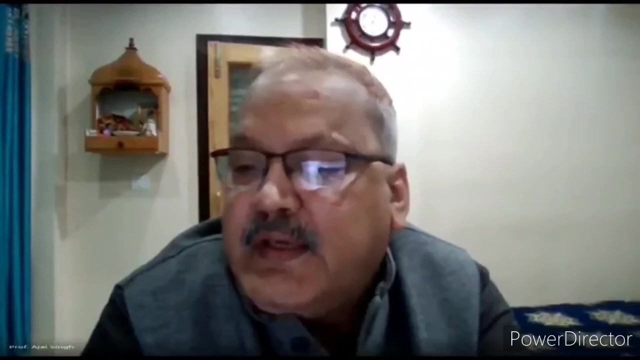 data. is that clear historical climate data need to be predicted by the climate models and then we can see how this is close to the observed value. I think that's good. so we we have two, three more question: Savitha and him and he, as he is asking what should be the minimum. 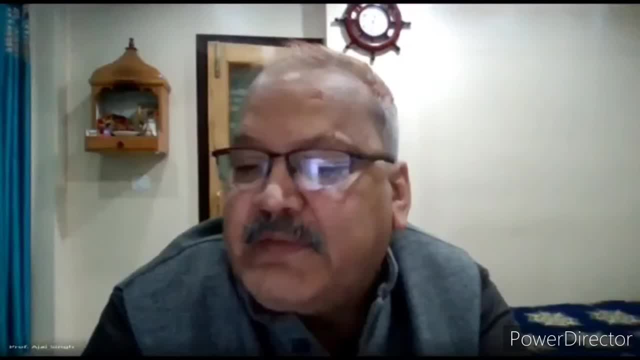 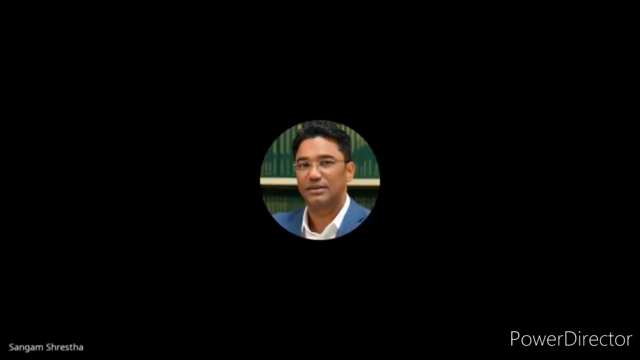 length of metallurgical data needed for climate modeling. what will be the minimum length of metallurgical data needed for climate bonding right? this is also very important question. normally we require a clearst of 30 years of climate data. okay, so the world meteorological organization. they recommend use of the 30 years, or more than 30. 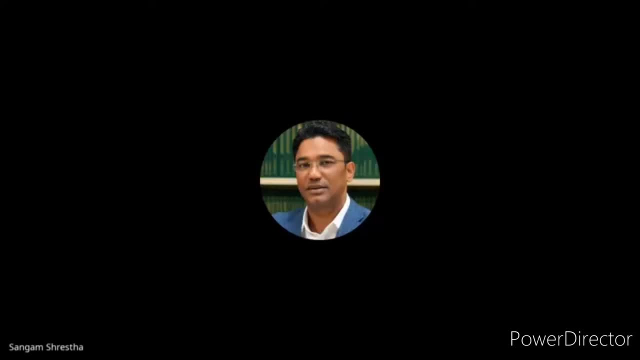 years of the meteorological data to define the climate of any given location. right, so it means that if we want to- um you know, study the climate change or climate change impact assessment studies, we need at least 30 years of the climate data. thank you so much. yes, one more question is there. 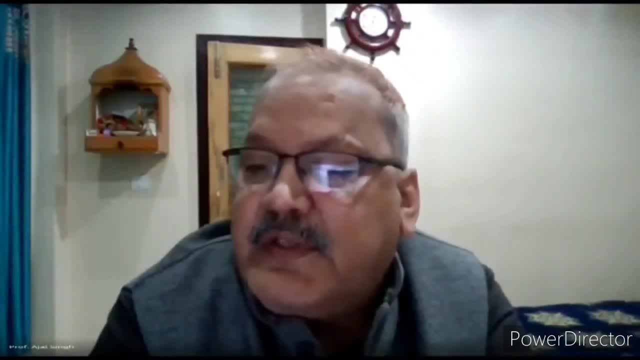 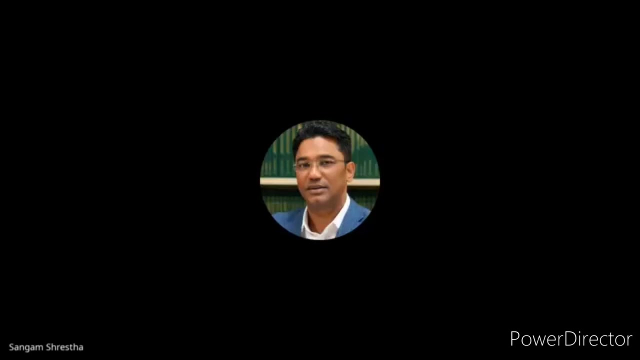 from tasif ahmed and he is asking that: what are the hydrological models used to analyze the impact of climate change on the urban areas? okay, the hydrological models used to analyze the impact of climate change on the urban areas? okay, that's very good question. also, as i mentioned that you know there are several types of the. 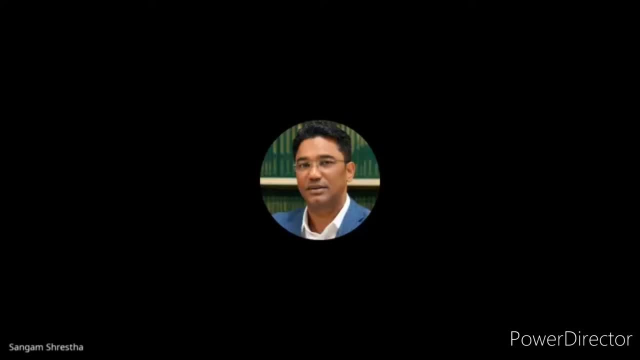 models which can simulate the hydrological processes of the water state or river basin. also the urban area, right. so we need the, the models which captures the hydrological processes in the urban area and there are several, you know, urban hydrological models which can be used to assess the impact of climate change on hydrology, on on urban, you know, hydrological processes. 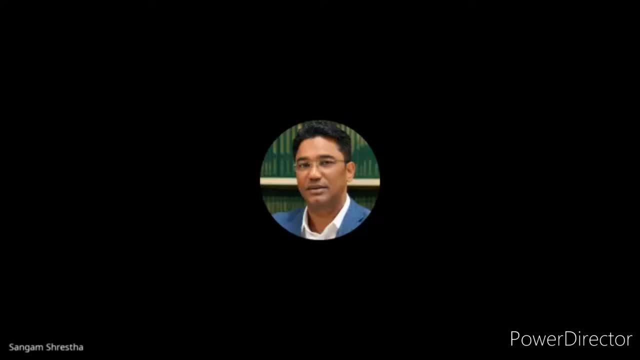 so one of the very popular models available is called pc swing. this pc swing model can be used to assess the climate change impact on the urban runoff or urban drainage. and again, there are several other- uh, you know- hydrological models available um to to predict the climate change impact on the urban hydrology. so these are basically urban. 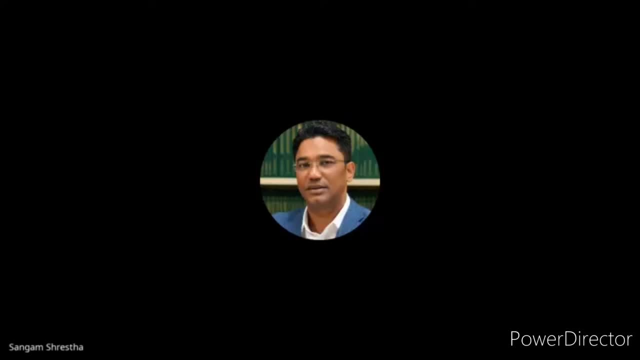 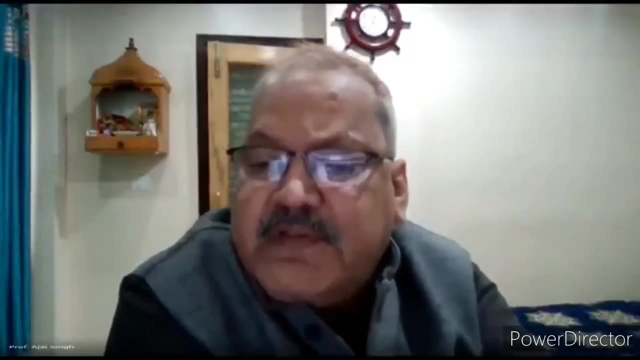 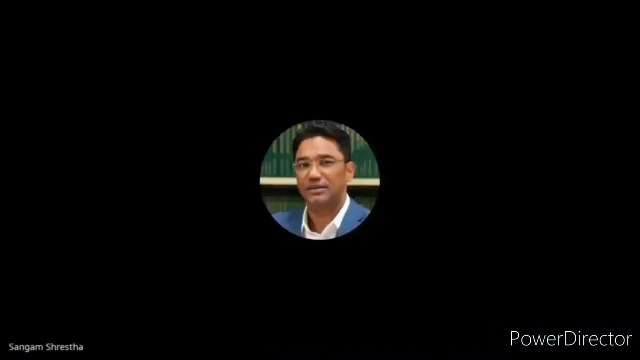 hydrological models like pc swim or you know, the the basin model. thank you, yes, this is uh same means: swma model. yeah, right, right, yeah, okay. uh, mr suman de bourbon is asking that that what may be the impact of the climate change impact on urban hydrology? 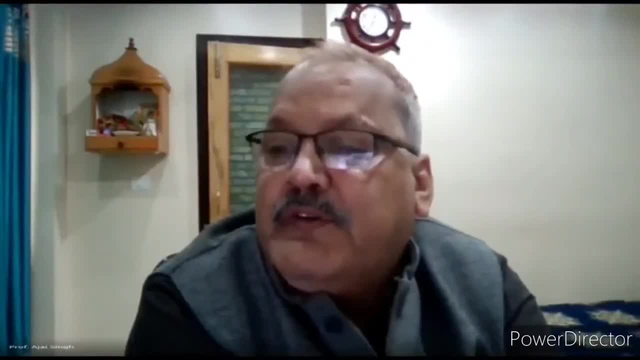 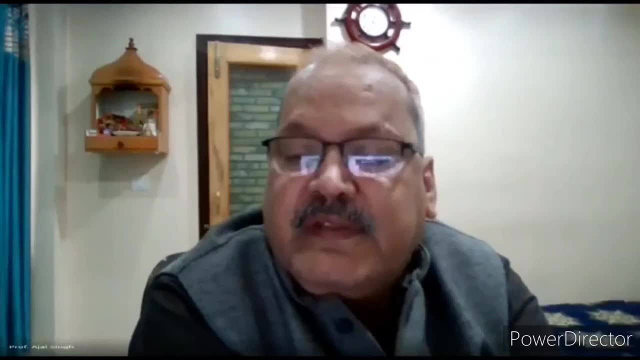 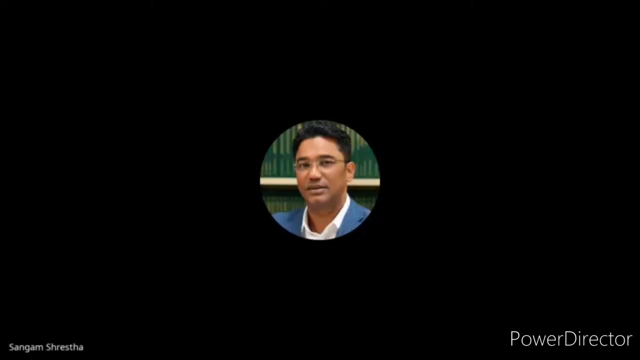 climate change on sediment load of a river basin. climate change impact on sediment load of a river basin? yeah, that's also very good question and yeah, it depends on how the climate will change in that river basin and how that will impact the you know the runoff processes in the river basin, because 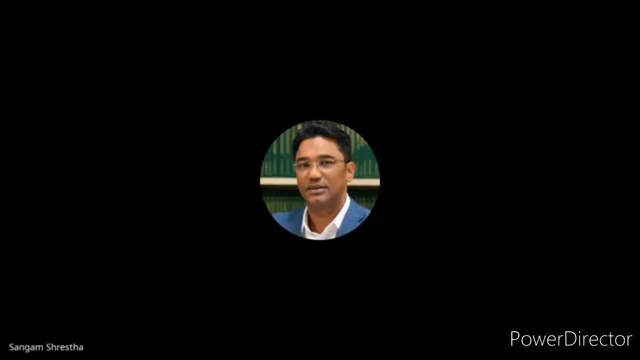 they are linked right. so, for example, if any river basin, the the rainfall is projected to be very low, then probably that will generate, you know, either no sediment or soil erosion or very less soil erosion, right? so in that case probably sediment load will be very less. but if the rainfall intensity is very 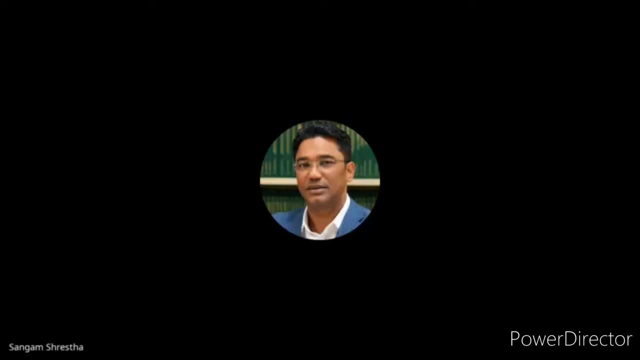 high and, depending on the land use and land coverage and the water quality, the sediment load will be very low and the the sediment load will be very low and the sediment load will be very low and the you need to. you know we really need to conduct the this climate change impact. 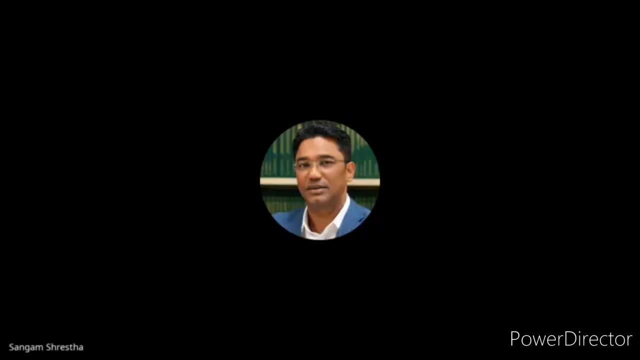 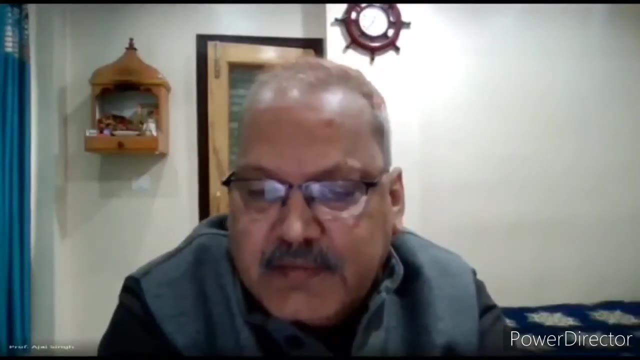 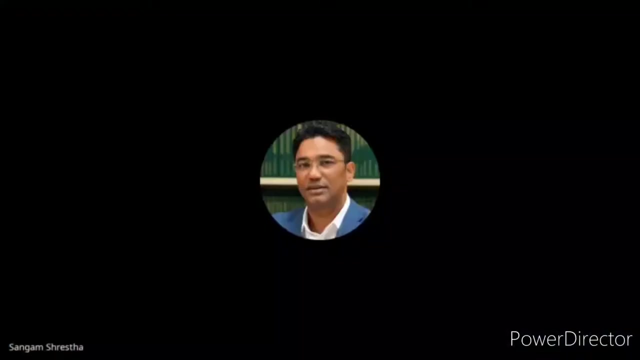 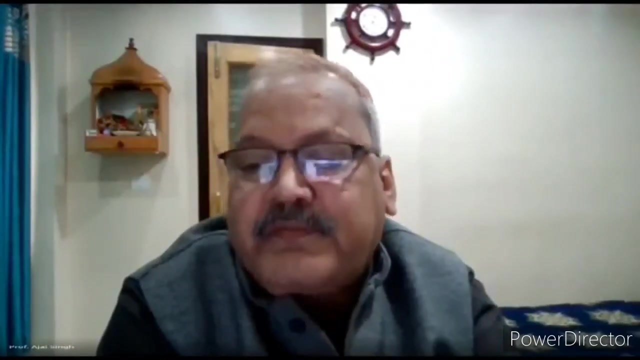 assessment on the sediment yield or sediment loads. Yeah, actually, under climate change impact, lots of accumulative rainfall can occur in a single day, So this is what the participants predicted. So more rainfall means more generation of runoff. So more generation of runoff can be understood to give more sediment, which will finally 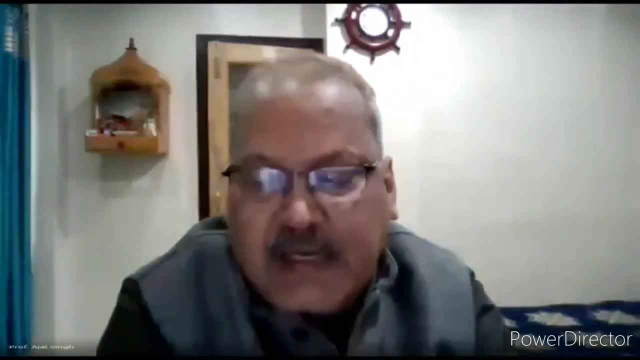 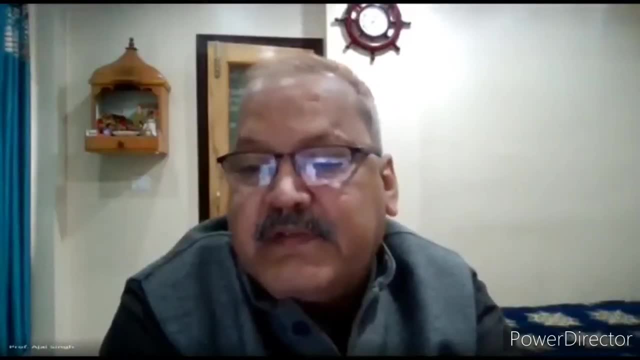 go to the river basin if you're not managing your land uses Exactly. Yeah, That's right. Yeah, Yeah. In the first class I have requested to all the participants that before you do the modeling work, you please read the hydrology very well. 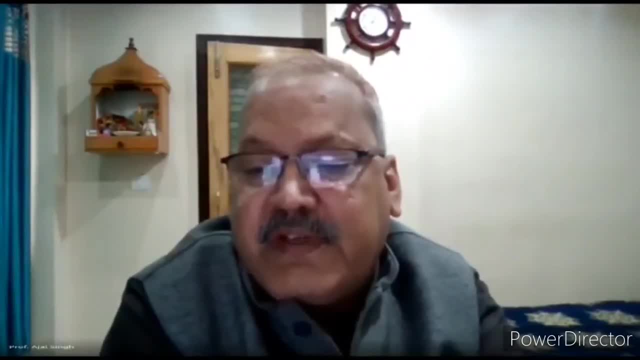 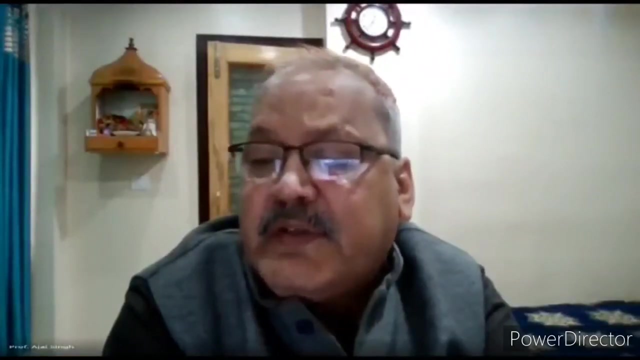 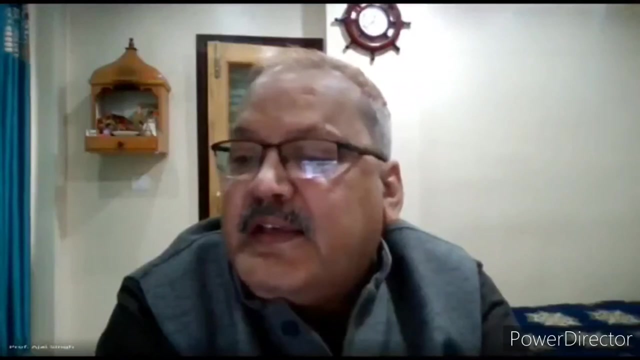 You must understand that what are the factors which are going to affect these hydrological processes, so they can understand the modeling processes. We will take one more question, then you can continue the lecture. Yes, Vanita Pandey. she is asking: can the stochastic modeling also be used for similar? 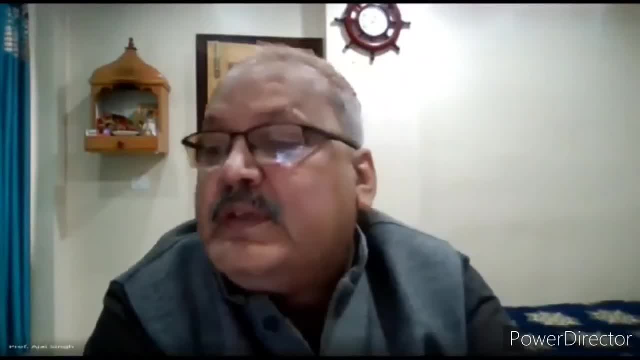 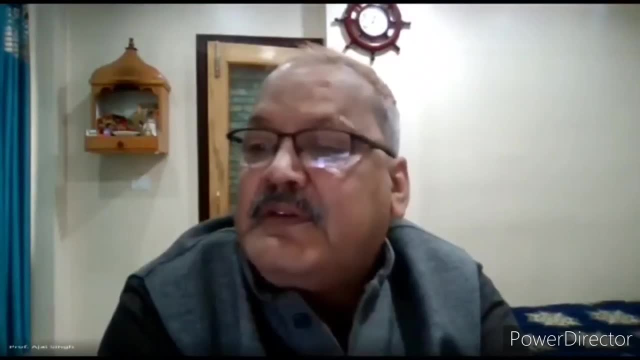 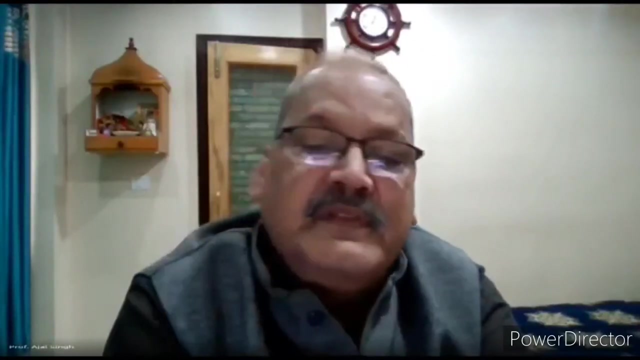 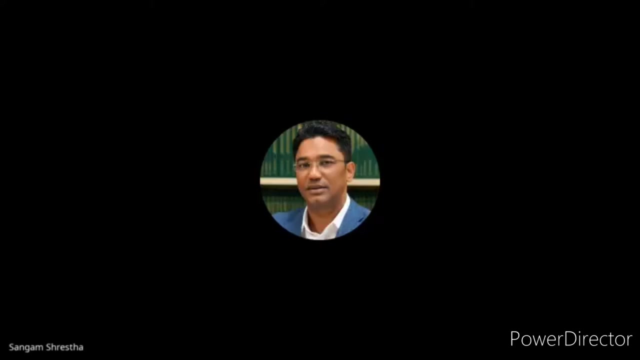 accuracy of future hydrological modeling of climate change assessment? Can we can use stochastic modeling, Right? That's also a very important question, Professor Ajay. So there are several types of the models we can use for the climate change impact assessment on hydrology. you know water resources, right? 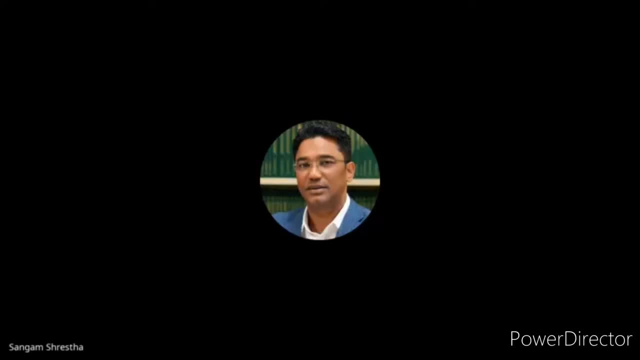 So yeah, I cannot say you know, definitely stochastic models are having similar accuracy, similar performance with the other kind of- you know deterministic or you know other kind of models. but these models can also be used. But again we have to compare the performance of these models. but definitely stochastic. 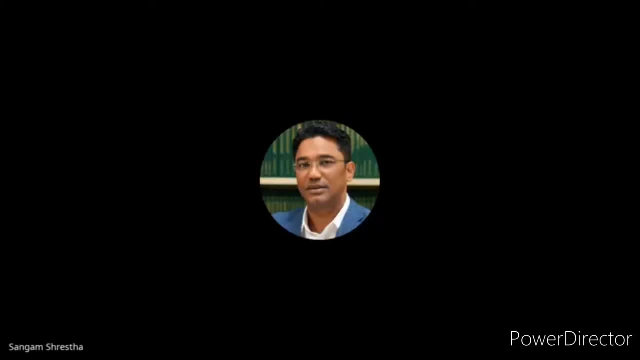 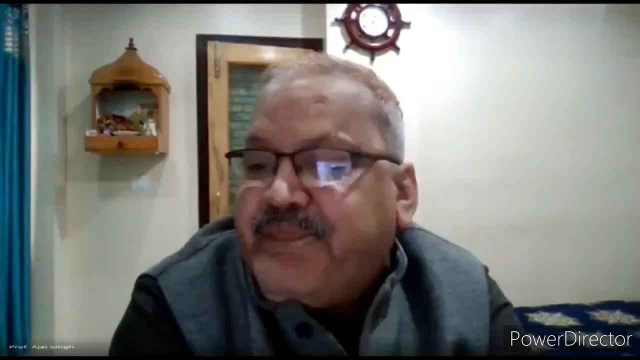 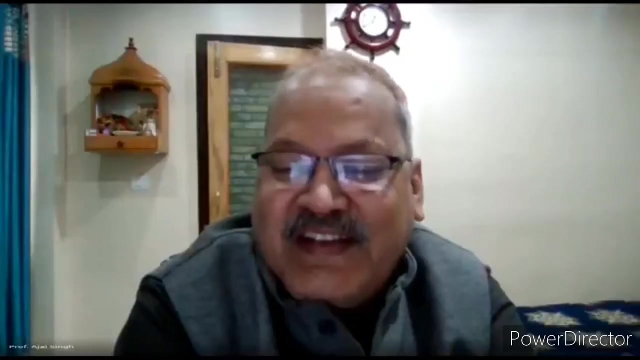 models can also be used to assess the impact of the climate change on the hydrology. Yeah, Yeah, So Okay, We'll take the remaining question later. Yeah, I think there are. Please continue. Yeah, There are several very important questions I saw in the chat box. 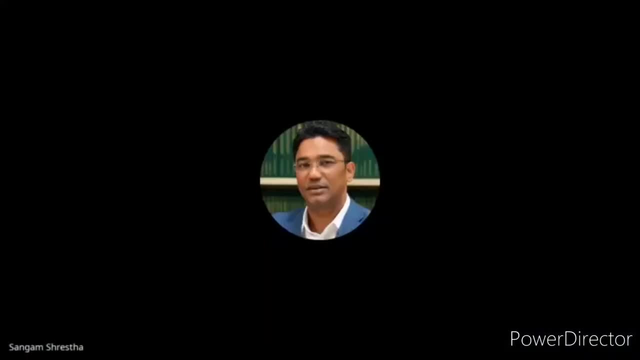 And Now you can respond. You can respond. So we we have the question and answer session. also I plan to keep it. you know, after every the major contents I covered, But anyway, I think there is one question by Suman Dev Burman I see presently in different. 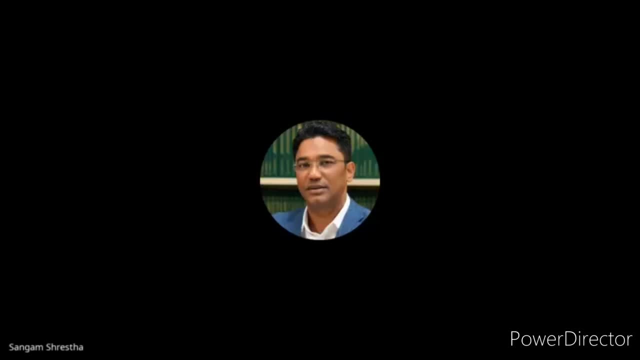 river basins, several dams, barrage constructed, So how to assess climate change impact on river designs, And I think this is very, very important question. So yeah, the hydrological processes are impacted by not only the climate change, but also the 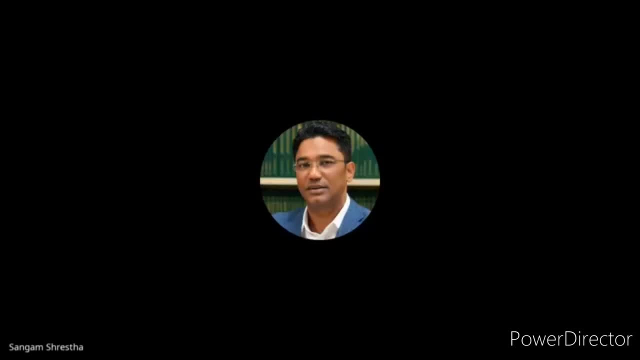 anthropogenic factors right, For example, construction of these barrage reservoirs. you know water diversion, land use and land cover chains. We convert the forest land use to agricultural land use, forest land use to residential land use And these will have all impact on the hydrological processes. 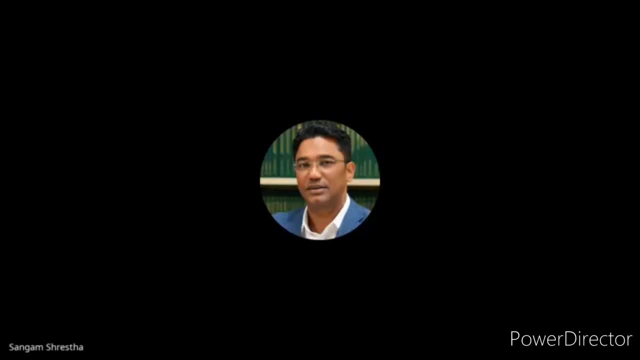 So in this case, we have to assess the combined impact of all these factors on the hydrologian water resources. It's not only the climate change that impacts the hydrologian water resources, but it is also other factors. So we can do several- you know- simulations or scenario analysis. 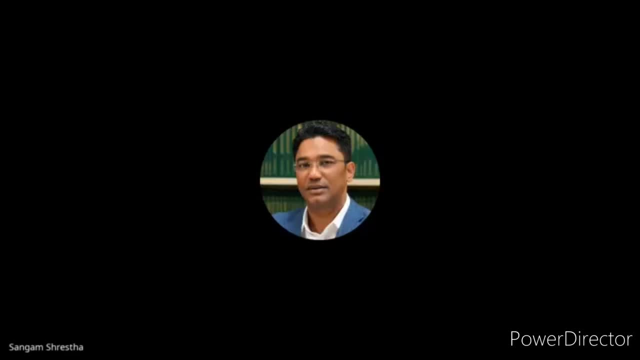 For example, if there is only change in the climate in that basin, what will happen to the hydrology? okay, And if there is change in the climate, maybe there are some other changes also, right? So the construction of the barrage, construction of the reservoir, land use change from the 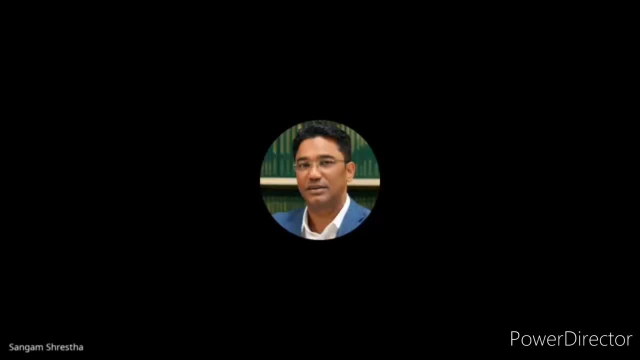 forest to the river. So we need to assess the individual as well as the combined impact of those changes on the hydrology. Okay, So I still see there are many questions, So I will, you know, describe some of the case studies and then we can come back up. 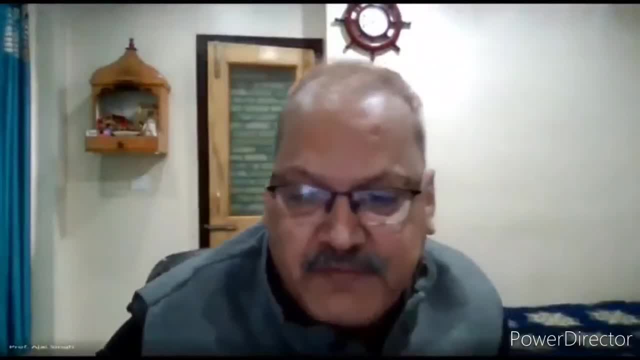 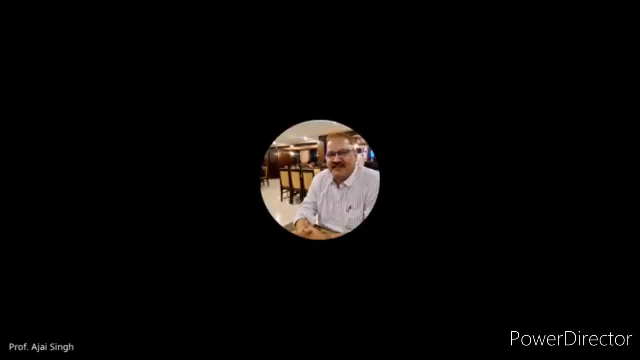 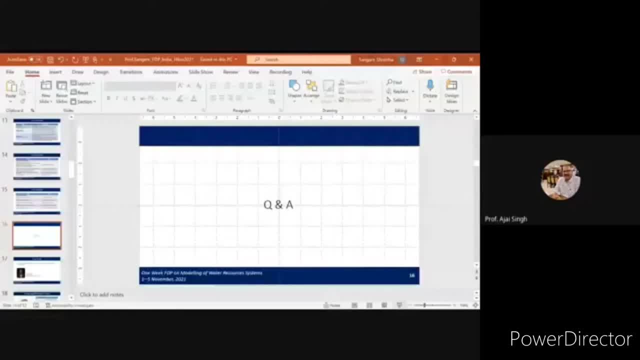 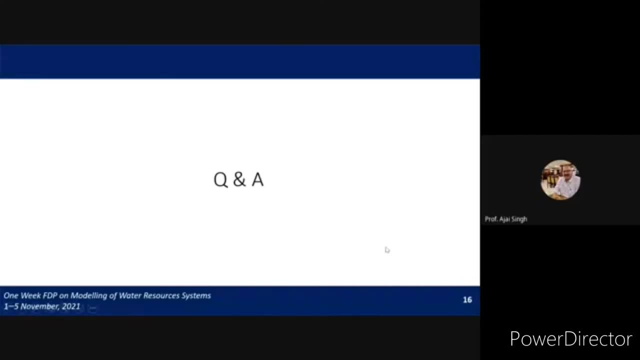 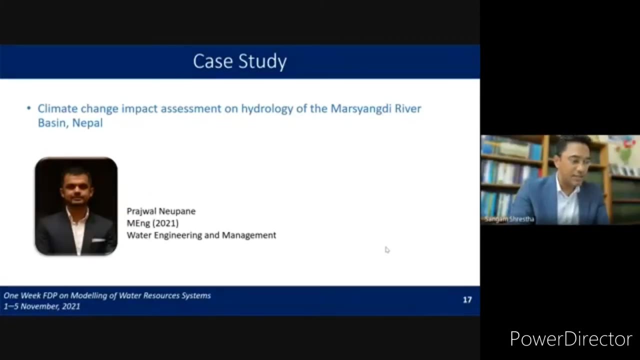 Okay, So I will explain one of the case studies. one of my students had, just you know, completed his master's thesis, so his study was related to climate change impact assessment on hydrology of marsh and the river basin in nepal. yeah, i have taken this case study to present to all of you. 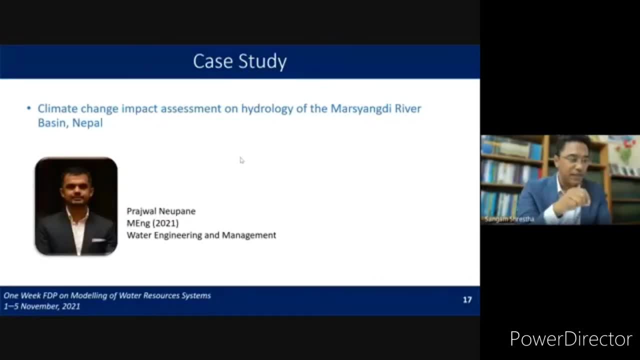 for for a few reasons. one is- this is very new study conducted by my student just two months ago and he used a new climate scenario called shared socio-economic pathway. and also this river basin is very important river basin in nepal because it has, you know, a lot of existing hydropower projects. 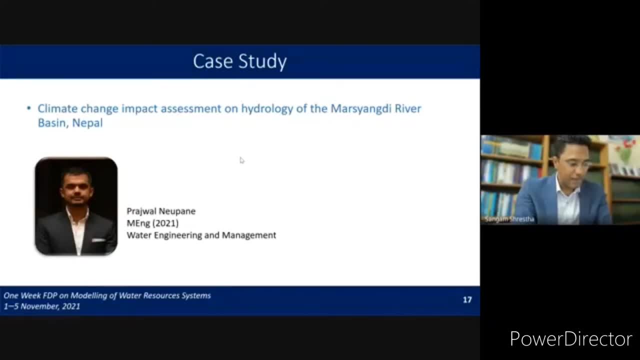 and also there are a few, you know- hydropower projects under planning. and the third reason is i have been to this river basin many times, so i'm very familiar with the river network. you know the, the land use and land cover conditions, and also the, the hydropower projects located inside this patient. so this is the reason why i have 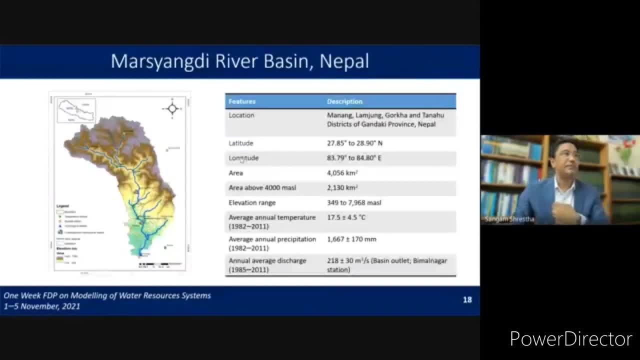 you know, presented this case study here. okay, let me briefly explain about this river basin called marsh and the river basin in nepal, and it's very important to understand the the characteristics of the basin before we proceed these kind of modeling studies. so this marsh and the river basin in nepal is located in the mid western part of the nepal. 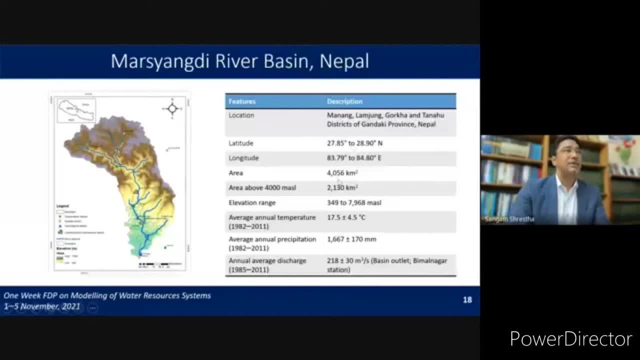 and it has a catchment area of about 4 000 square kilometers and very important is that almost 2 000 square kilometer of the area lies above the 4 000 meter above mean sea level. it means that the the basin has a lot of, you know, snow and snow cover area and these snow and snow cover 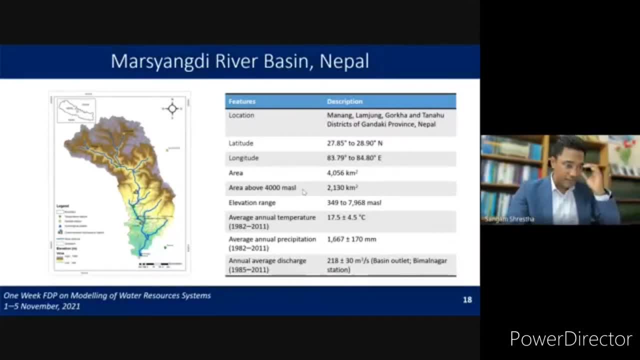 are very important source of the water for this marsh and the river basin, so the elevation ranges from 349 to almost 8000 meters above mint sea level. the average annual temperature and and rainfall is given here, So the average annual rainfall is almost 1,700 millimeter. 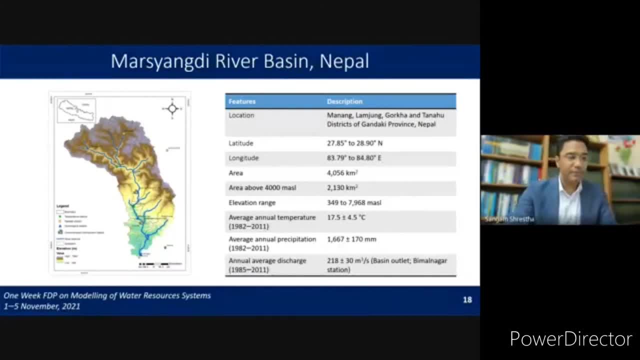 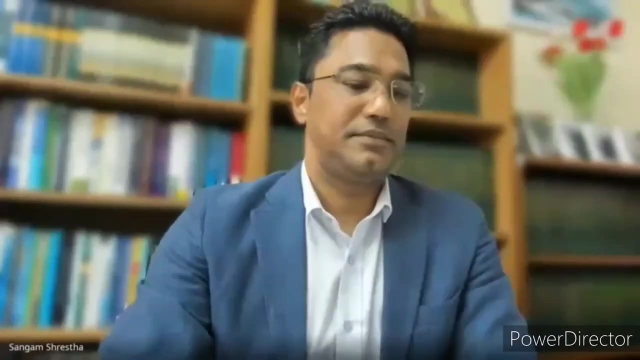 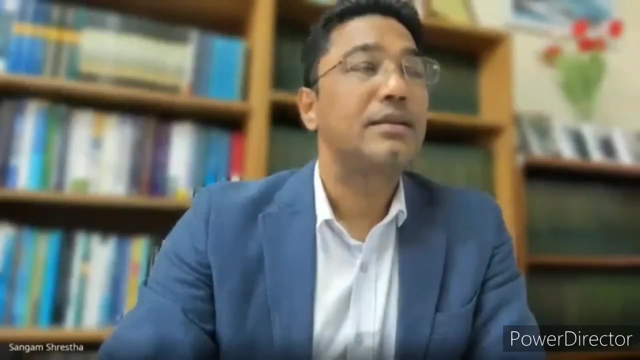 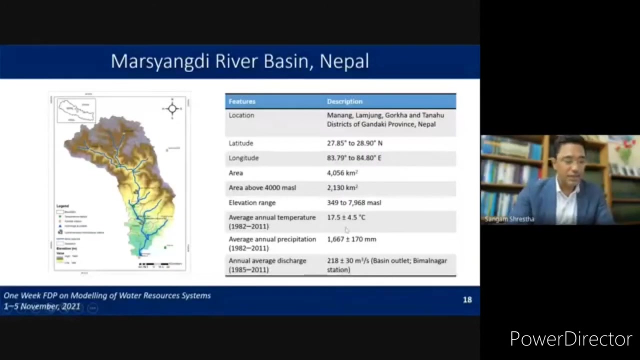 which is a pretty good amount of rainfall, And the annual discharge is about sorry, Sorry. so the annual discharge is about 218 cubic meter per second, which is at the Marsangdee River Basin Outlet, As I mentioned that this river basin 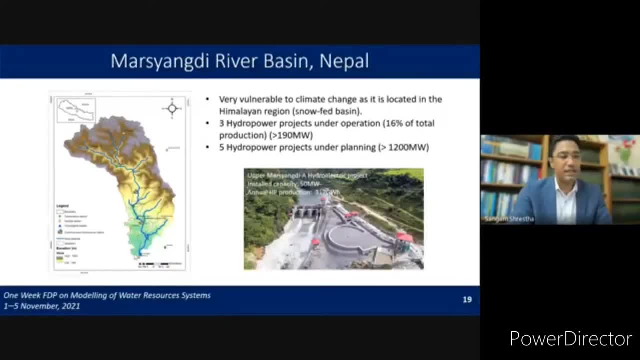 is very important in terms of the climate change vulnerability to the hydropower projects located inside this basin. Currently, there are three hydropower projects under operation and about 16% of the total production for the hydroelectricity comes from these three hydropower projects. 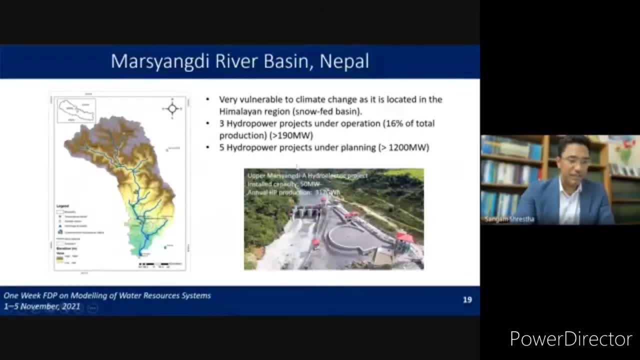 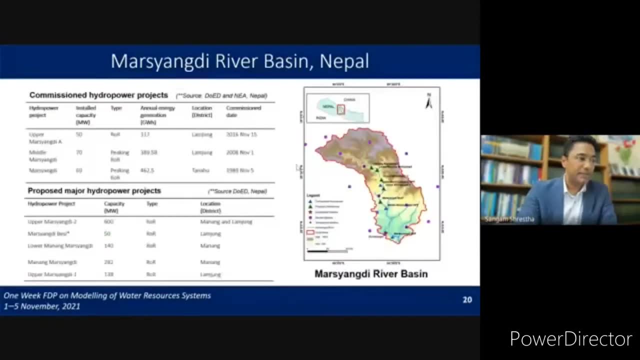 And there are five hydropower projects under planning, which is the installed capacity of more than 1,200 megawatt, And you can see the list of the existing or commissioned hydropower project and the hydropower projects under planning. 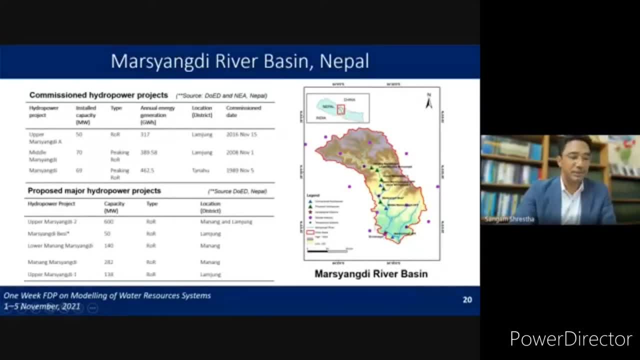 So if you look at this river basin map, you can see that these blue the triangle they are the commissioned or existing hydropower projects And this red triangle are the proposed hydropower project And the operation of the hydropower projects. 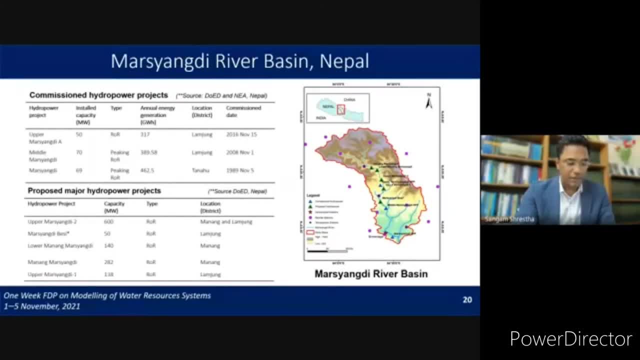 depends on the availability of the water in this main river and also the tributary river. So it's very important to assess what happens to the hydrology and water resources of this river basin to the climate change. So this is some of the photographs. 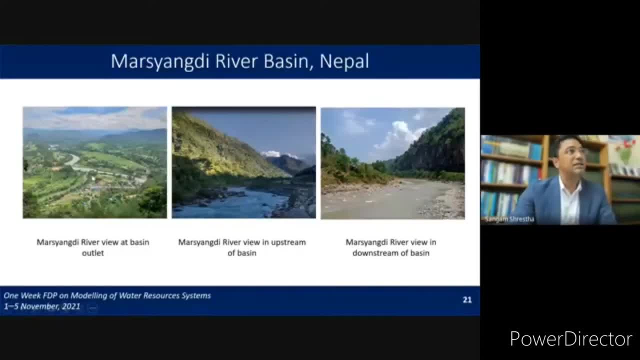 of the Marsangdee River Basin On the left-hand side. this is the Marsangdee River view at the basin outlet. The middle one is the Marsangdee River in the upstream area of the basin And the most right-hand side is the Marsangdee River. 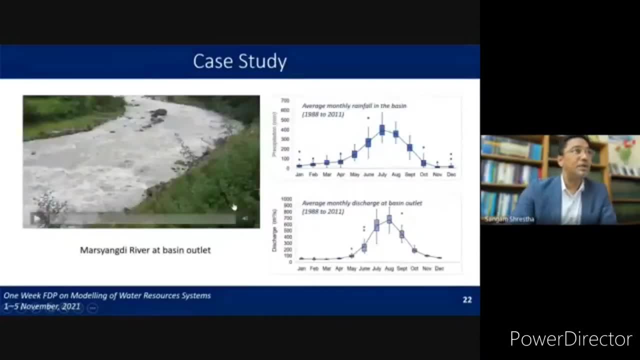 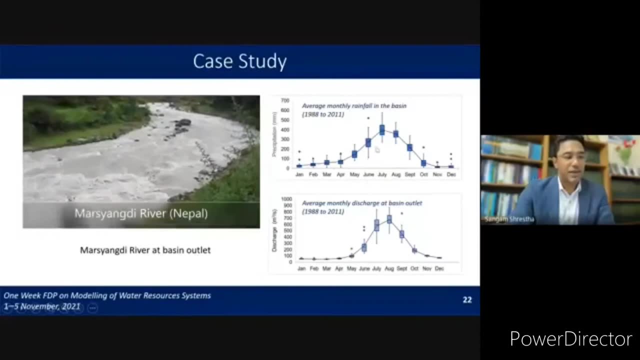 in the downstream of the basin And you can see here the river flow at the basin outlet. On the right-hand side you can see the average monthly rainfall in the basin and in Nepal the monsoon season starts from June to September. 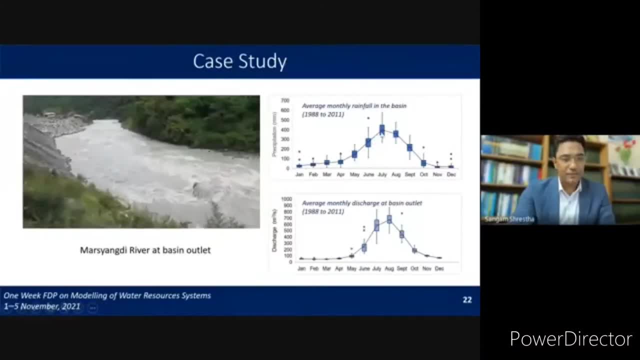 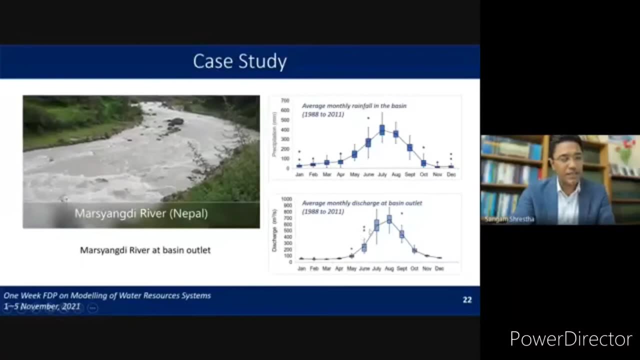 So you can see a very high amount of rainfall And in the below cargo pads of Marsangdee diagram you can see the hydrograph of the basin in terms of the average monthly discharge and, corresponding to this rainfall, the discharge is also higher in June to September. so in this video I think I imagine that this- 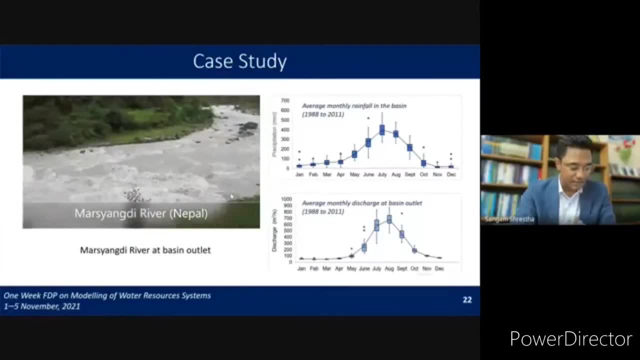 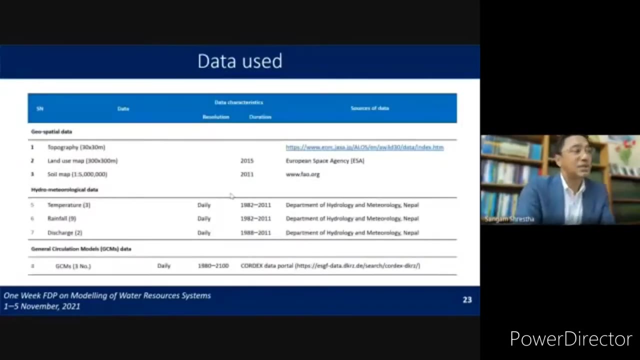 discharge is during the monsoon season. I can see quite you know big amount of flow, so it must be maybe during the July or August of the month. okay, so this table shows what kind of data we have used for this climate change impact assessment on the hydrology and water resources. so, as I mentioned that since 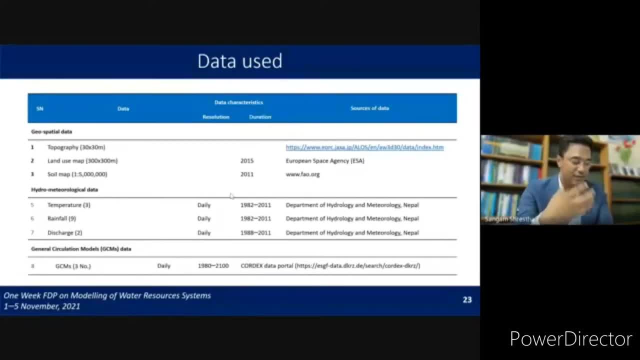 the hydrological models are, you know, artificial representation of the the hydrological processes of the river basin or water state. and these hydrological processes depends on the several, you know, characteristics of the water state, such as topography, land use, soil type and so on. that's why we have 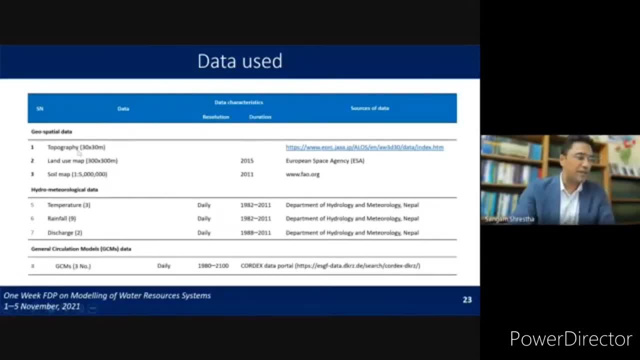 to use these kind of data, like the topography, land use map and soil map. they were obtained from these sources. the hydrometeorological data: we have used the temperature of three stations. we have used rainfall of nine stations and discharge from two stations, and these are also at the daily resolution and you can see here the duration of the. 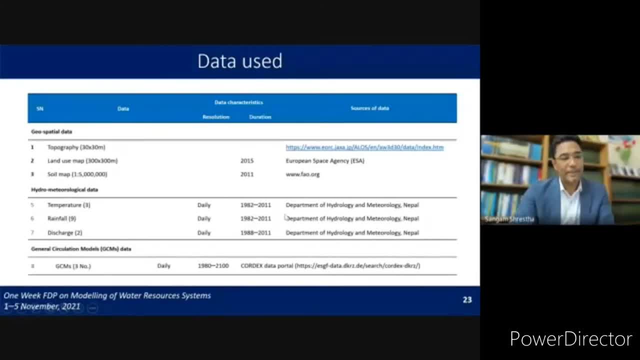 data. this is 30 years of the duration and these are data were obtained from the national source, which is from the department of the hydrology and metrology. and for the future climate data, we have used the data from three: general circulation model or global climate model, and 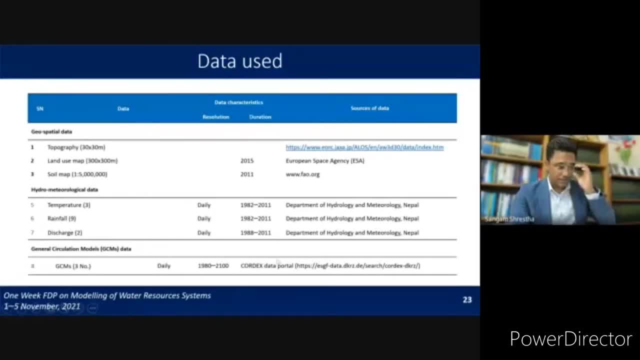 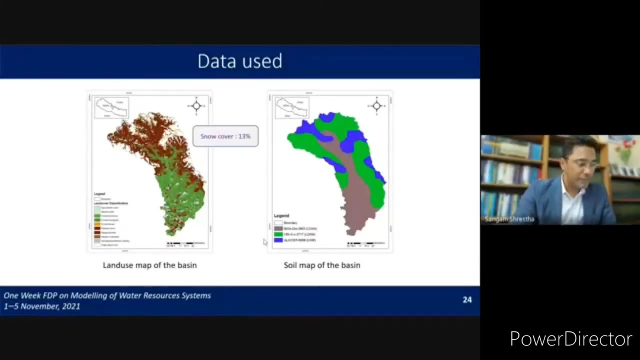 these data were obtained from this website of the cordex, you know project and these data are also at the daily resolution and this is the post pit, not the. the data are there. these two maps are related to land use and land cover map of the basin and the soil map of the basin, and on the left hand side you can see. 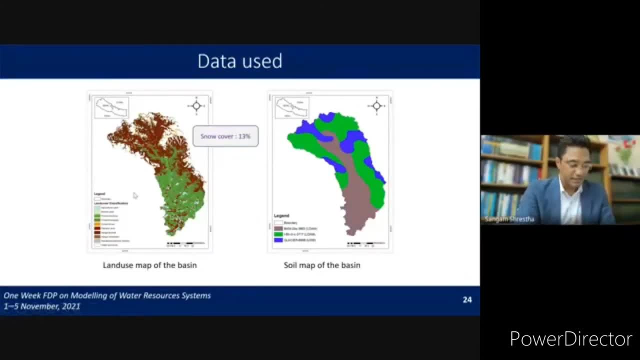 the land use and land cover map of the basin and these are the reclassified map and you can see the majority of the land use is the forest land use. There is also a snow cover area of almost 13% on the northern part of this, Marsangde. 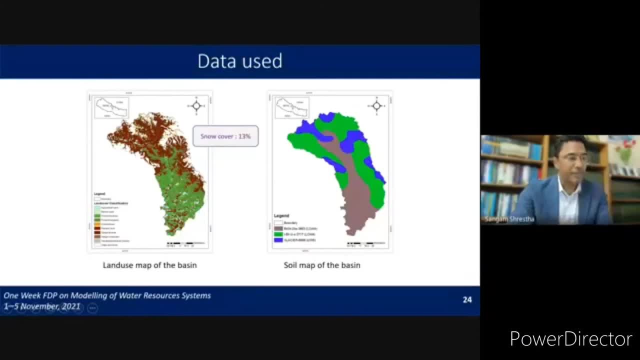 River Basin and this snow cover, or snow cover melting, also contributes to the runoff into the several tributaries and also the major river of the Marsangde River Basin On the right hand side. this is the soil map of the basin and soil map the majority of 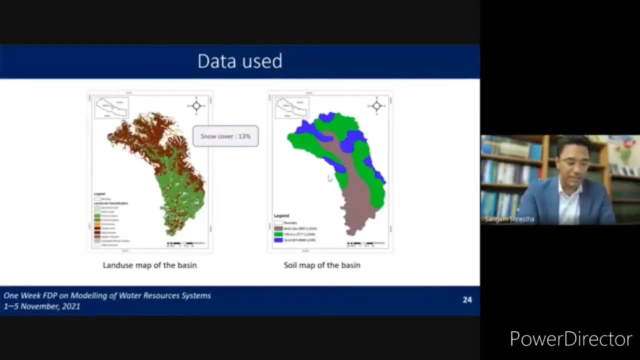 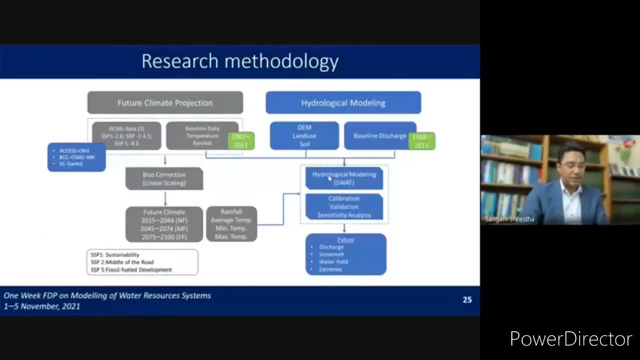 the soil is a loamy type in the basin. So this slide shows what kind of methods we have adopted to assess the climate change impact on the hydrology and, as I mentioned in the beginning, the modeling framework. this is a two-dimensional model. 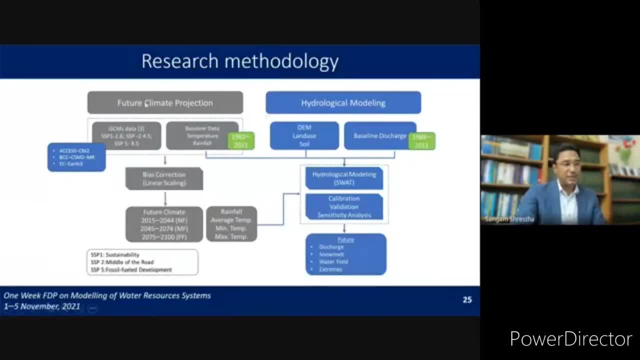 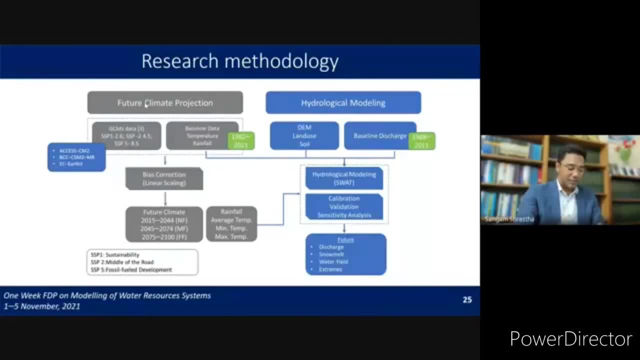 the future climate data on how the temperature will change and how the other climate related variables will change in the future, and we call it as a future climate projection. So in this particular study we have used the climate data from three general Lower agency final star regulation models. 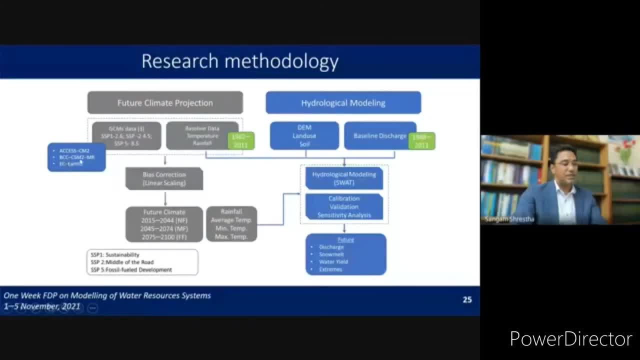 These are XSCM2, BCCCSM2MR and ECR3.. So these are the three general circulation models and we use the climate data of these three general circulation models, both historical data and the future climate data, And there are several scenarios where these GCMs has already simulated. 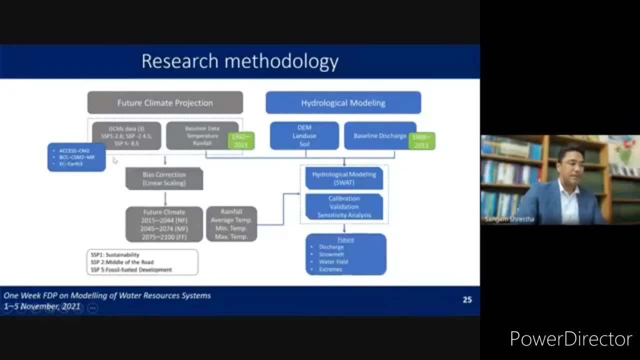 And these scenarios are from SSP1, 2.6,, SSP2, 4.5, and SSP5, 8.5.. And the name of these scenarios I mentioned here: SSP1 is sustainability scenario, SSP2 is middle-of-the-road scenario and SSP5 is fossil fuel development scenario. 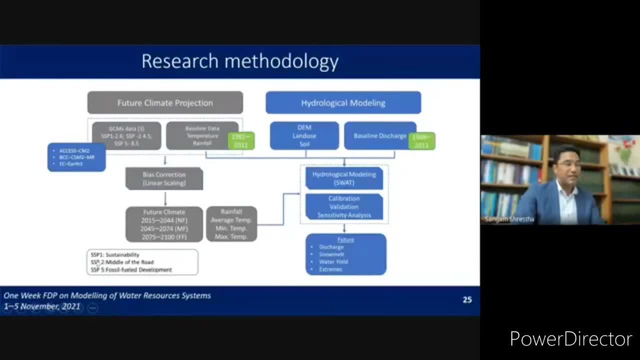 So you know there are. There are five SSPs, data available and the meaning of these SSPs are how the socioeconomic development will take place in future, Because the greenhouse gas emission depends on the, you know, socioeconomic development and also the different kind of climate change mitigation and adaptation policies. 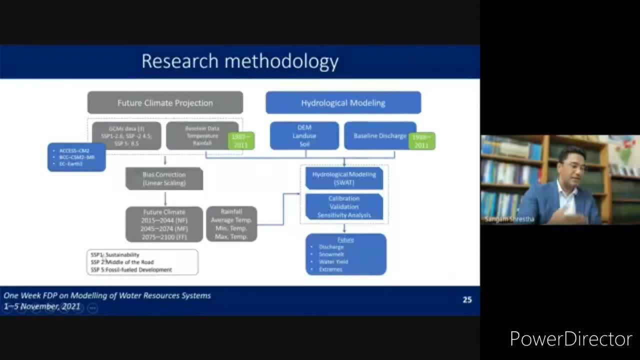 So there might be different kind of scenarios That will generate different concentration of the greenhouse gases in the atmosphere in the future. So, since we do not know how exactly the socioeconomic development occurs in the future, so there are several scenarios proposed here And based on that there are different, you know climate data that are available. 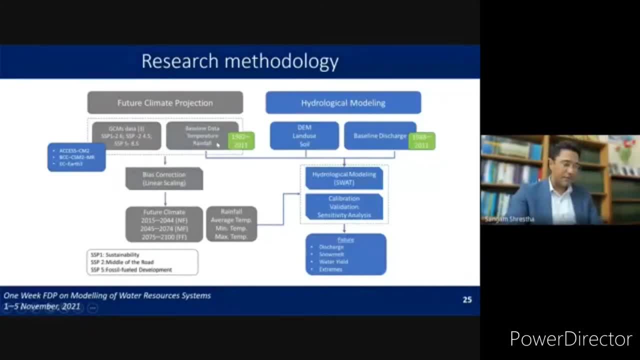 We also have the baseline data of the temperature and rainfall of 1982-2013.. And we have the baseline data of the climate change mitigation and adaptation policies. So we have the baseline data of the climate change mitigation and adaptation policies And we have the baseline data of the climate change mitigation and adaptation policies. 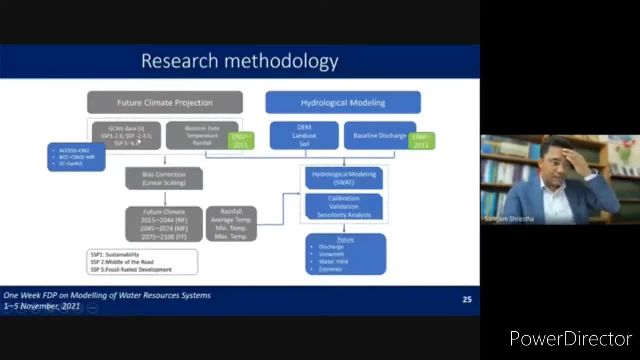 And we have the baseline data of the climate change mitigation and adaptation policies. As I've mentioned previously, there are a number of scenarios that we can use in these significant environment. In some people there may be some allons at the localㅠ which may cost Rs. 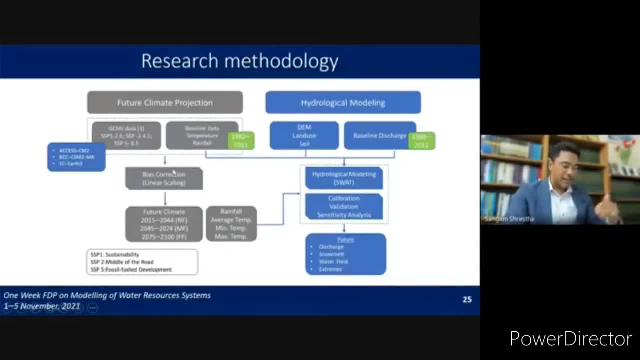 20,000, handwriting to see them and materials to deuit at the bol gam and in some people may cost Rs 150,000.. So we may have to look at all the solutions. So if there are opportunities to work to customs block metrics to assist with the 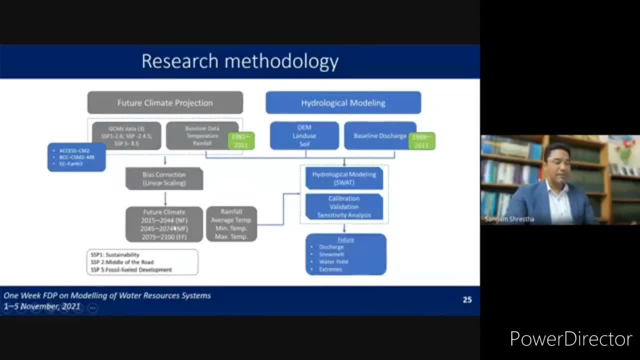 R Sem, to generate the future climate data into the three future period. one is called the near future, the second one is called the mid future and the third one called the far future, and these time period is having 30, 30, 30 years. so we have the data. 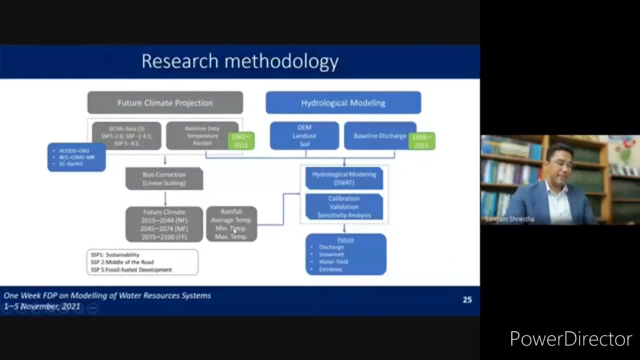 of rainfall, average temperature, the maximum temperature and and minimum temperature of the daily resolution. and once we have these future climate data, we can feed these future climate data into the hydrological model and we can simulate the. you know how hydrology or hydrological processes changes in the. 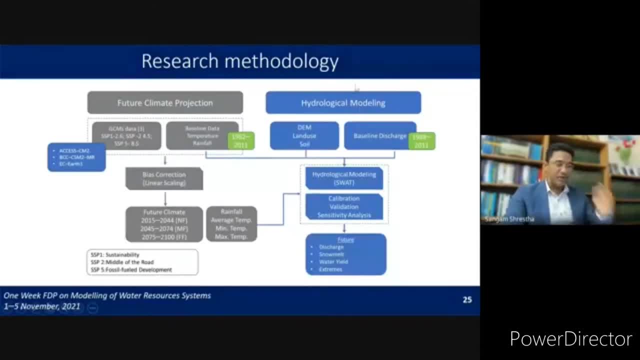 future. so the second step is hydrological modeling and in the hydrological modeling we use this model called soil and water assessment to and this model is developed by USDA in collaboration with the Texas A&M University, and this is a physically based semi distributed hydrological model which can simulate the hydrology, the water balance component, sediment. 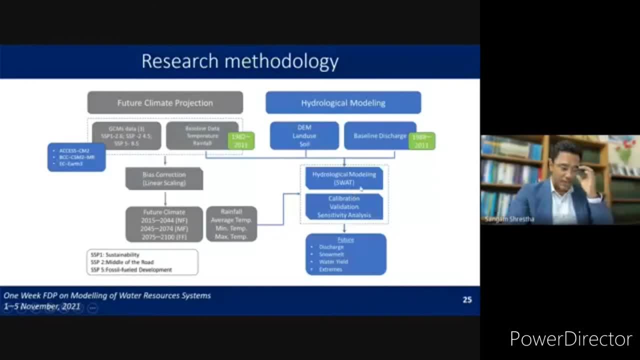 yield, groundwater and so on. you also have the- these you know: introduction of the SWAT model and how to use SWAT model in the subsequent session. so the the SWAT model is calibrated and validated by using the discharge data of 1988 to 2011. so once we have these calibration and validated, 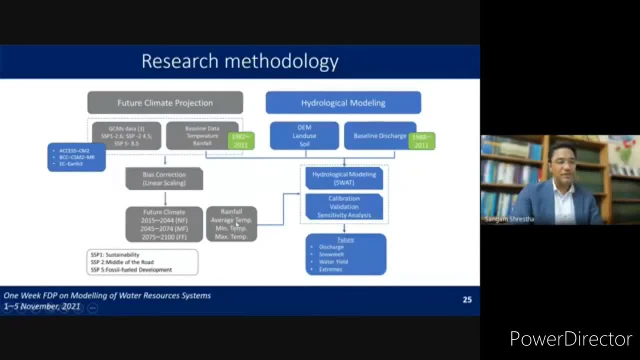 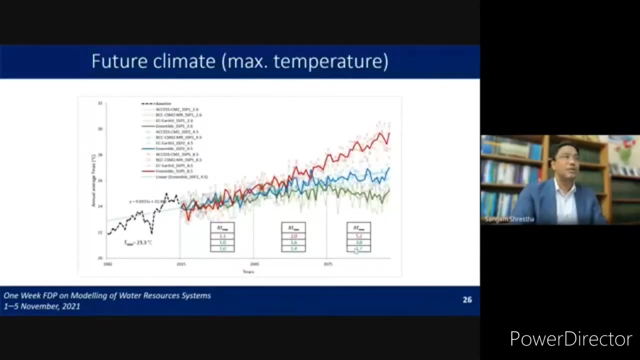 hydro, the SWAT model. we use this future climate data to see how the future discharge, snowmelt, water yield and some of the extreme hydrology changes in this river basin. ok, i'll be presenting a few results from this case study. one is the future climate in terms of the maximum temperature. we we see that the maximum 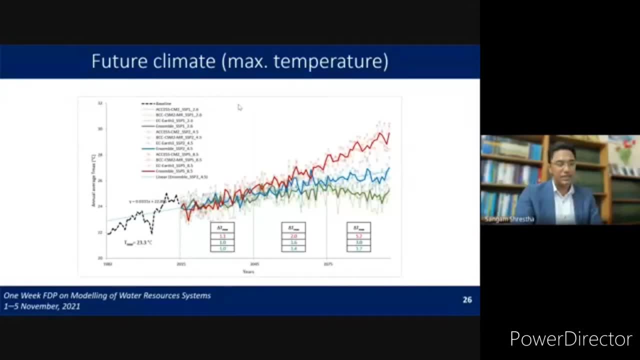 temperature will be increasing in the future in this basin. so in the x-axis you can see the time period and y-axis you can see the annual average temperature and until 2015, this is the you know baseline temperature, which is the historical observed temperature. okay, and even you can see that, this you know historical temperature. 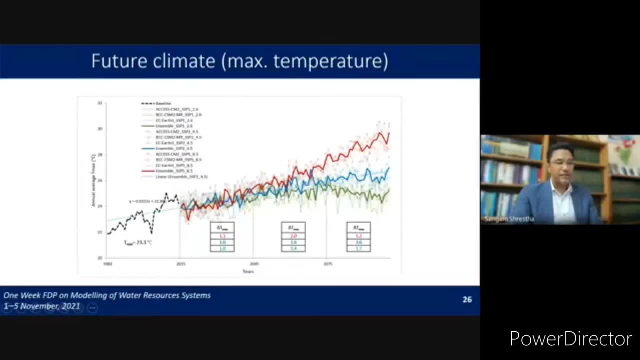 is increasing in the basin right and after this you can see several lines, and these several lines are the temperature projected by 3 G C M's under different SSPs or shared socio-economic pathways. and please just look at these bold line and these bold line- the green line- is the 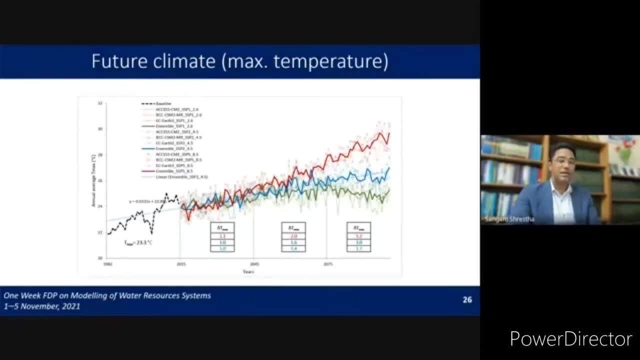 the ensemble of of the the SSP1,. the blue line is the ensemble of the SSP2, and the red line is the ensemble of the SSP5.. So the ensemble are the average of these three GCMs And you can see that in all the future time period the average maximum temperature is: 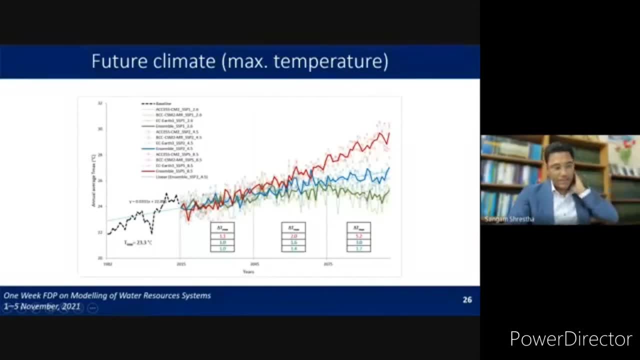 increasing And the increment is different for different SSPs. For the SSP1,, of course, the temperature is increasing, but increasing at the lesser rate than the SSP5. So here in the table I summarize what is the change in the average maximum temperature. 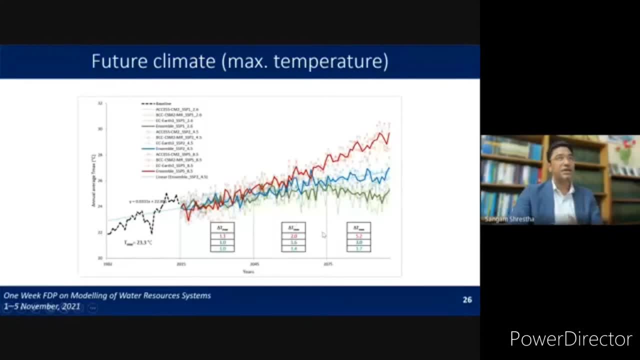 in these three different time periods. For example, by the end of this century, the average maximum temperature will be increasing by 5.2 degrees centigrade with the scenario of SSP5, whereas it will be increased by 1.7 degrees centigrade under SSP1. 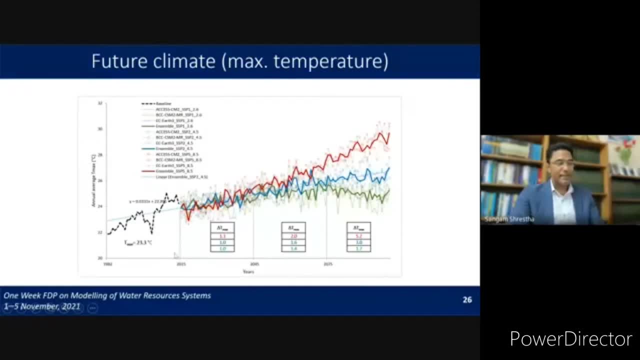 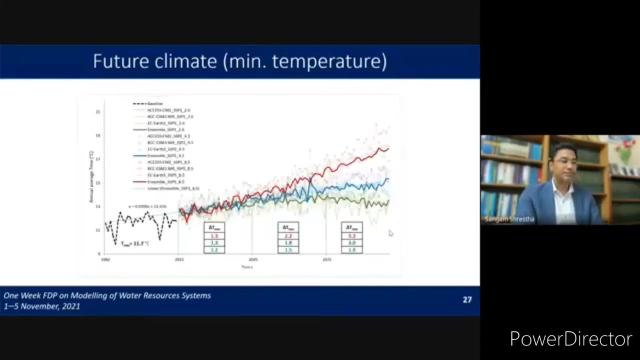 So it means that the average temperature will be increasing. There is a lesser increase of temperature under SSP1 and higher increase of temperature under SSP5. But you can see that the temperature is expected to increase in all the future time period in this Marsang De River basin. 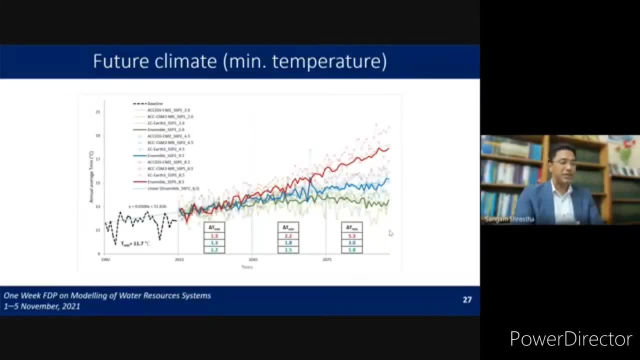 This is the result of the minimum temperature. 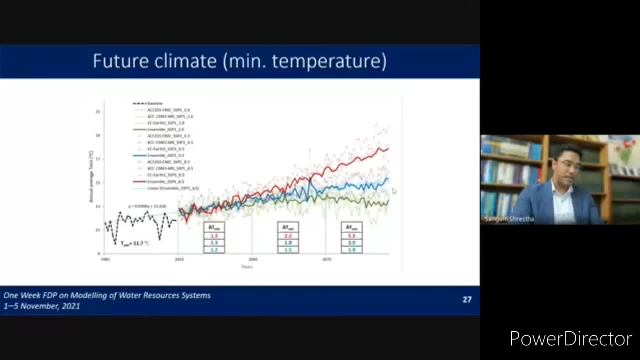 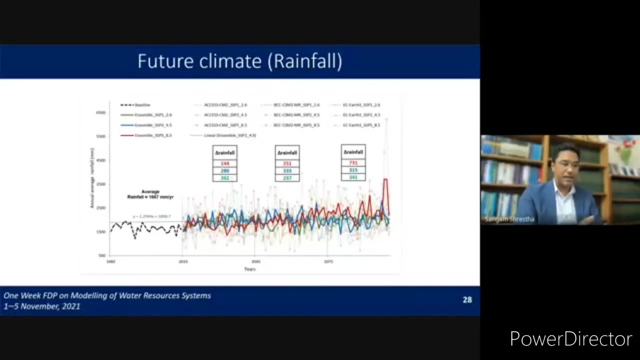 If you look at this table I have prepared here, so in all the future scenarios, in all the GCM, they are projecting that the rainfall is increasing in the future or the Mustang River Basin. 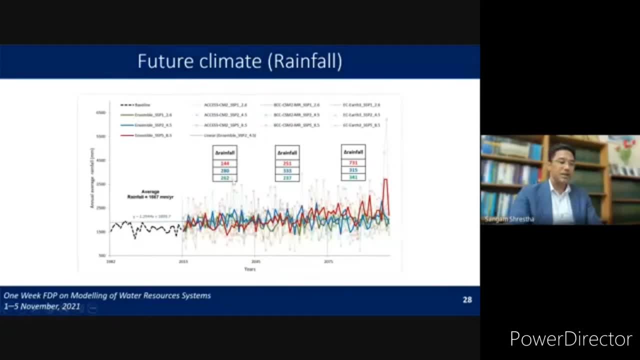 is getting wetter in the future And then also the change in the rainfall is given here. For example, by the end of the century in the Mustang River Basin the rainfall is projected to increase 731 millimeter annually compared to the average annual rainfall now. 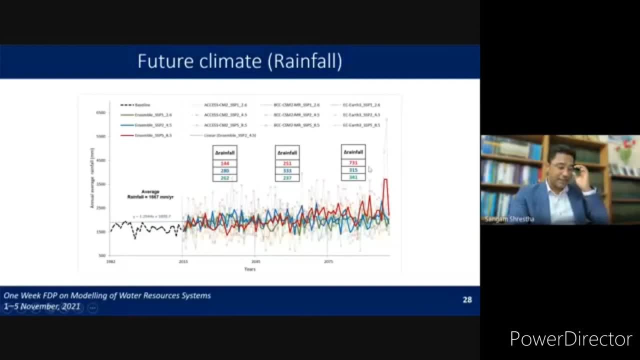 So it means that by the end of the century the rainfall will be 1,667 plus 731.. So it's It's more than 2,300 millimeter in one year, right? So the basin is expected to be wetter. 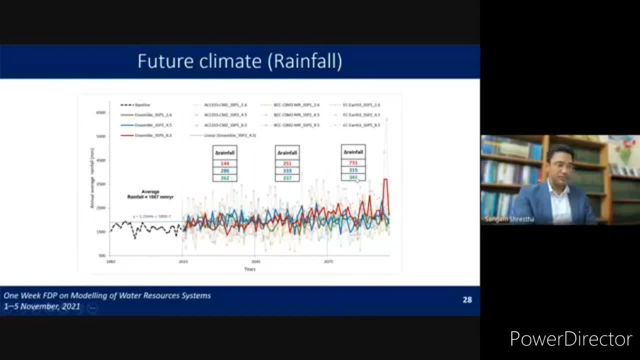 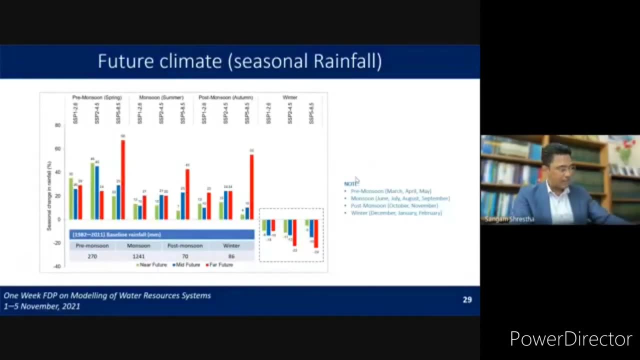 in the future in all the climate change scenario. So the temperature is getting warmer and the rainfall is also getting higher in the basin, But I tried to analyze how the rainfall is going to change on a seasonal basis. OK, So climate change will impact not only the average rainfall. 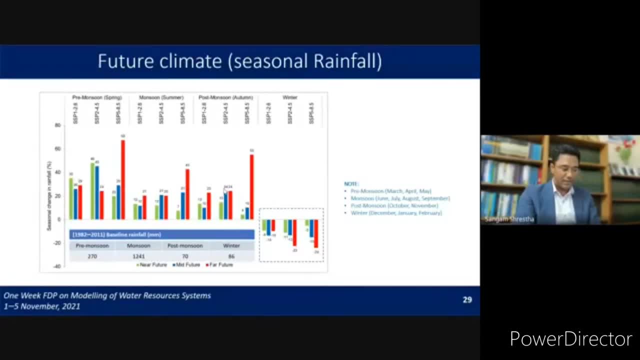 but also the seasonal rainfall, intensity of rainfall and so on. So in this graph you can see how the rainfall is going to change in the pre-monsoon, monsoon, post-monsoon and winter season in the basin. OK, 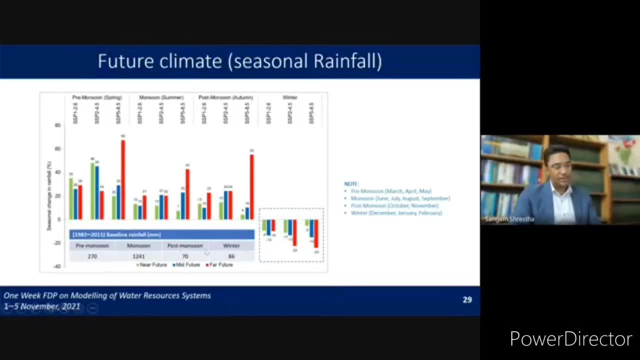 So this table shows that the rainfall is going to change- the baseline rainfall in different season. okay, and the graph shows the percentage change in the seasonal rainfall compared to the baseline period. so you can see that in all the seasons the rainfall is going to increase in the 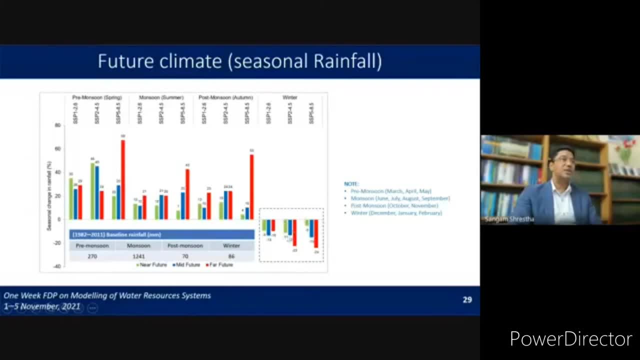 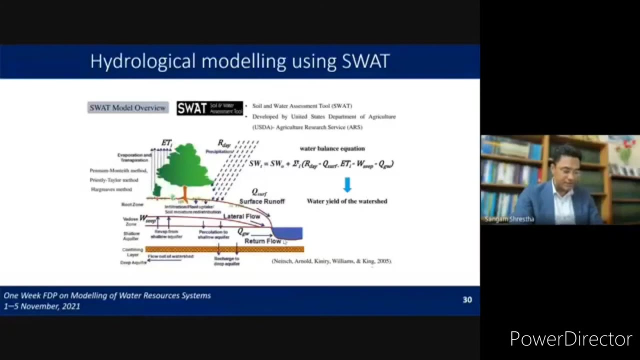 future, except the winter season. right, so in the winter season the rainfall is expected to decrease in the future? yeah, okay, so, as I mentioned that in this case study we used SWAT model to simulate the how climate change impact the hydrology and water resources. I will not explain. 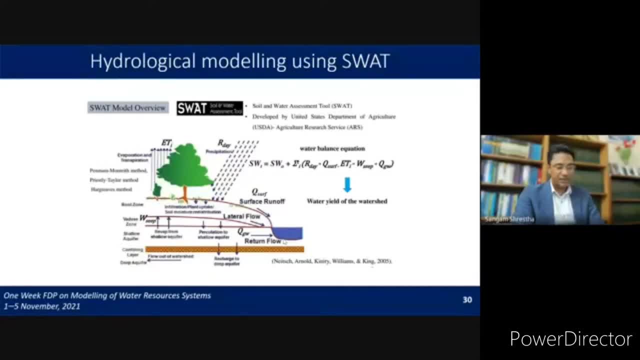 in detail here because I see that there is a- you know, separate session for SWAT model. so basically, SWAT model is a continuous, physically based semi distributed hydrological model and it has been widely used in several parts of the world to assess the- you know- impact of climate. 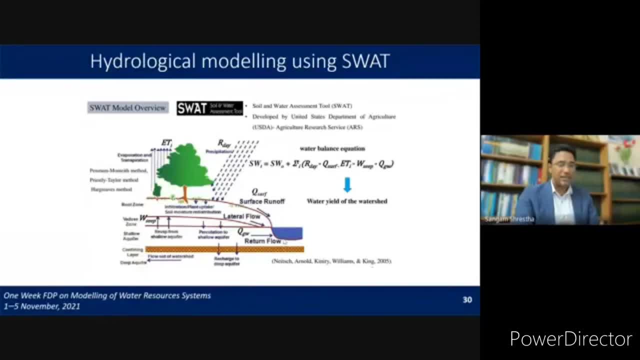 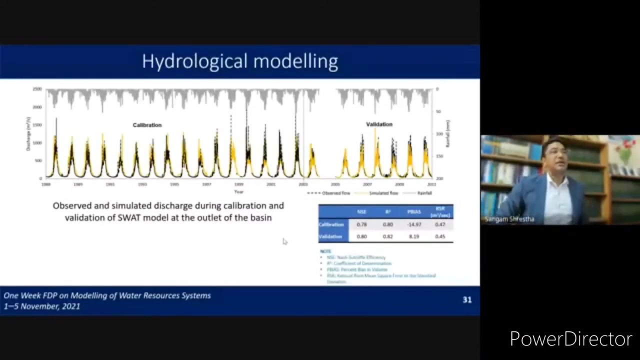 change, impact of land use and land cover, change for solar and energy consumption in the world, in particular, water resources management studies. so it's quite popular model and in this study also we have used this SWAT model to simulate how the climate change, you know, impacts the, the hydrology. okay, so, as I mentioned before we we calibrated- 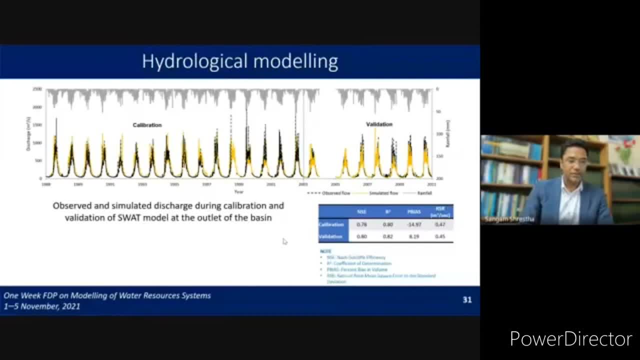 and validated the SWAT model. to see how the SWAT model captures the hydrological processes of the enable basic and the calibration invalidation were performed at the basin outlet and also the opposite Ramof. this hydrograph you can see here is observed and simulated this charge during. 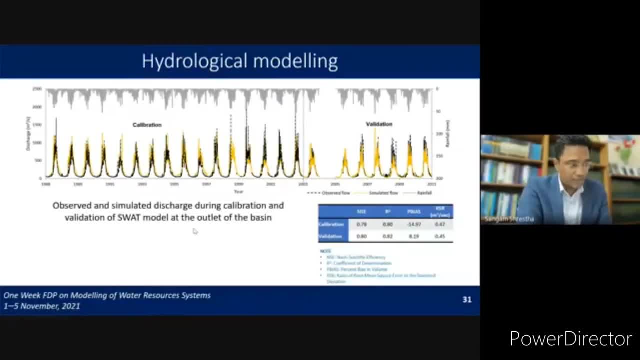 the Calibration and validation at the outlet of the basin. okay, x-axis is the time and Y-axis is the discharge, and you can see that the dotted lines are the observed discharge Whereas the colored line is the simulated discharge. So I presented both, you know, calibration and validation hydrograph here. 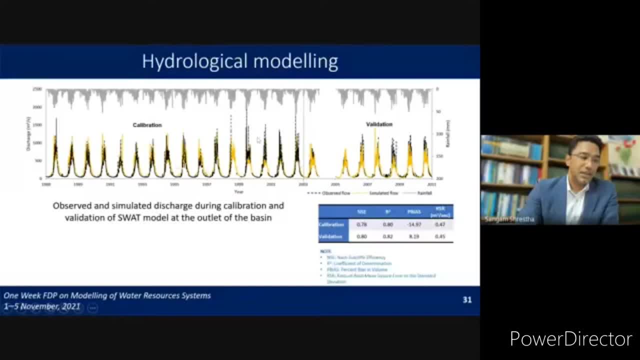 It. It is quite matching. So it means that the, the SWAT model is, you know, accurately simulate the- you know- hydrological processes in the river basin. The table here it shows the some of the statistical indicator to see what is the, you know- closeness between the, the. 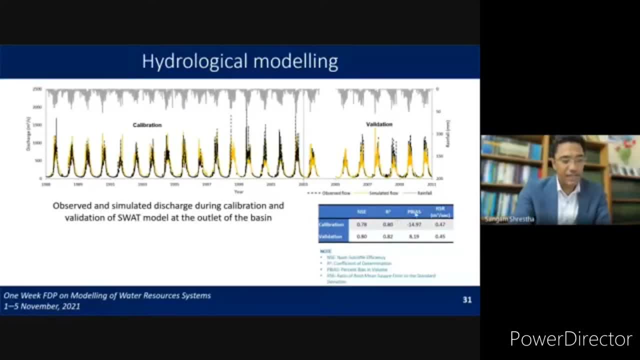 simulated flow and observed flow during the calibration and validation. So the statistical indicator are NASA efficiency coefficient of determination, percentage bias in the volume and also the Ratio of the root minus square leader to the standard deviation right. so we have used this for indicator to see What is the performance of the SWAT model. 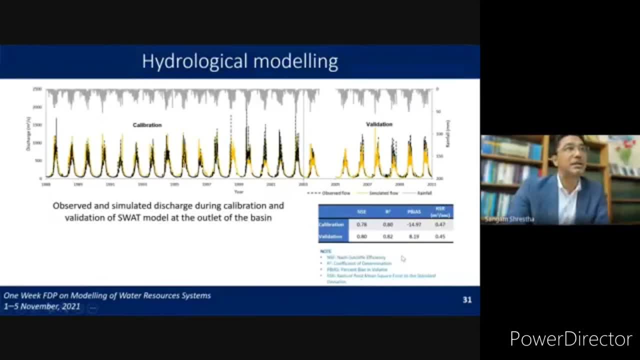 to simulate the flow and You can see here, you know All of the statistical indicators values are quite high: NSE. if it is close to one, we We assume that the model perfectly simulates the flow. Again, I square: if it is close to one, we also assume that the the model simulates the flow very accurately. and 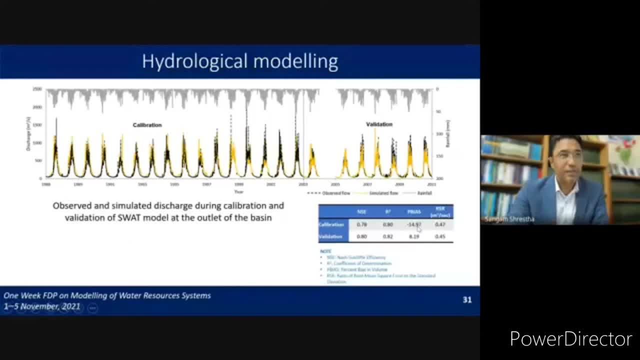 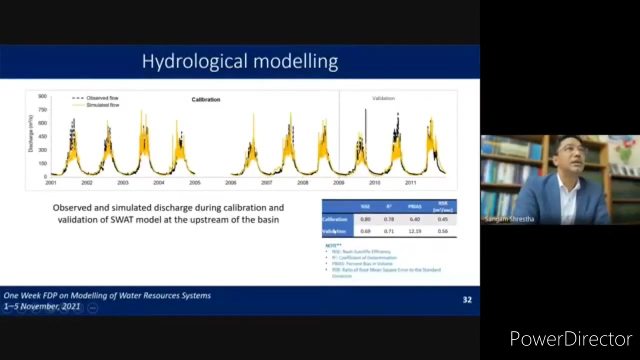 and the lesser the value of the p bias and RSR, the better the performance of the model. okay, so if the model, You know, has the p bias of the plus minus 15%, We say that the model is simulating the flow very well. similarly, we calibrated and validated the 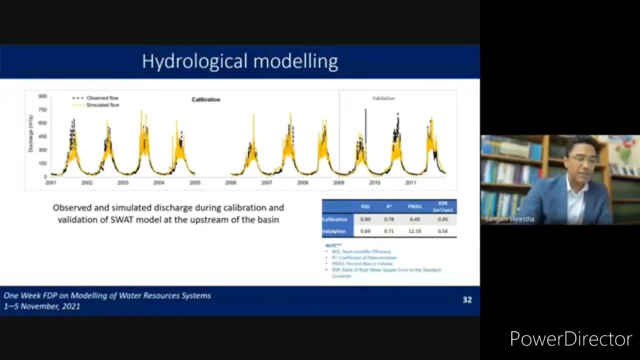 model In the opposite stream of the basin and you can also see here the comparison of the observed and simulated discharge during the calibration and validation Phase. and in this table you can see the value of the statistical indicator of NSE I, square p bias and RSR, so similar to 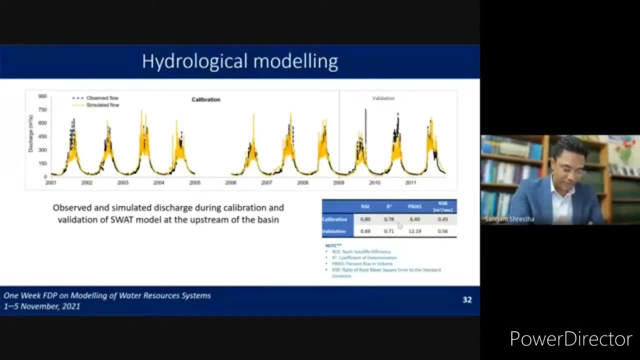 downstream of the basin, upstream of the basin, has also Very good, you know, performance of the SWAT model to simulate the flow and we assume that This model is is very good to use to simulate the climate change impact on the hydrology and water resources of the Merchant River Basin. 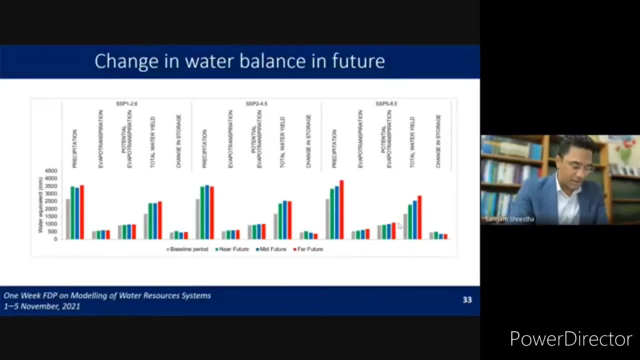 Okay, so I will present some of the results of climate change impact on the hydrology and this slide is basically the change in the water balance and other component of the Merchant the River Basin in future and this Bar diagram shows the You know change in the 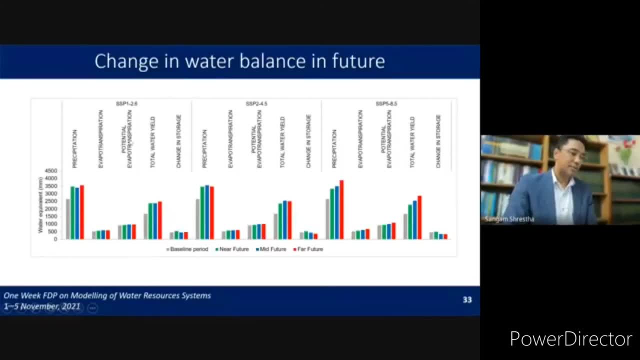 precipitation, evapotranspiration, Potentially evapotranspiration, total water yield and the change in the stories under three SSP scenario, which are SSP 1, SSP 2 and SSP 5. Okay, and these different colored bar diagram are the baseline period, which is the gray gray color and 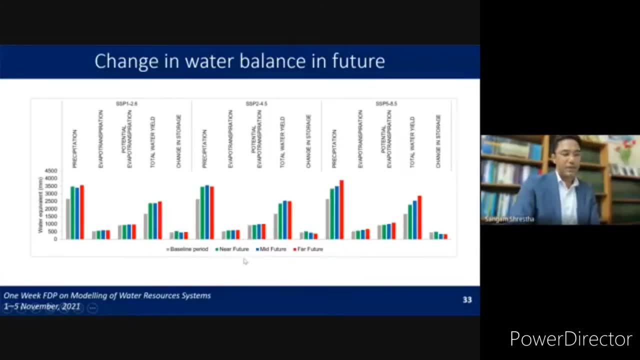 The green color is the near future and the blue is the mid future and the red is the far future, right? So You can see that the precipitation In the future is Expected to increase, okay, In all the SSPs. similarly, Total water yield is also expected to increase in the future, right? 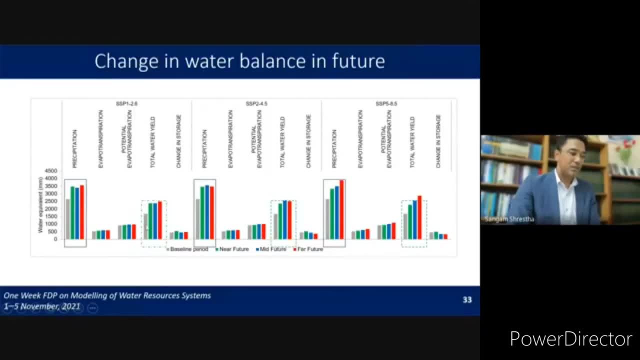 So, for example, in SSP 1 the baseline water yield is about 1600 millimeter, but in the future it might increase up to 2500 millimeter. So this the water yield is how much amount of water is Going out of the water set right. So in terms of the 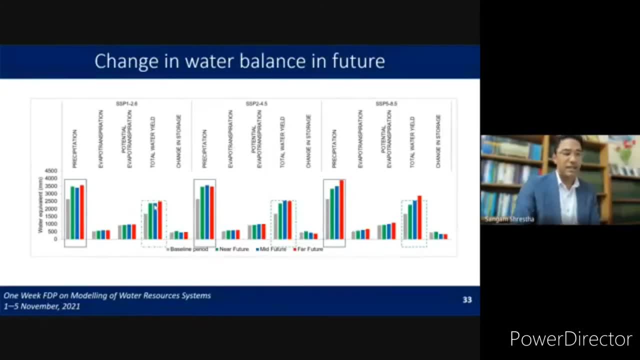 surface flow plus ground water flow, Yeah, minus the transmission loss. So in the particular, you know, case study, We have estimated the water yield on a sub basin wise. So I will show you that the special pattern of the change in the water yield in the 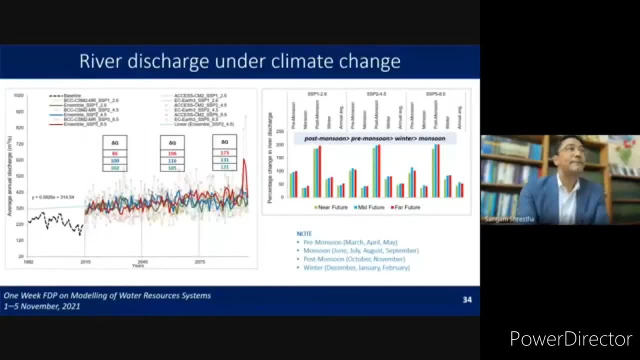 subsequent slides. This is the change in the river discharge under climate change scenarios. so on the left-hand side you can see the average annual discharge in the baseline period and also in the future period. The X axis is the timeline and y-axis is the average annual discharge. and 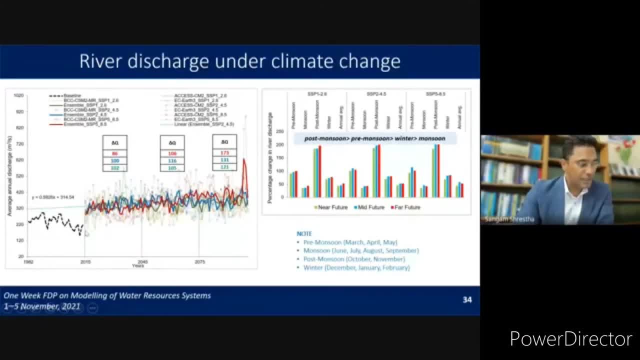 in Inconsistent with the change in the rainfall or increase in the rainfall, the, The average discharge, is also expected to increase in the future. Okay, So again you can see that the solid, the bold, solid colored lines are, You know, the the average annual discharge in the future. 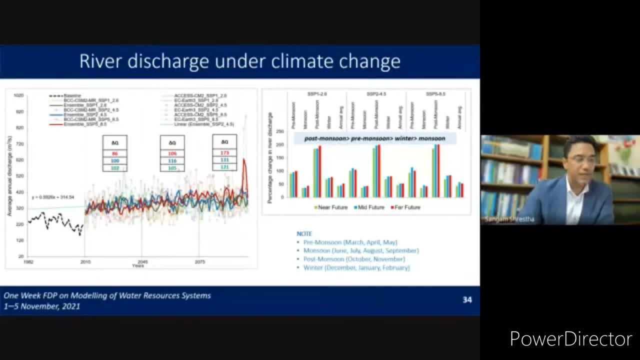 under three, three SSPs: SSP 1, SSP 2 and SSP 3. SSP 1 is green color, SSP 2 is blue color and SSP 5 is red color. So The change in the annual discharge I have calculated and put it in the form of table here. 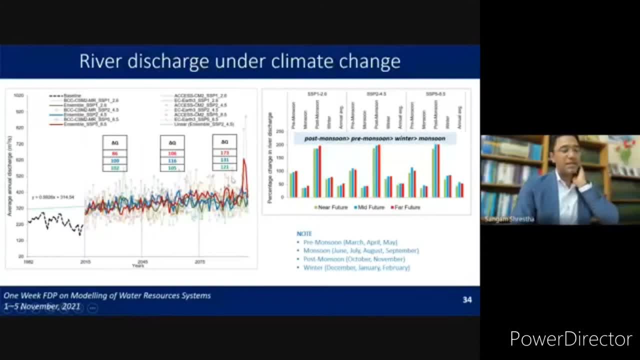 so the change in the discharge is higher in the end of the century right. so By the end of the century the, The annual discharge will be increasing by 173 cubic meter per second Compared to the baseline average. similarly, in SSP 1, the average annual discharge will be increasing by. 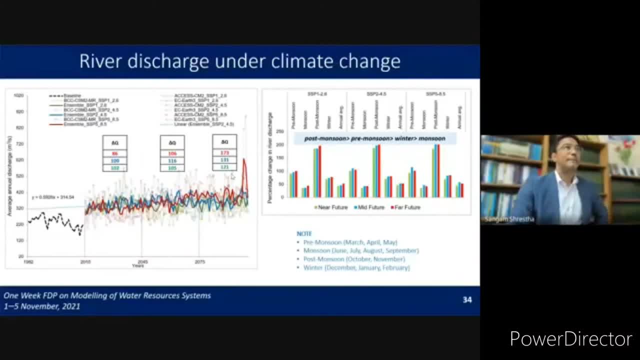 121 cubic meter per second. So we analyzed how the river discharge is going to change in different seasons. These seasons are pre monsoon, monsoon, post monsoon and winter and you can see that different months are allocated for different seasons and The the percentage change in the river discharge is higher in post monsoon and 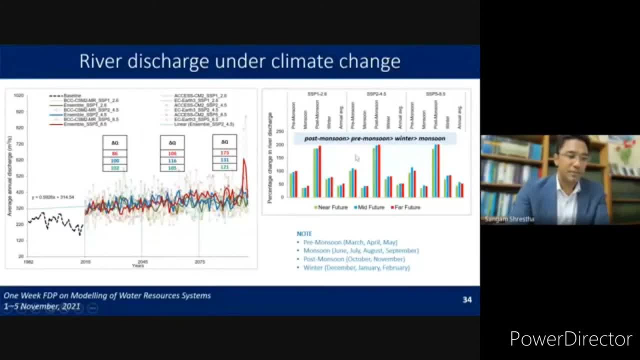 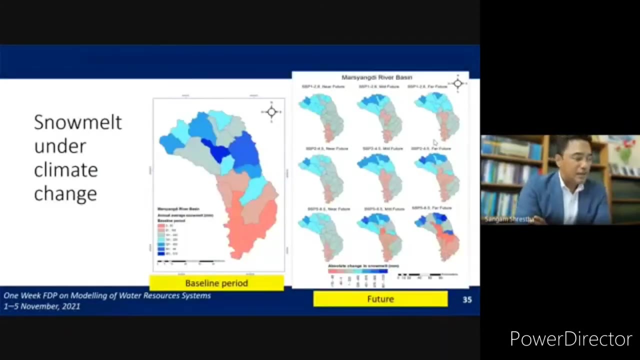 lesser in monsoon. So the post monsoon, pre monsoon and winter season discharge increases are higher compared to the monsoon season discharge in this river basin. Okay, this Map shows the snowmelt under climate change. So I have prepared the spatial- you know, variation of the change in the snowmelt under the climate change scenario and 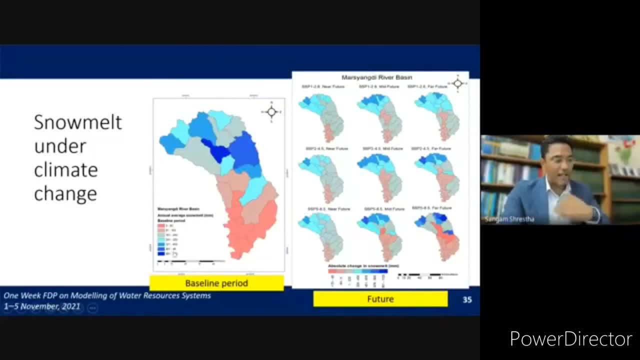 This darker, you know blue color- are higher snowmelt. so on the left-hand side, This is the snowmelt in the baseline period, right. so the snowmelt Is higher in northern part of the basin. okay, and in future. we found that these snowmelt. 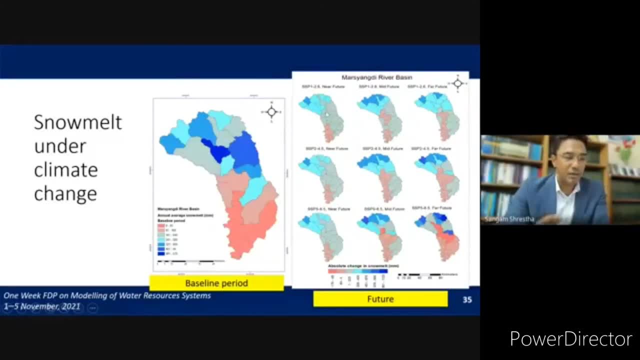 is going to be increased in the northern part of the basin because of the- you know, snow cover area located in these northern part of the basin. so So in all SSP you can see that these blue and darker blue color These are the you know snowmelt under climate change and you can see the absolute. 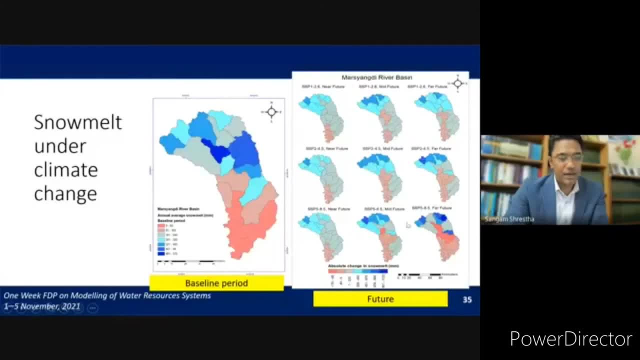 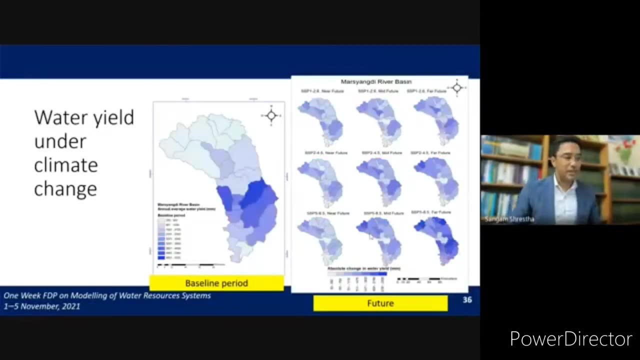 Change in the snowmelt in the northern part is higher than the other part of the basin. Similarly, we also calculated how the- You know- water yield will change in different sub basin. to see the spatial variability of the water yield under climate change and on the left-hand side. 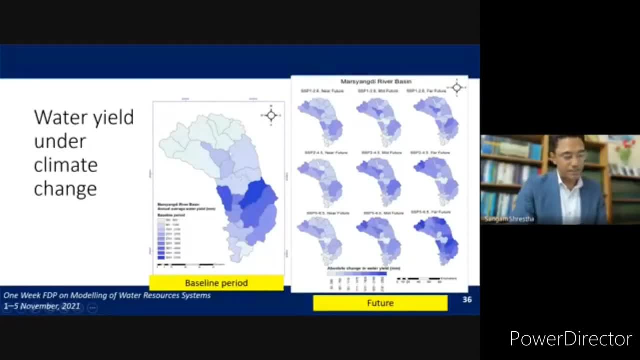 This is the water yield in the baseline- Okay, no climate change. and then the right-hand side is the water yield under the climate change conditions, Under SSP 1, SSP 2, SSP 5, and there are all the future period, right near future. 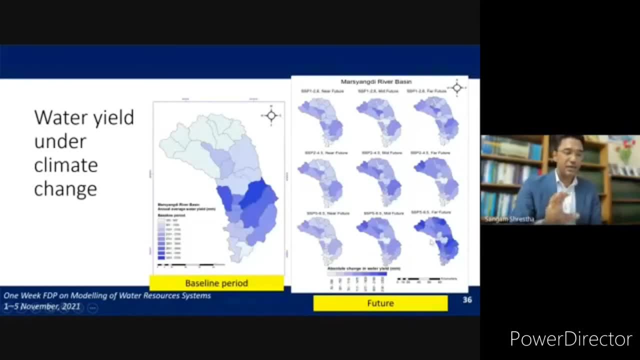 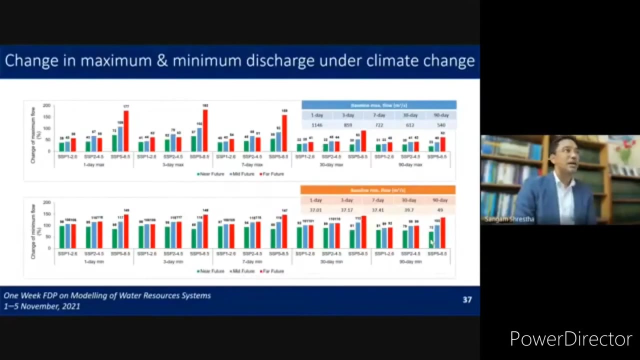 mid future and and far future. And you can see the northern part and the central part of the sub basins Are having higher water yield compared to the other parts of the basin. Similarly, we calculated the change in the maximum and minimum discharge under climate change. so, as I mentioned in the previous, 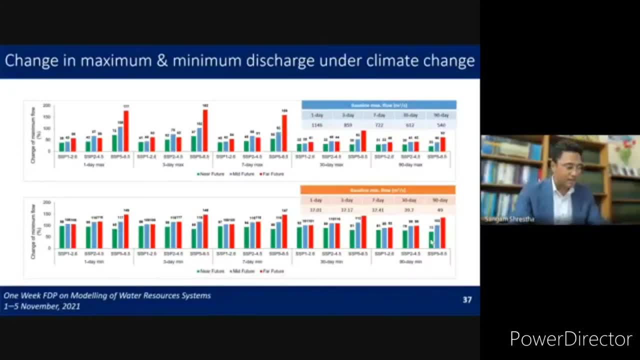 slides that It's very important to understand. you know the the several components of the discharge, Not only the average discharge but also the maximum and minimum discharge. so the upper bar diagram shows the change in the maximum discharge and the lower bar diagram is the change in the minimum discharge. and 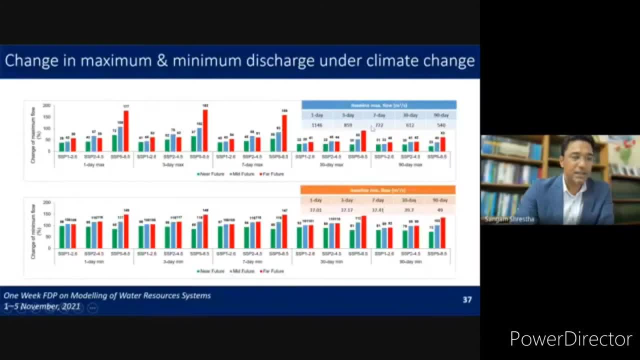 The table you can see here. These are the you know, baseline maximum discharge and baseline minimum discharge and the. the indicators of the Maximum discharge and minimum discharge are one day maximum, 3 day maximum, seven day maximum, 30 day maximum and 90 day maximum. and you can see here in both of the 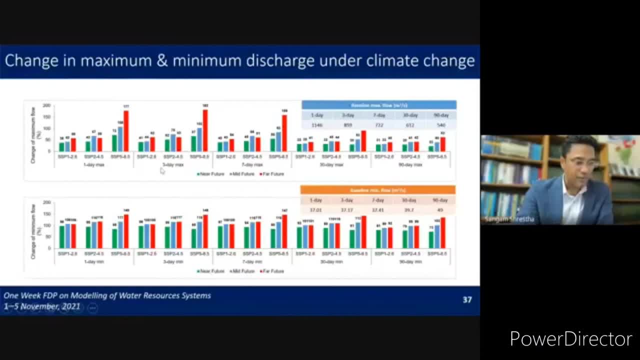 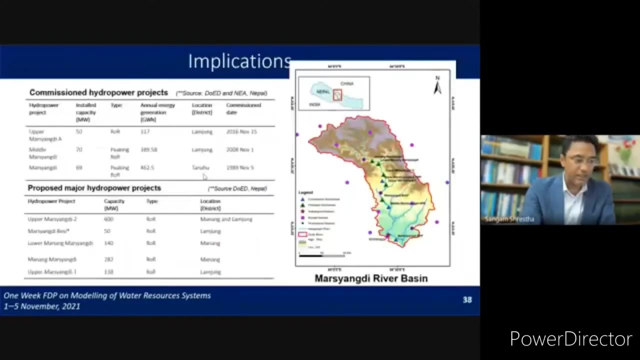 you know, indicator maximum flow and minimum flow. These you know discharge will be increasing in the future. Okay so, And this might have several consequences on the hydropower projects, As I mentioned in the beginning that this basin has three commissioned hydropower projects. 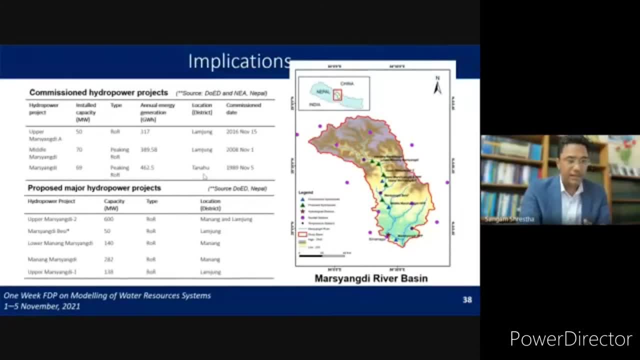 and also five hydropower projects are under planning. So of course, availability of water is increasing. Maybe it is beneficial to the hydropower project because they can produce more hydropower. At the same time, if the maximum flow are increasing, then it might bring floods into the basin. 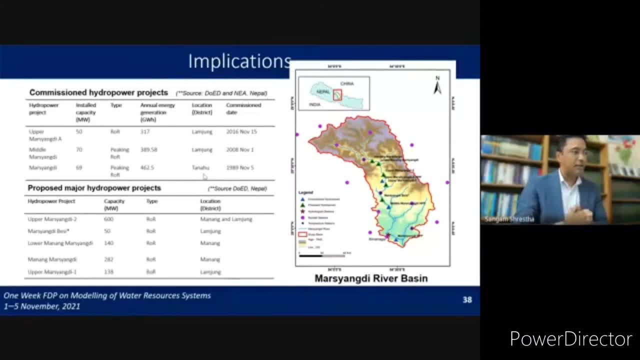 So if there are floods then probably the several facilities of the hydropower projects are under risk. Maybe it will destroy the several facilities Such as intake, probably the hydropower plants, dams. So there might be risk for the hydropower project which can be analyzed and several 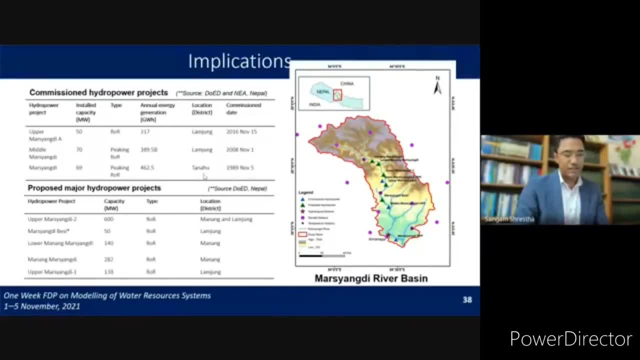 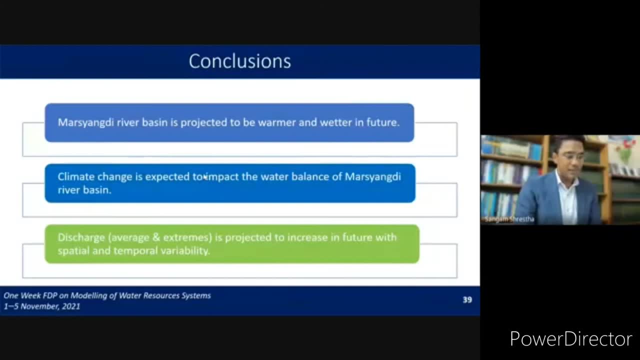 adaptation options can be proposed in this river basin. So these are the conclusions I want to make from this case study. So, as you rightly know, Notice that the basin is projected to be warmer and wetter in future And the climate change will bring impact on the water balance. 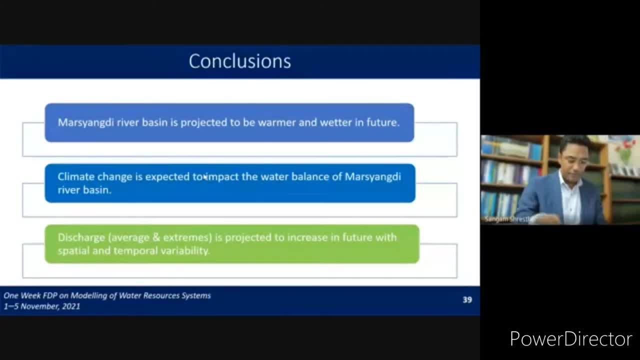 Water balance consists of rainfall, runoff and other components like ground water, lateral flow and so on. So it's not only for the hydropower projects perspective, But also for the other water resources management objectives. If the water balance changes- probably you know- the planning has to be done accordingly. 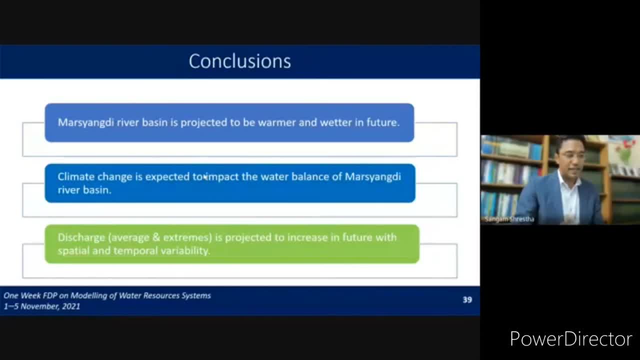 And the discharge, both average and extreme discharge, are projected to increase in the future. But it has both spatial and temporal variability and it's very important to consider how these- you know- Change in the discharge, Change in the flow In terms of the average discharge, maximum and minimum discharge will impact the hydropower. 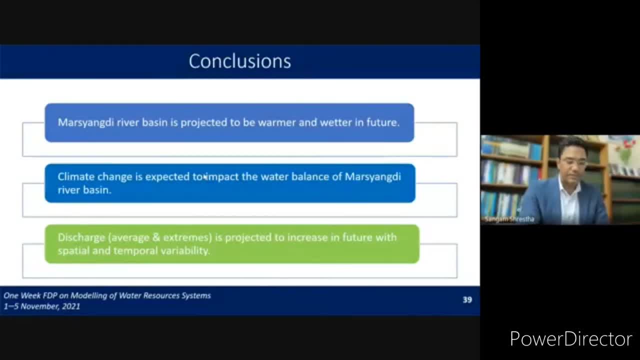 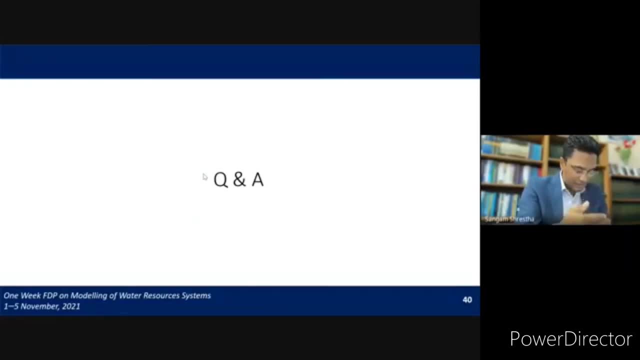 projects and hydropower facilities, hydropower production. So with this I will stop here and maybe we can also have some discussion on this. you know case study, Professor Ajay. yeah, if there are any questions, I'll be very happy to. 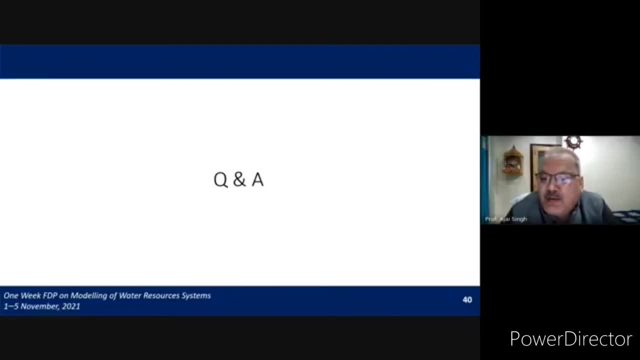 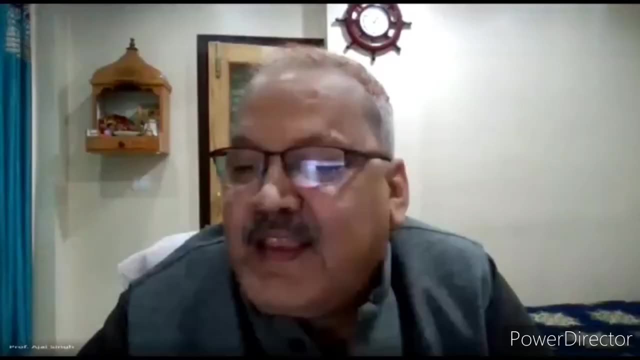 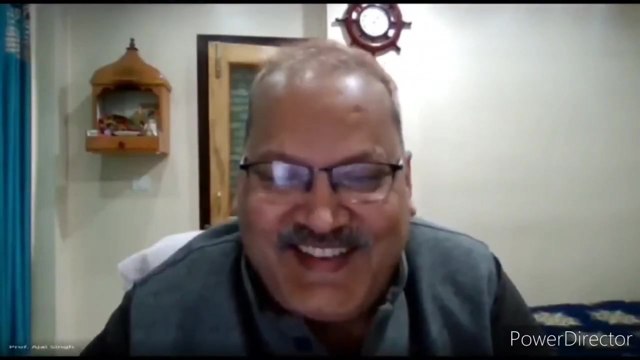 Yes, there are three, four questions in the chat box. You please go through it. One question is there from Rinky Dronc. She is saying that she wanted to do the PhD under your guidance. Yeah, I'll be very happy to accept you for a PhD in AIT. 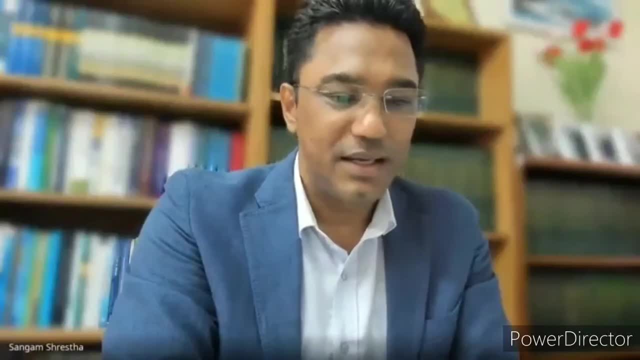 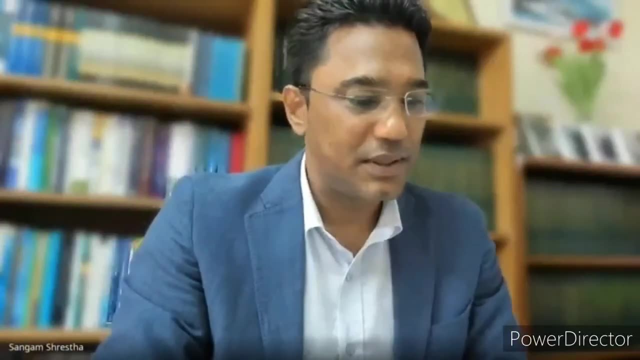 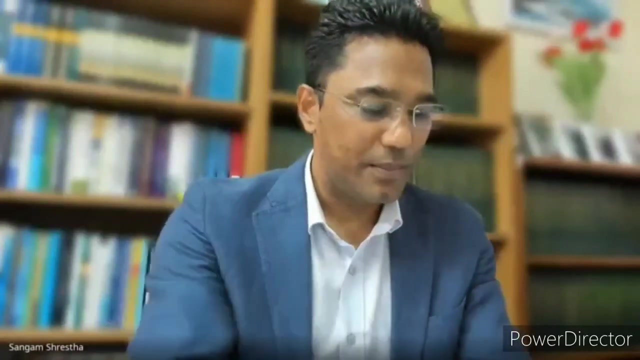 So I will accept you. Thank you very much, Thank you. Thank you. I suggested to submit your application. do you know the website of AIT and also website of WEM? maybe I can quickly, you know, give you the WEM website and the. 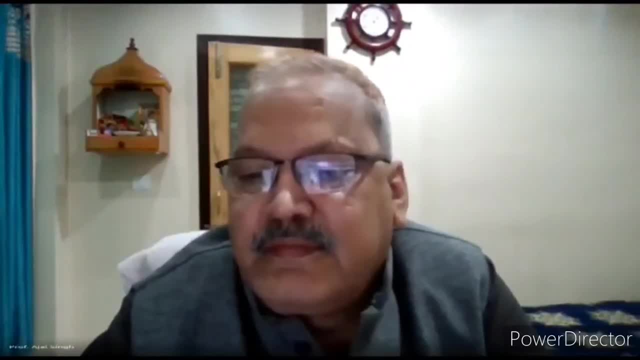 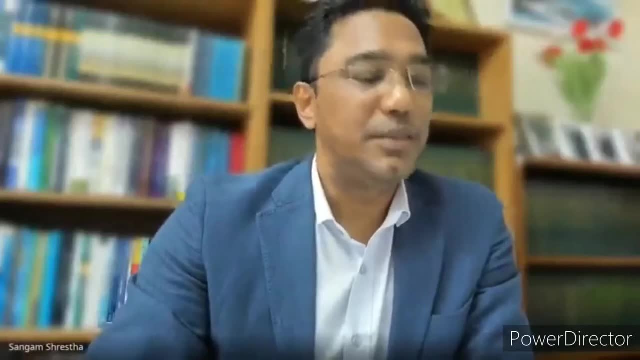 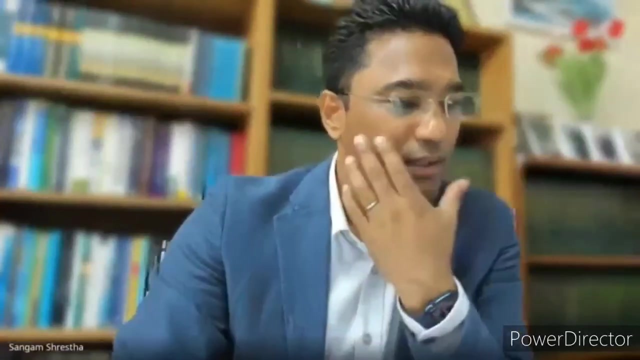 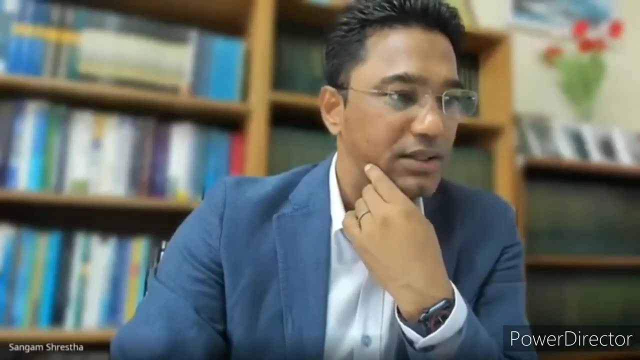 last date when they should apply. yeah, actually there is no deadline for the PSD application. all right, the PSD application is year-round. yeah, and we have two session. one is the January session, start from first week of January and the other one is the August session and we have the scholarships. 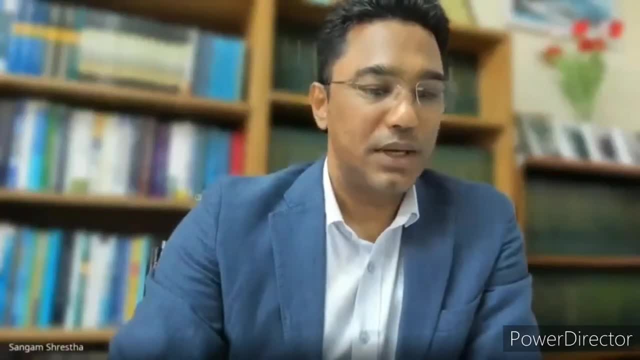 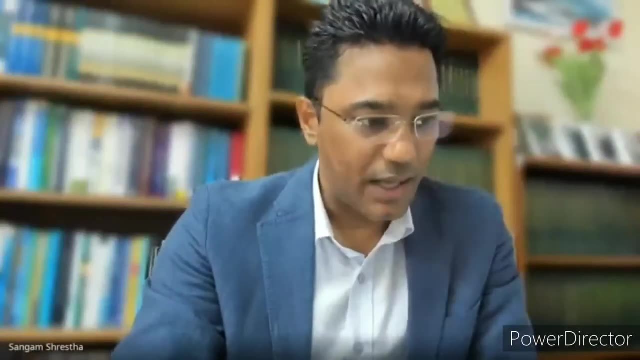 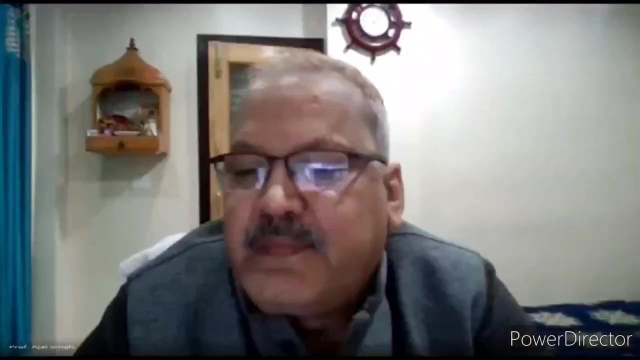 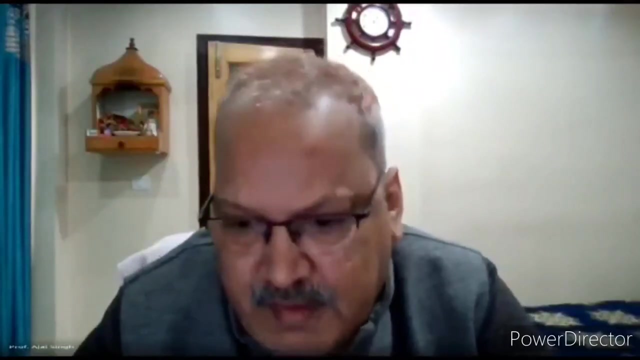 available for the August session. so if you are interested, you can apply now and we can evaluate for the January intake or as well as for the August intake. so I have put this website. Rinki, you please prepare a good statement of purpose and the research proposal, and that will be good. so all the best. yeah, Rinki, please send me. 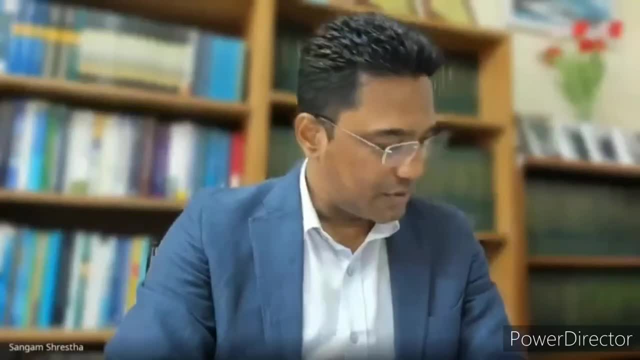 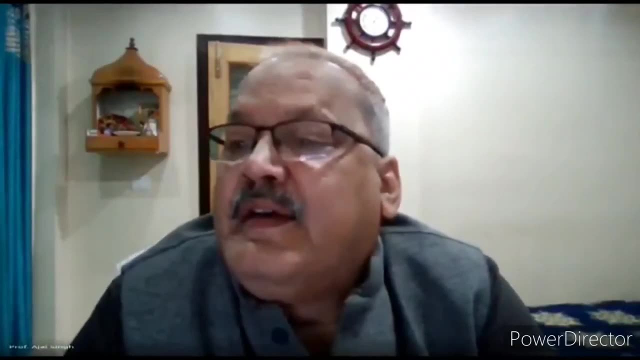 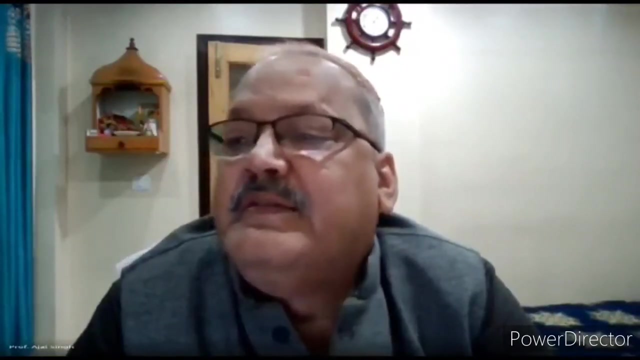 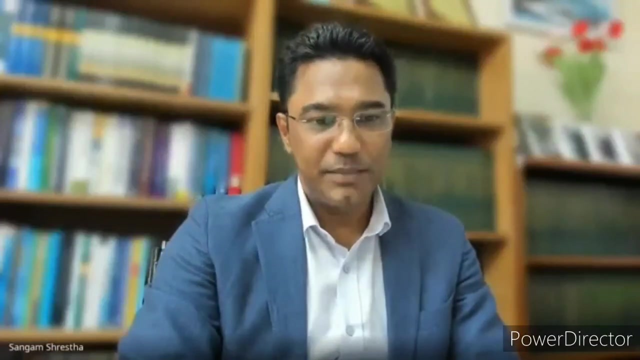 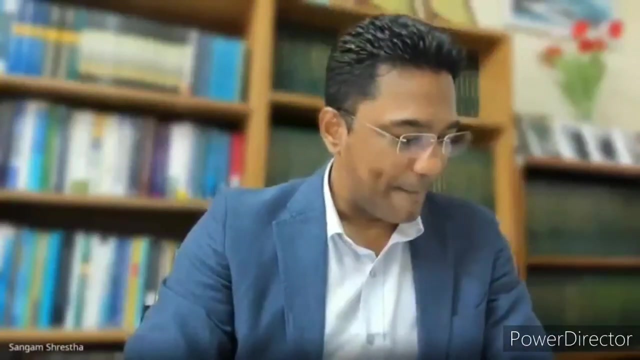 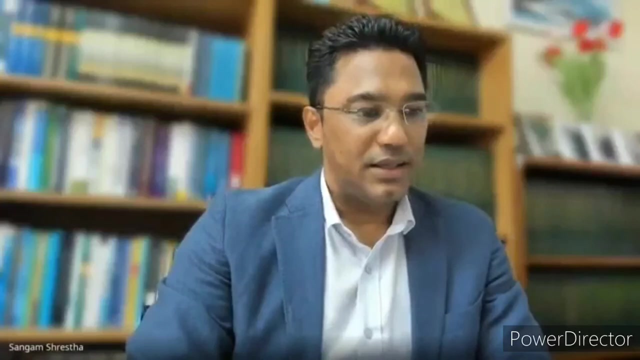 email and I will support you for your applications. yeah, yeah, that's great. is Vanitha Pandey how you du travailler ng�navd s? no, we're doing our homegrown. Where I work, there is a holiday. she's asking that whether you did this study for sediment here. um yeah, Vanitha, I did not do the sediment healed study in this study, but it is good that you have the marcyan. the river basin is mountainous basin and providing me with all the facilities in cinemas. 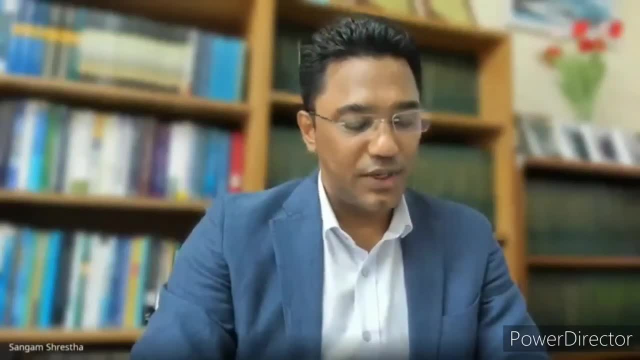 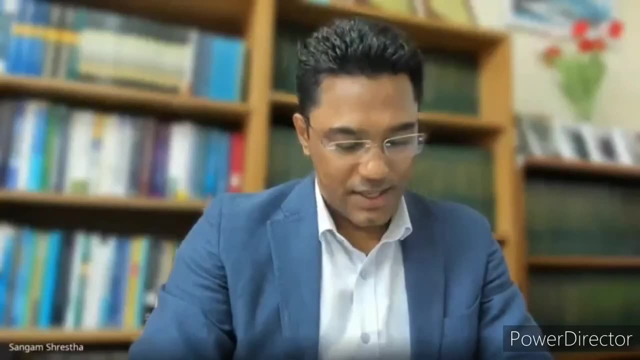 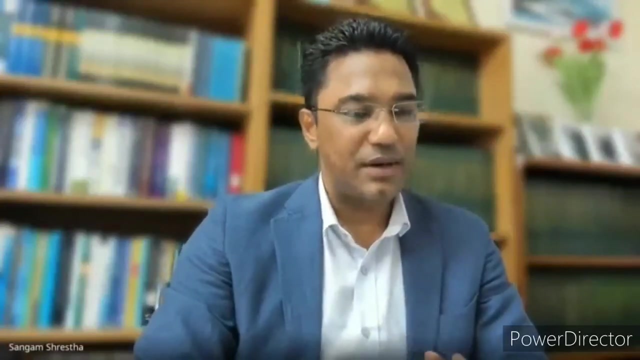 climate change would bring impact on the soil erosion and sediment yield and that will impact the hydropower project and this is very important and I was discussing with my former student that we should do a resiliency assessment of hydropower project under climate change. so it means that sediment yield study is 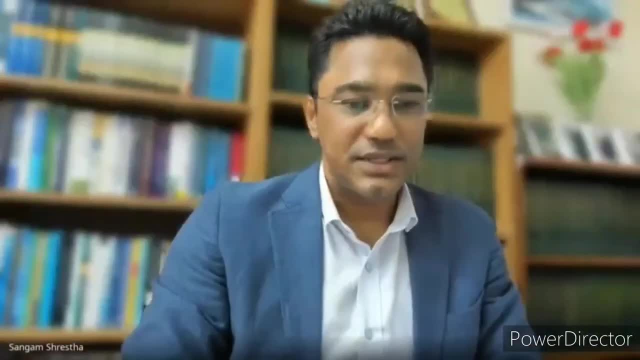 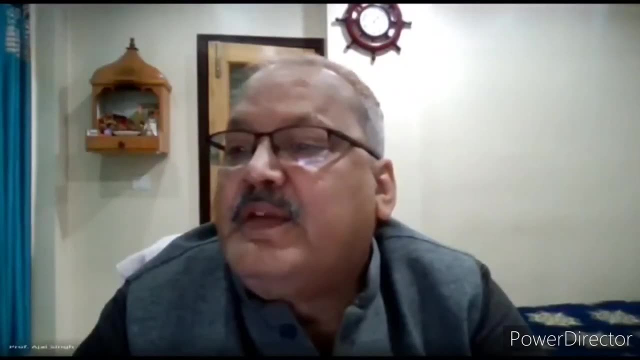 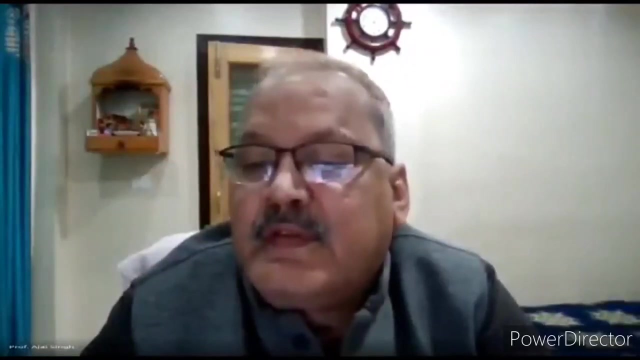 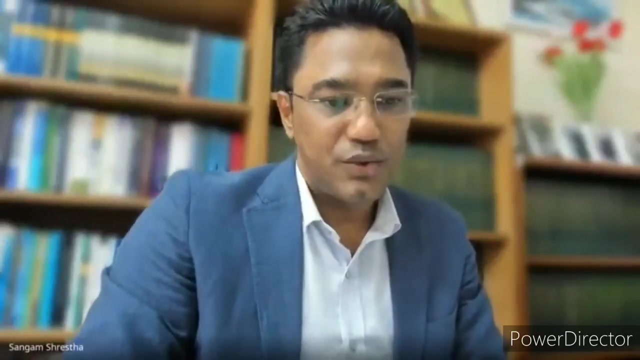 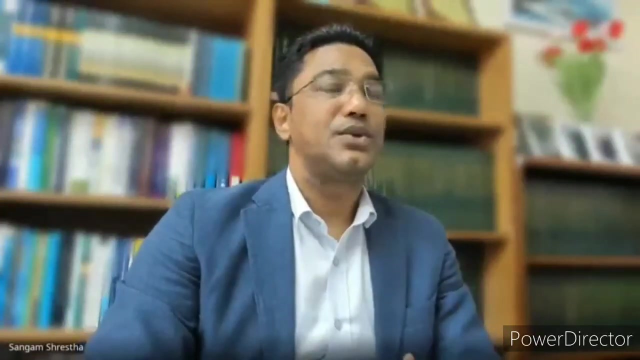 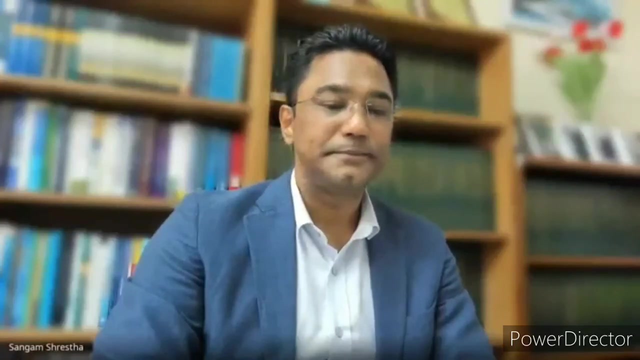 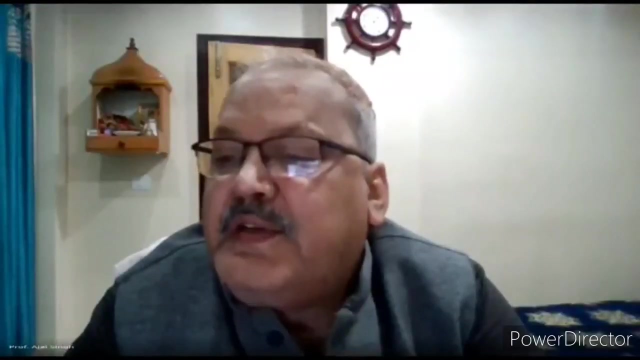 very, very important. yeah, that's a good suggestion. only one gauge station, so how to validate upstream discharge data? Suman, if you remember correctly, I presented the calibration and validation in two locations: one is at the basin outlet and another is in the upstream. so, yeah, right, yes, right, right. then Divya. Divya is asking: sir, why did you? 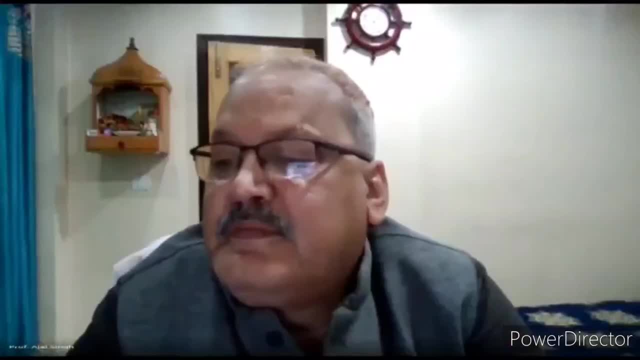 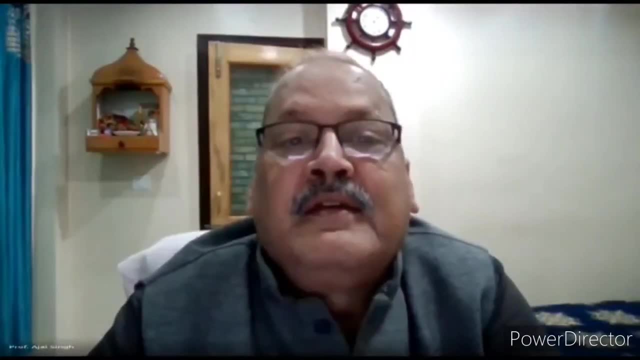 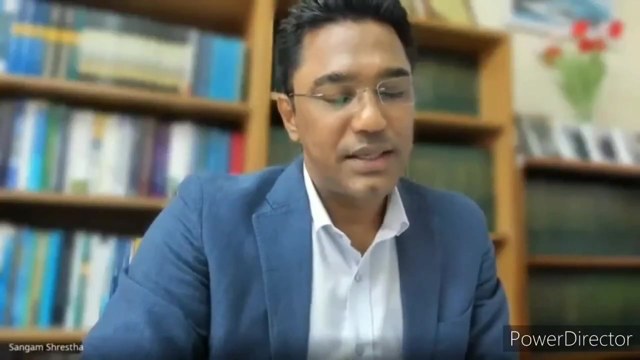 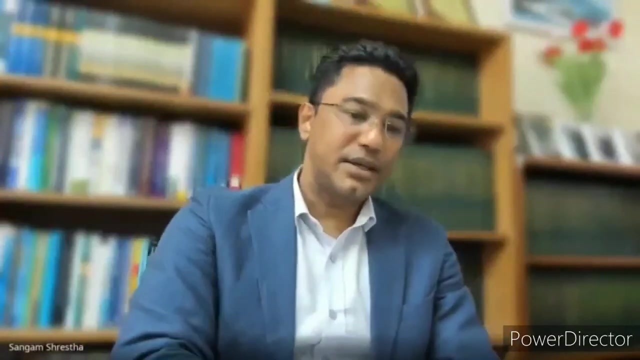 consider only three GCM, why you have considered three GCM. okay, uh, Divya, Divya, Divya. that's very good question. so there are two questions here I can see. one is: why did you consider three GCMs? and the another question is for bias correction. 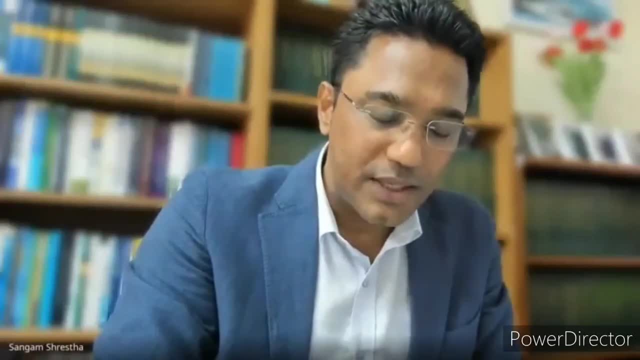 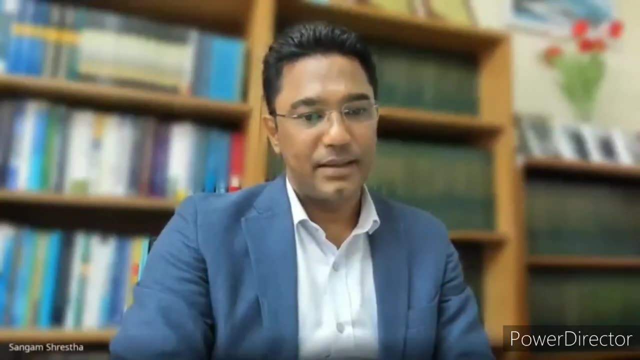 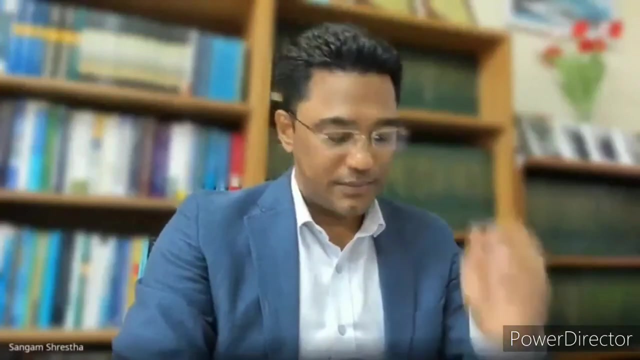 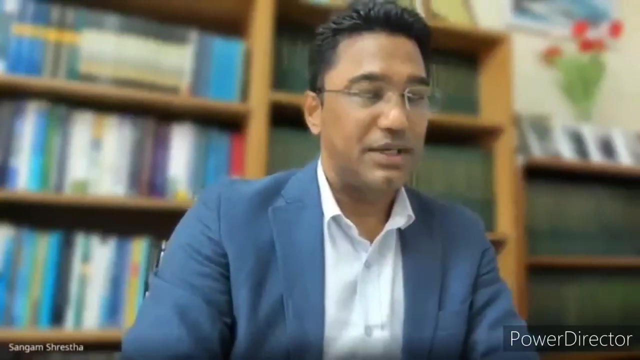 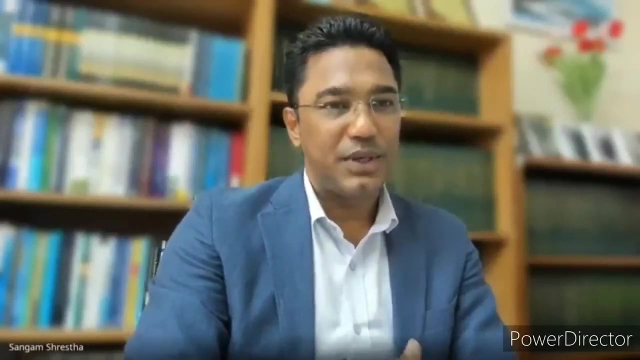 have you adapted linear method for both rainfall and temperature? okay, yes, in the bias correction, yeah, we used the linear scaling for both temperature and rainfall. so the the question of the, you know, selection of the three GCMs is very, very important. yeah, in fact, we we have to use as many number of GCMs as possible because you. 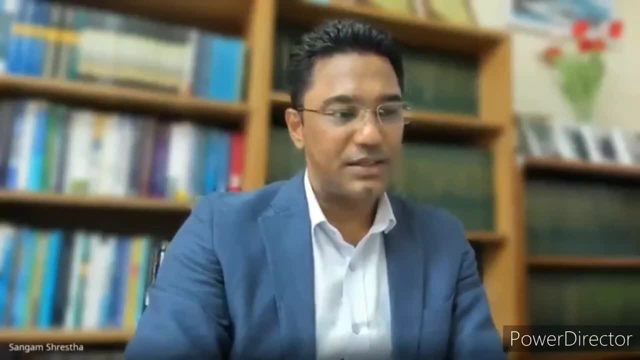 know there are a lot of uncertainties in climate change projection, right, so probably many of the GCMs- they can simulate many GCMs for this type of climate change and it is very important the climate differently, right, And we do not know which GCMs. 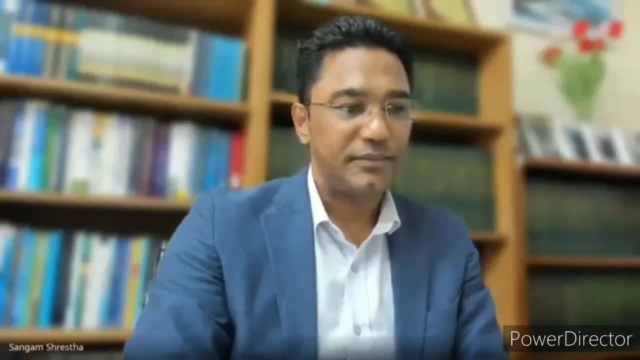 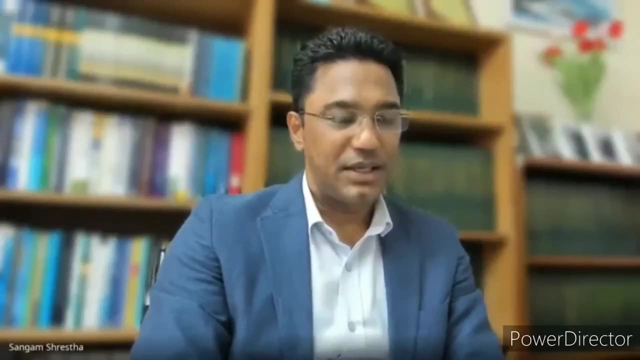 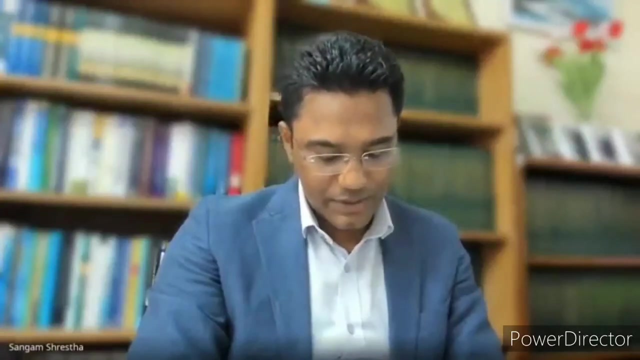 will simulate the climate accurately. So in that case it's always better to have these multiple GCMs, you know, to project the future climate scenarios and then use those multiple GCMs- the future climate scenario- for the climate change impact assessment studies. 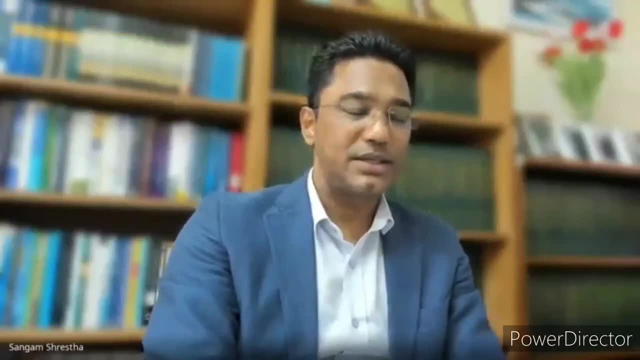 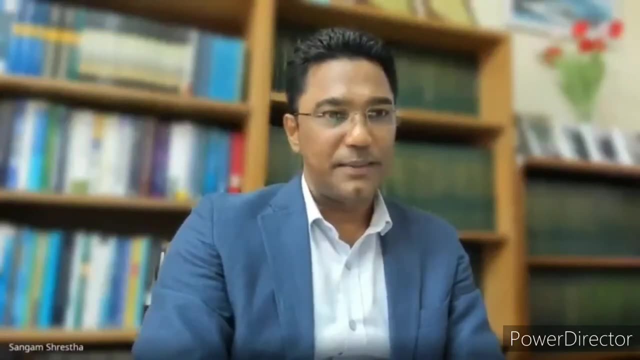 You know, maybe one GCM can simulate wet conditions accurately and another GCM can simulate the dry conditions accurately, right? So because different GCMs, they have different kind of structure, They use different kind of equations, although the- you know- boundary conditions. 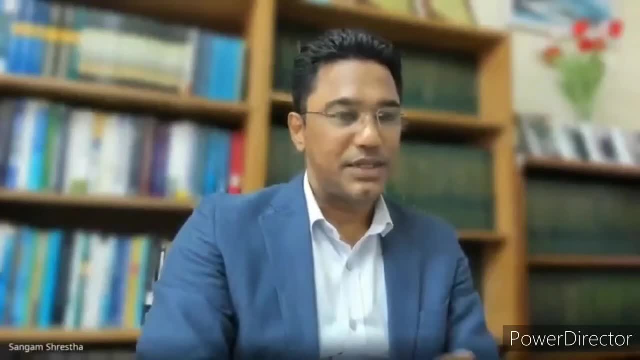 and initial conditions are same. okay, Because they are developed from different modeling centers and the performance of these GCMs probably vary from one GCM to another GCM. So that's why we use more number of GCMs, But in this particular study we used only three. 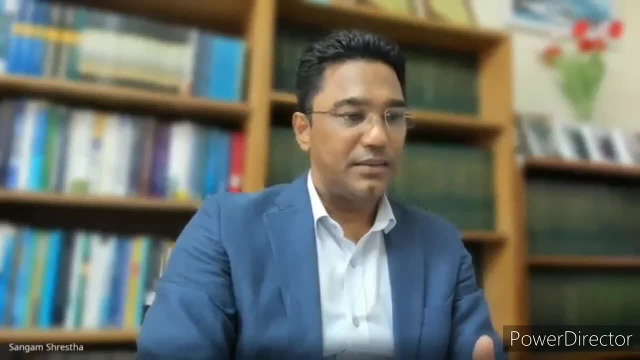 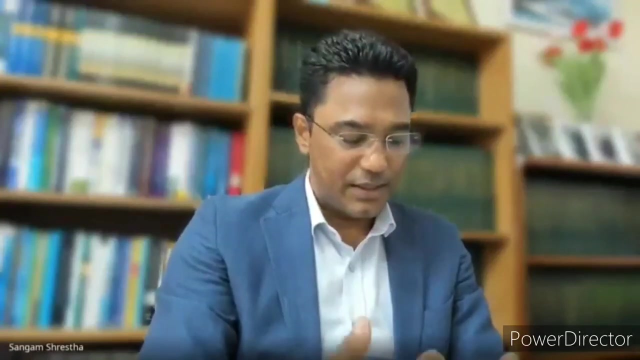 again because of the limitation of the time. But yeah, I have several students. they are using 20 or 30 GCMs also, basically for the PSD. so my suggestion is: you know, the larger the number of GCMs. 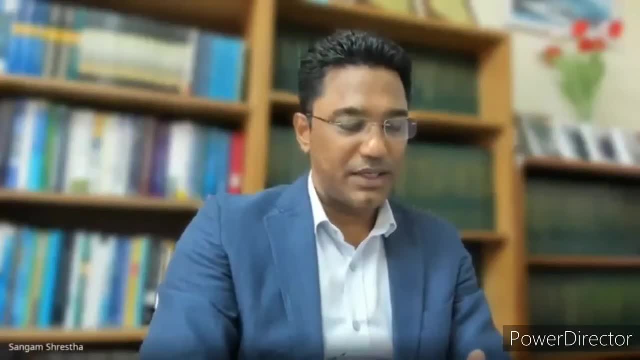 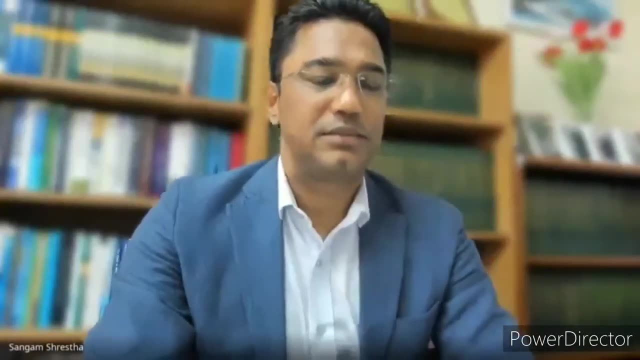 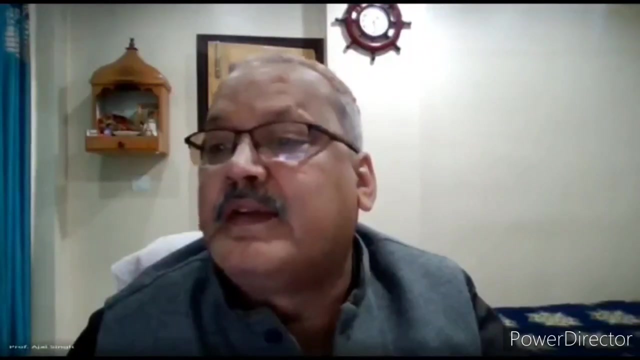 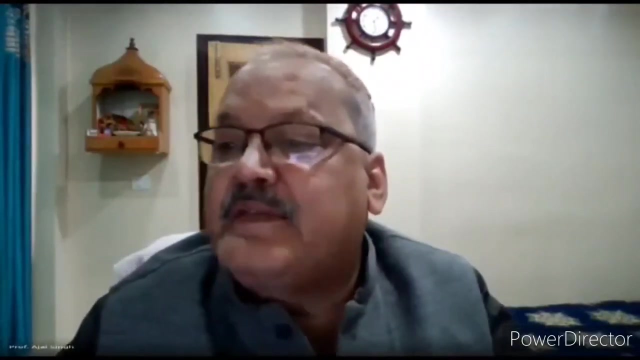 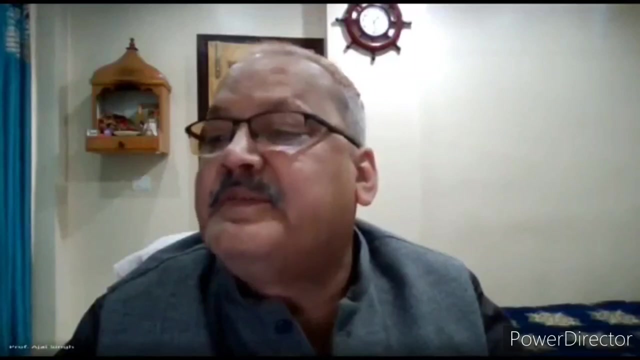 the better is the results or better is the you know assessment results. Yes, one more question was there from Amit Raj Sir: how to assess that Artificial impact of climate change on water resources? How to assess artificial impact of climate change? 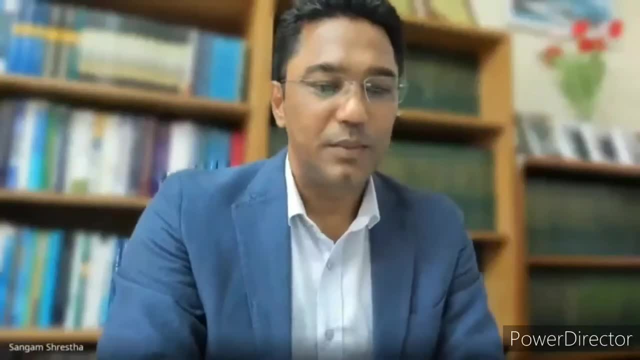 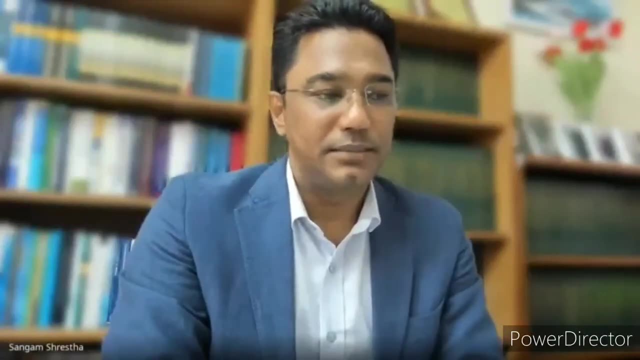 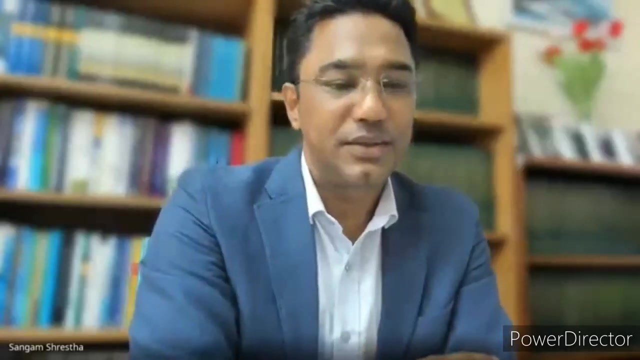 Yeah, Right, right, Amit, I think. the artificial impact, you mean the impact caused by the human activities, right, Yes, sir? Anthropogenic impact, right, Yes, sir? Yeah, that's good, That's very good question. 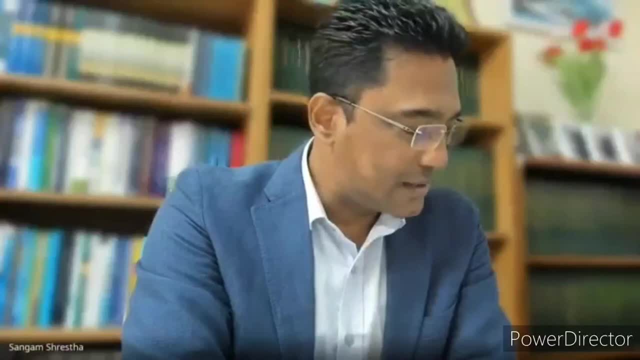 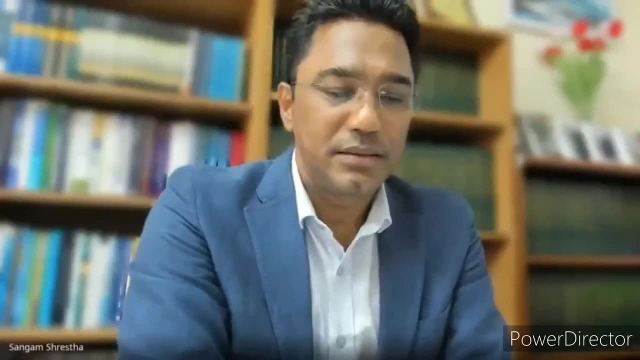 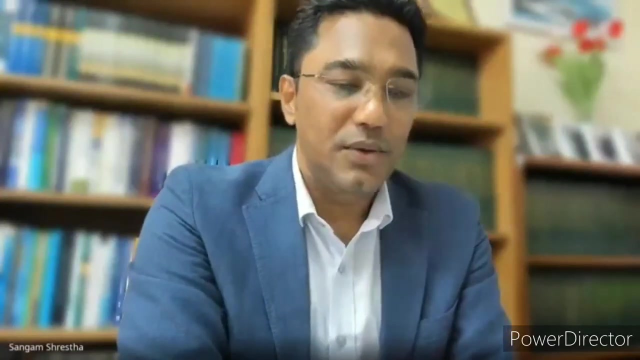 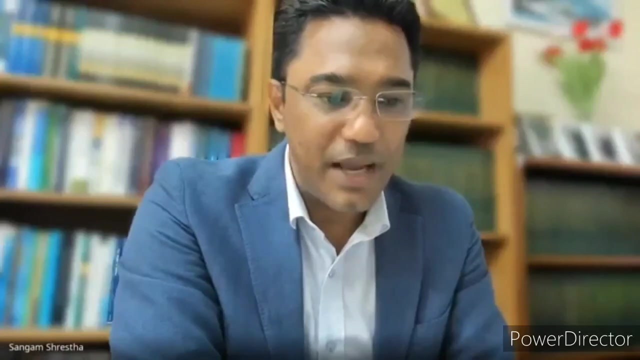 Yeah, so there are several, you know, anthropogenic activities that will impact the hydrology and water resources, right, Okay, so I read your question again, but it looks like your question is related to how to assess artificial impact of climate change on water resources. 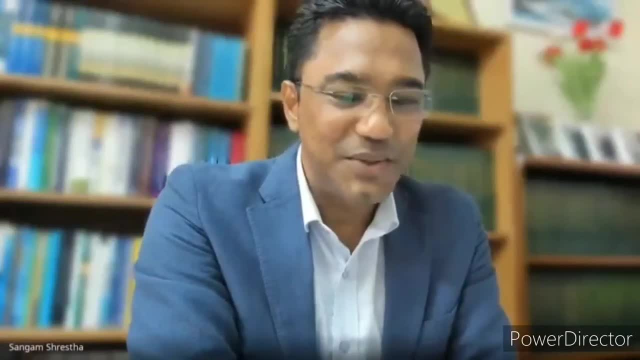 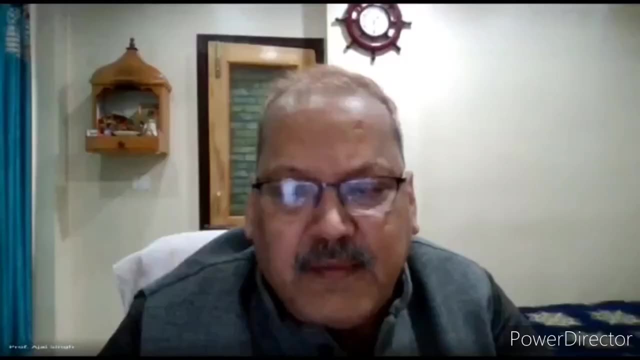 Maybe I misunderstood. Do you want to? Yes, sir, Do you want to? do you want to say that anthropogenic impact of Amit? you can unmute yourself or you can talk to me. I did mean the same, sir. 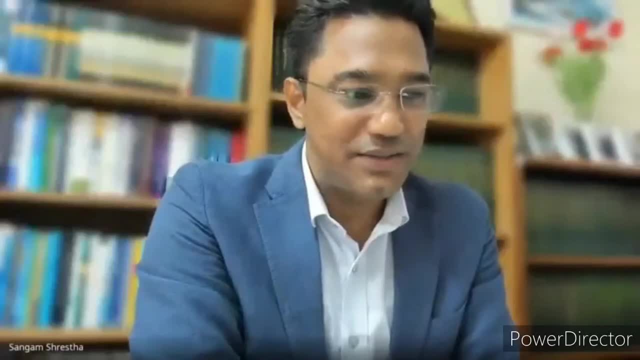 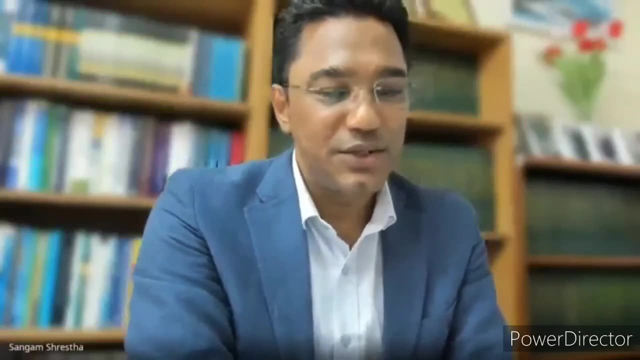 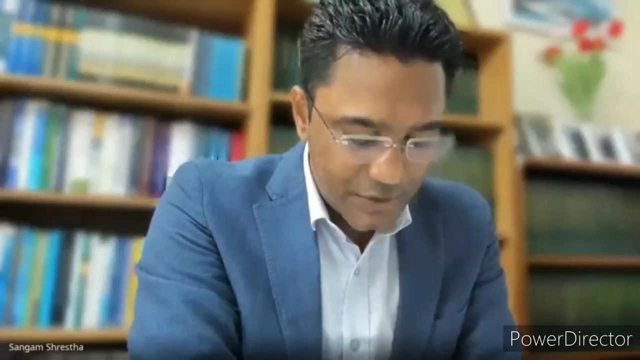 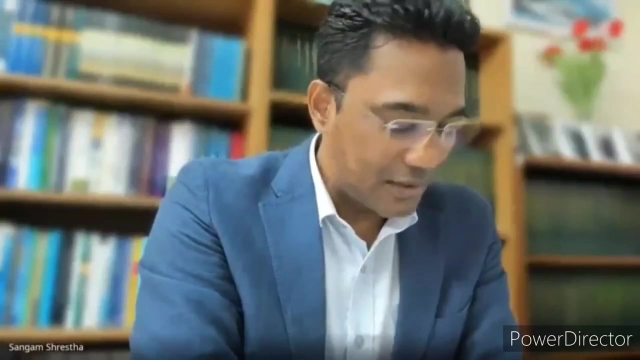 Anthropogenic impact. I see It's not the climate change, right? Yeah, you know, the recent climate change is due to the anthropogenic activity, right? It's not the natural, The rate of the increase in the temperature. it is very, very high because of the anthropogenic, you know, greenhouse gas emission. 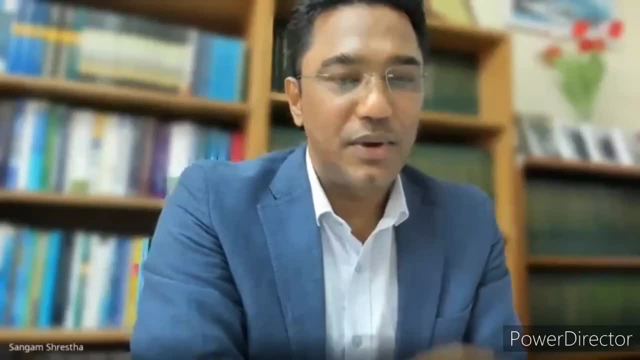 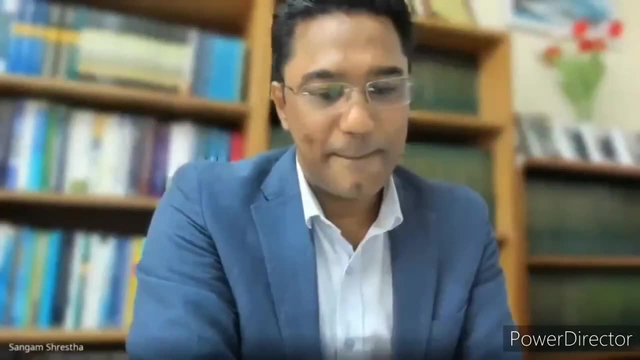 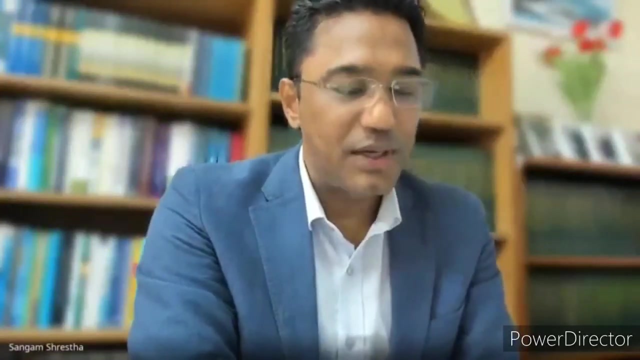 So that's the different part. But I think your question is related to how to estimate the anthropogenic impact on the hydrology and water resources. So there are several activities right. One is the construction of the dams and reservoir, The other is the conversion of the. 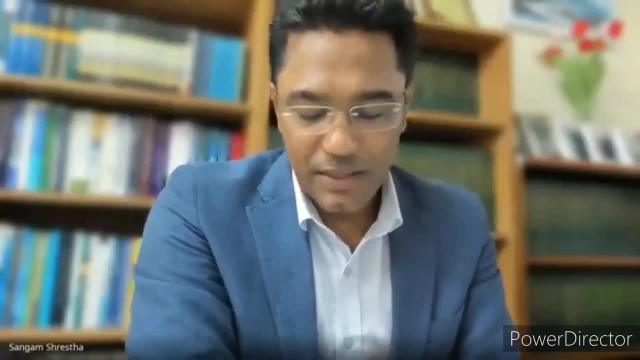 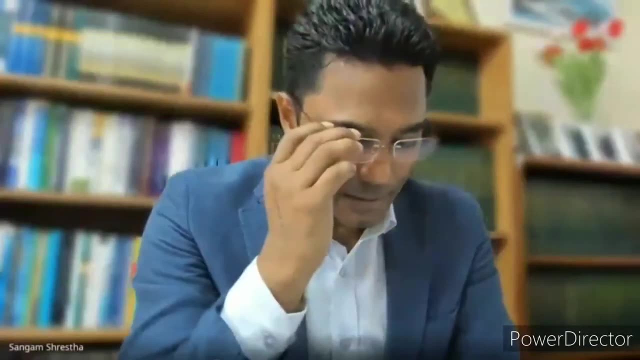 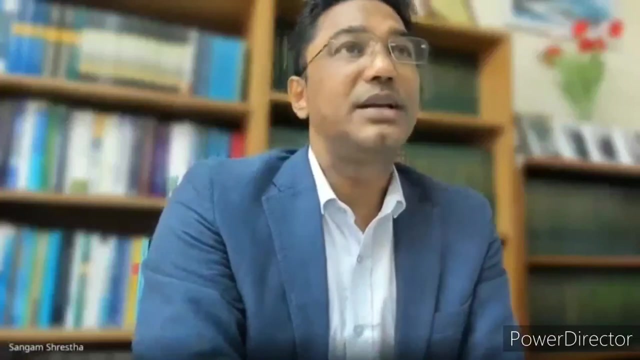 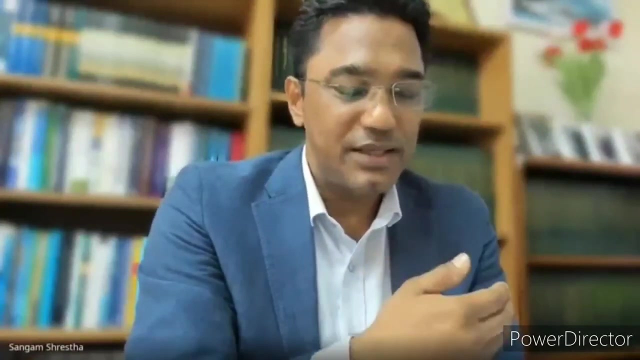 Land use and land cover, for example, conversion of forest area into agriculture area, right. So, you know, in the model we are using the hydrological model or any other kind of water resources systems model, right. So in those models you can, you know, create some scenarios to change the, you know, land. 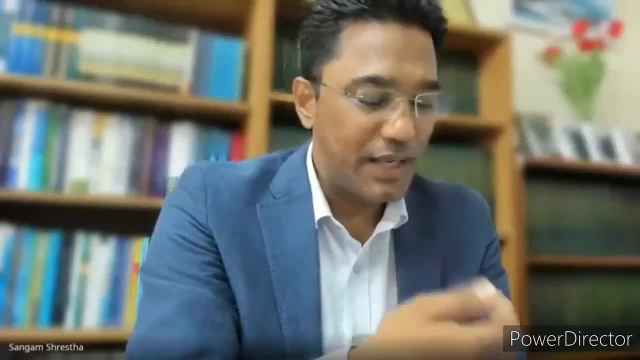 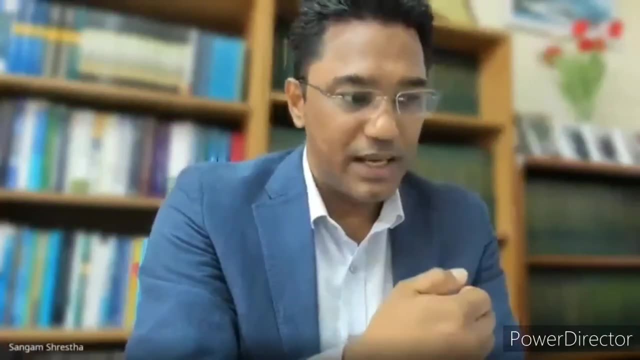 use and land cover. right In SWAT, for example, You can change the land use and land cover from forest to agriculture, From forest to you know urban area. So if you are using this SCS curve number method and you can change the curve number, 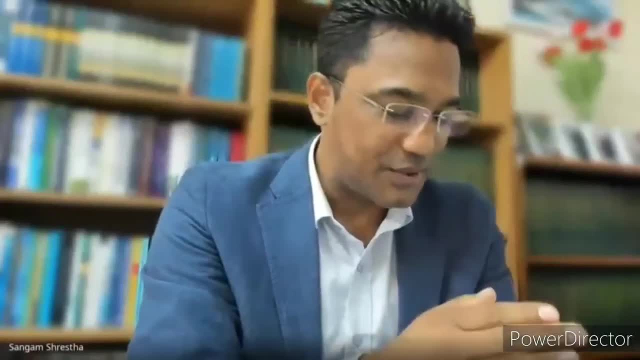 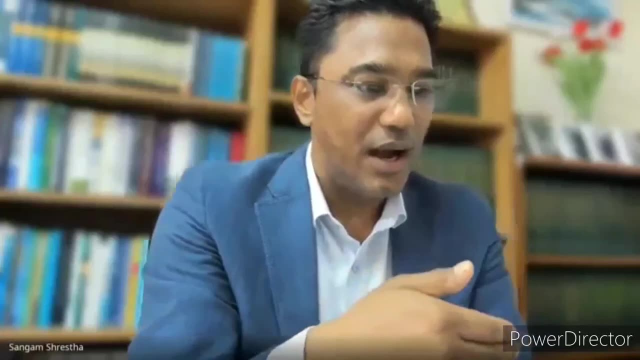 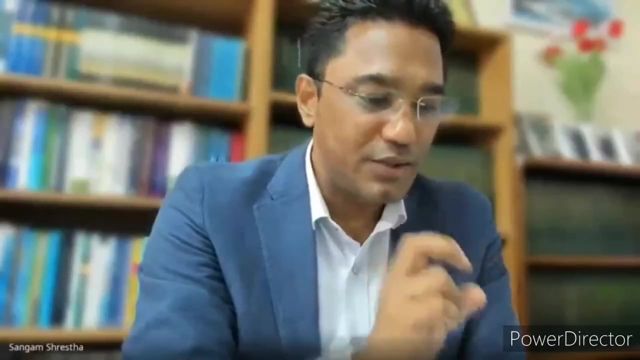 that represents the change from the forest to agriculture, forest to, you know, urban. And when you simulate that gives you how the land use and land cover change impact the hydrology, okay. Similarly, In the SWAT, there are several, you know, water storage module or reservoir module. 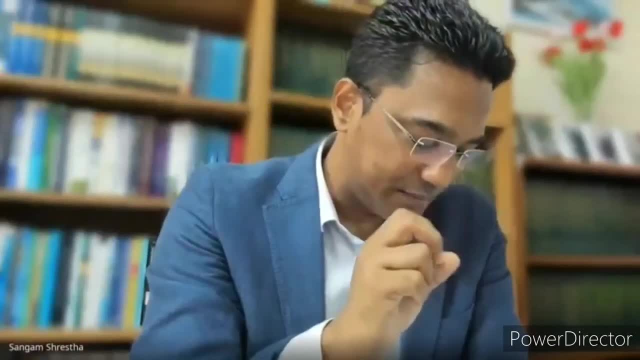 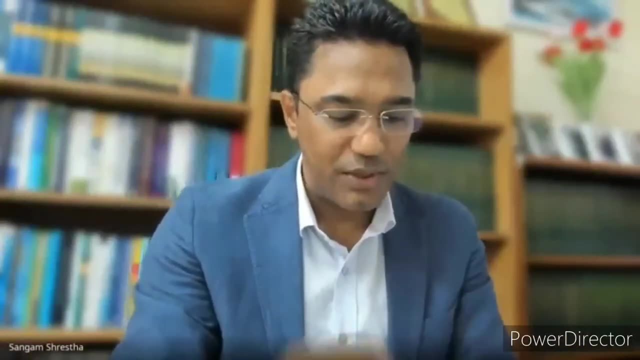 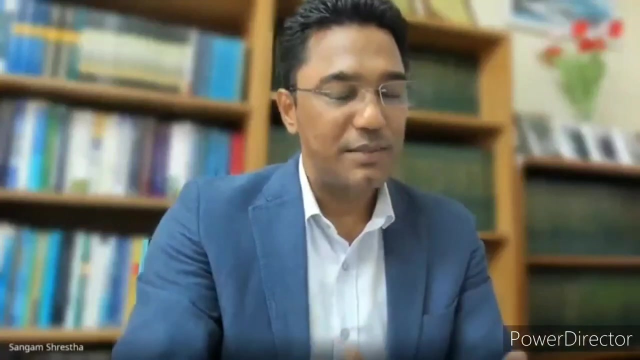 So when you develop the SWAT model or set up the SWAT model in the area where there is no reservoir, you put the reservoir in the SWAT model And you simulate the- you know- SWAT model and you can see what is the impact of you. 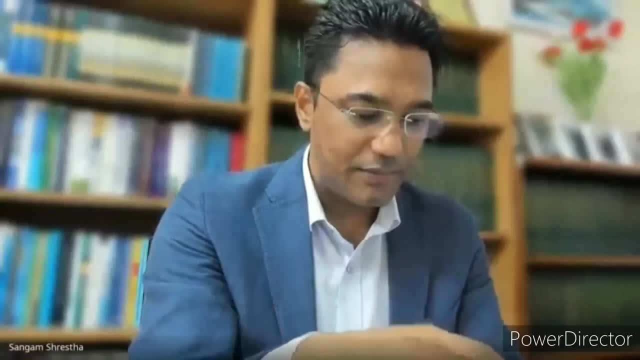 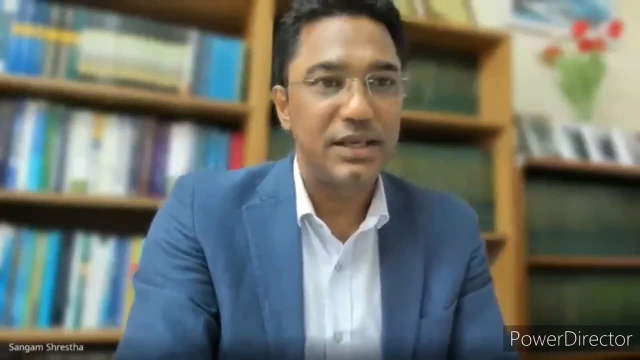 know, construction of the reservoir of different sites. Okay, Thank you, Thank you. So that's we simulate how the anthropogenic activities impact the hydrology and water resources. Is that clear, Amir? Yes, sir, Thank you sir. 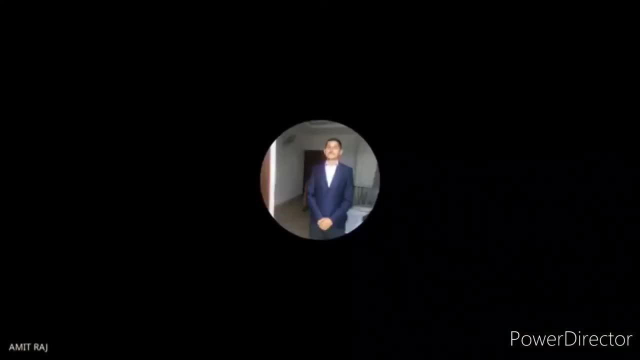 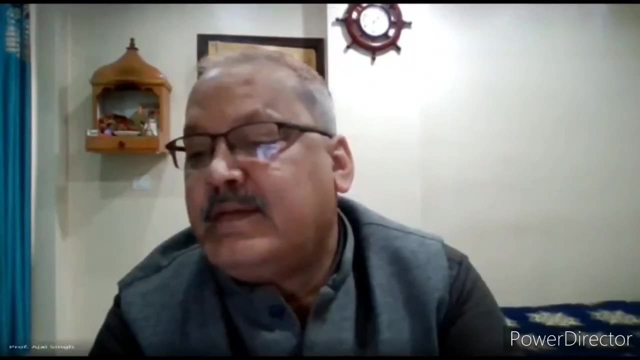 Okay, Okay, Okay. I see that another question from Bala Sundaram Right. Is there any possibility of analysis? temporal analysis or any kind of analysis of the environment damages a natural resource. Do they have to be done carefully And are they Shanmugas in the area? 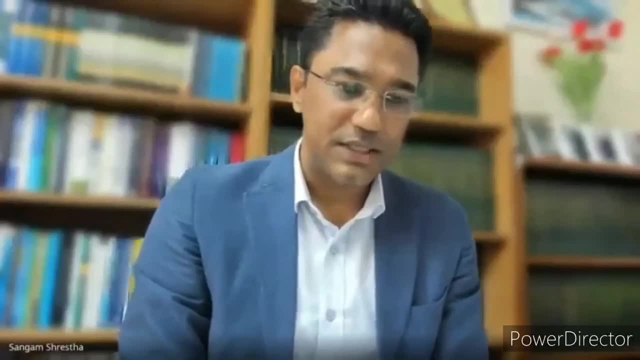 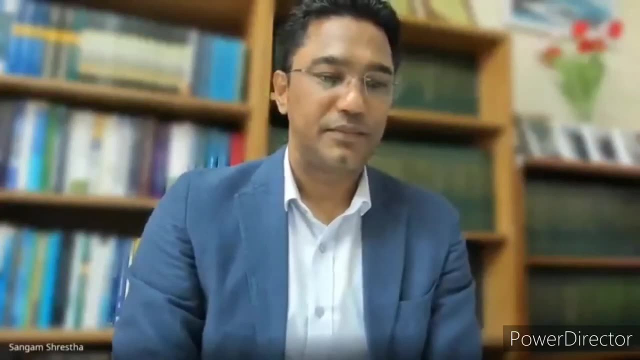 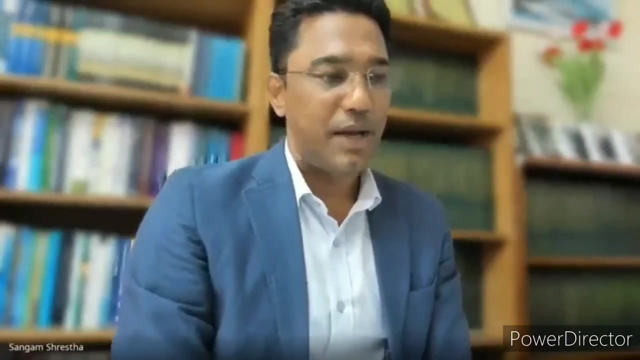 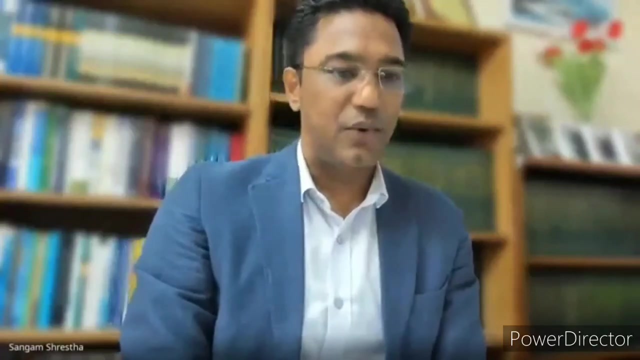 Yes, Yes, temporal changes in a particular areas by using any model. yeah, I think SWOT model is a continuous process based model, a bala. so a SWOT model gives you the daily, you know, changes in the flow, right? so it means that if you have the 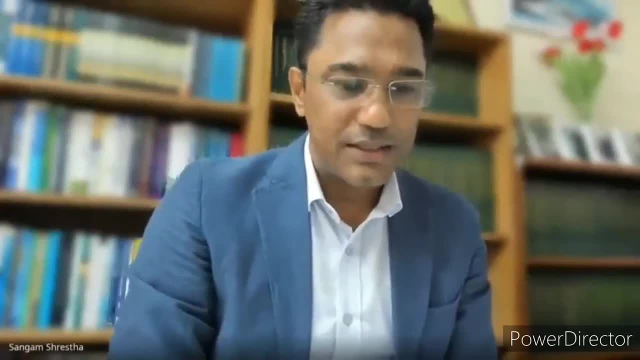 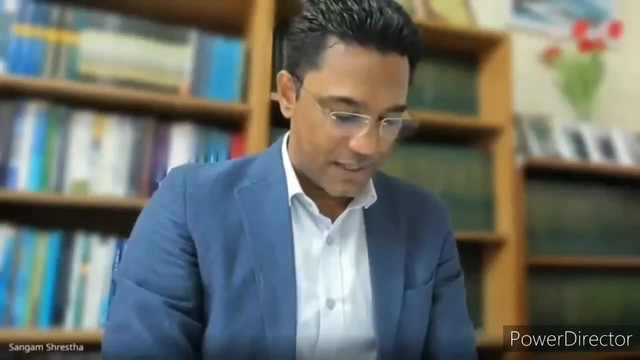 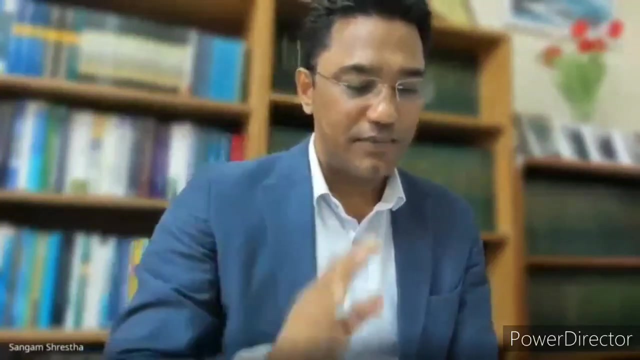 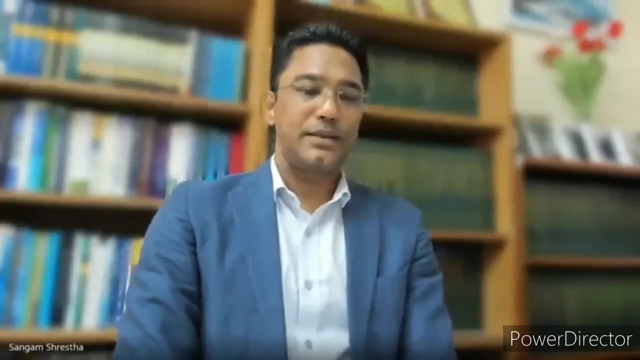 daily changes in the flow. you can do analysis of the temporal changes. know, and it has the special unit you know, like HR use and also the sub basin. so you have one sub basin and then you have a daily flow of hundred years and then you can easily do this temporal change. yeah, okay. 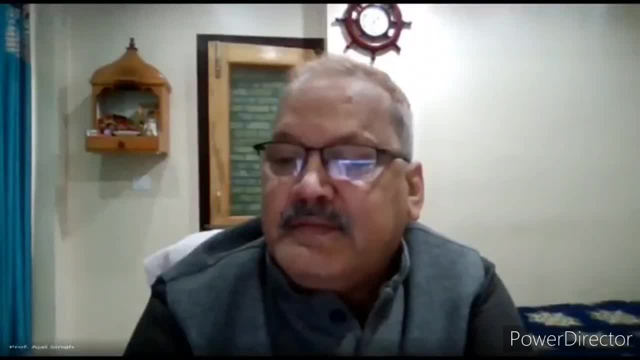 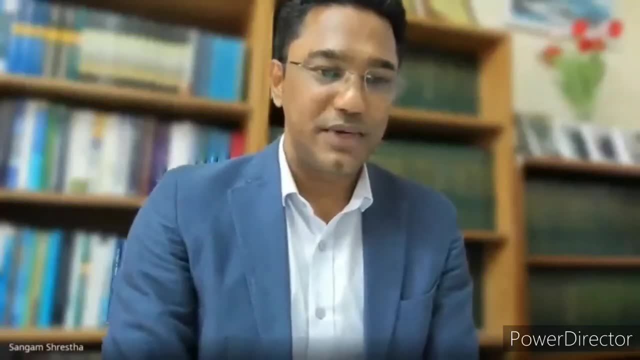 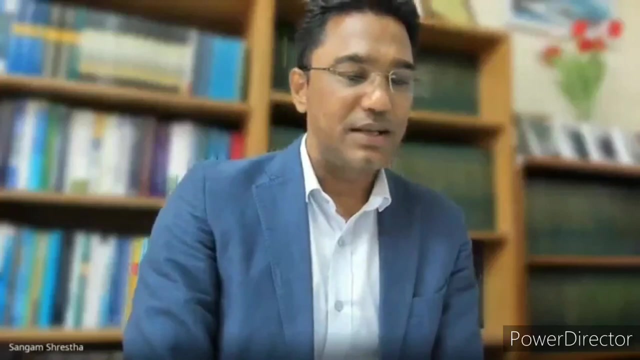 one more question is from by the body. yeah, Benita, using multiple GCM also increases complexity of projection because different DCMs are based on different assumptions and boundary conditions. is it advisable to add up this approach? yes, yes, that's true. that's true that multiple GCM increases the 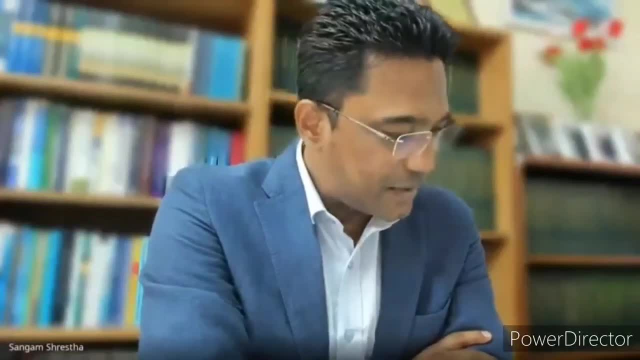 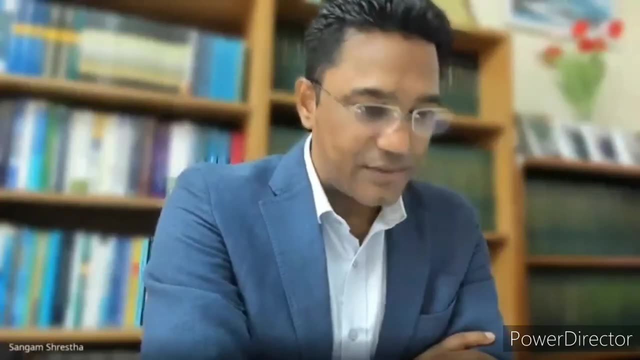 complexity of projection. that's true, but at the same time you have to also understand- you know the way it is- that multiple GCM increases the complexity of projection. that's true, but at the same time you have to also understand- you know there are uncertainties in climate change projection, right, so it's always. 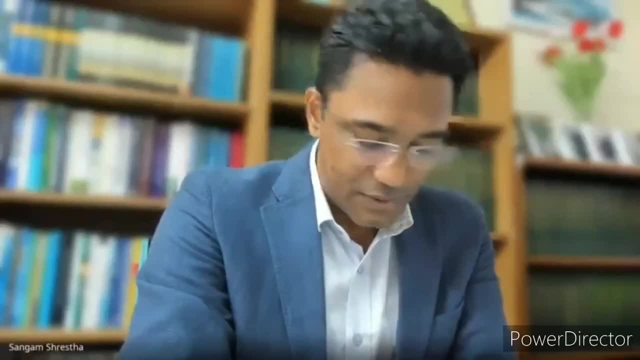 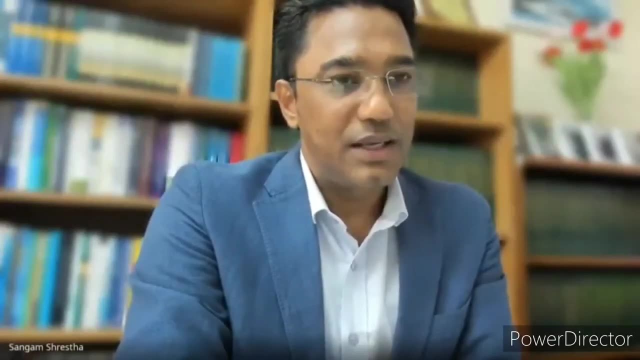 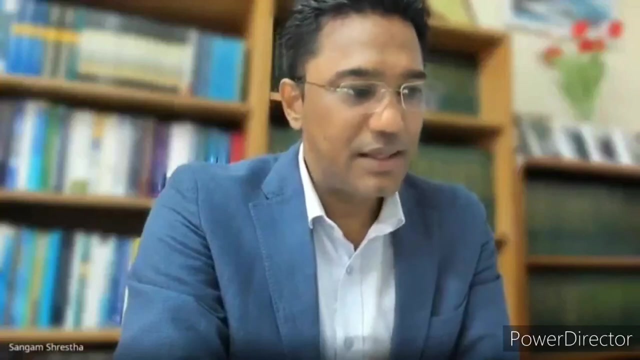 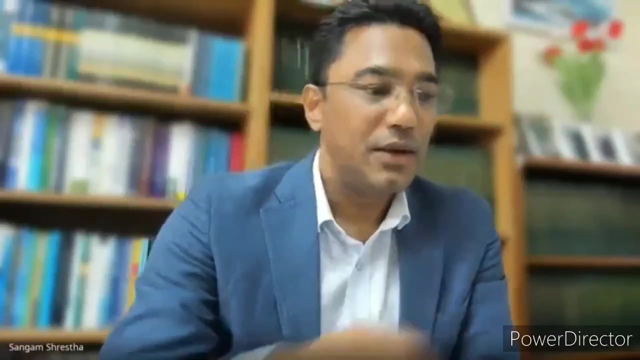 better to use multiple GCMs to address those kind of uncertainty. yeah, it's difficult, complex, but I think there is. if you have to prescribe the policy recommendations to the policy maker and planners, I think it's better to use as many number of GCMs as possible. okay. 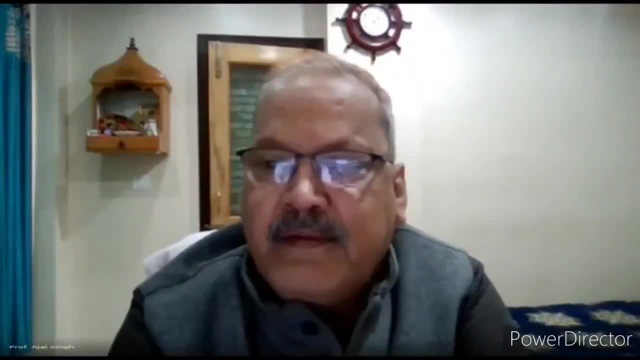 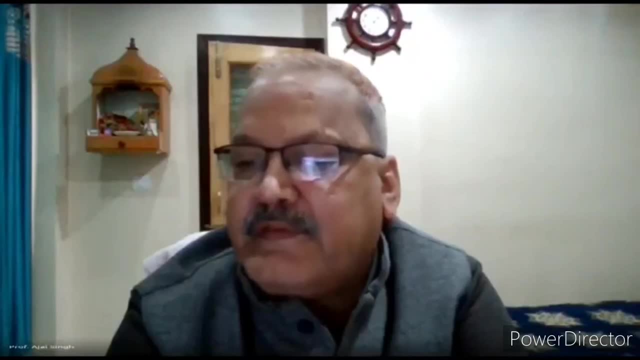 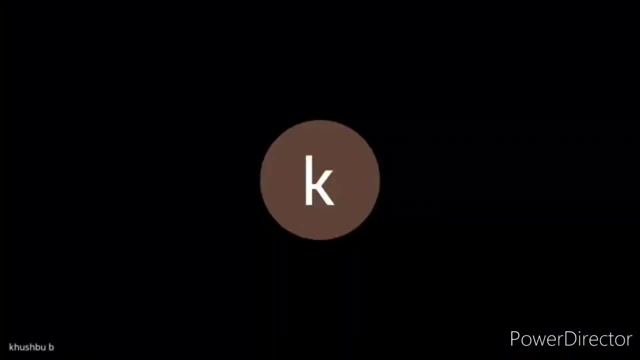 let us conclude, then, any that one question that we can take feedback form sent, please. yes, feedback form will be made available from AICT and you have to give on the website. let me talk to them, sir, may I ask my question? I have one question. yes, sir, actually I have. 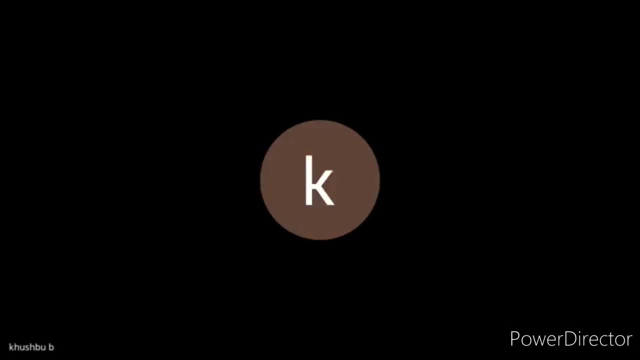 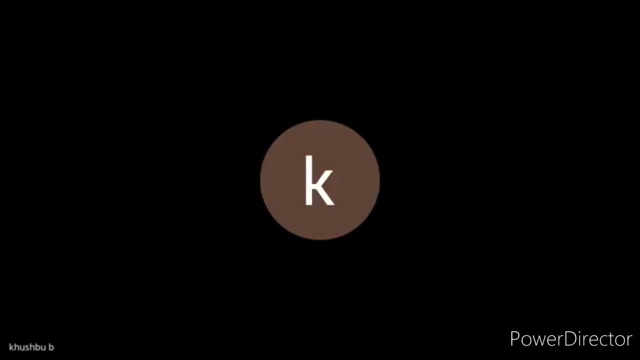 highlight like I am suffering from this problem, like where I am not able to validate my results. I am using proxy indicators, using empirical equations, but is there any other way people or like experts are using to validate SWAT model in an ungauged catchment, which is the case of Bangalore city? 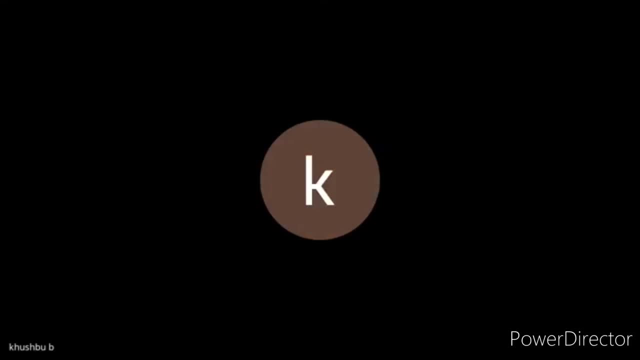 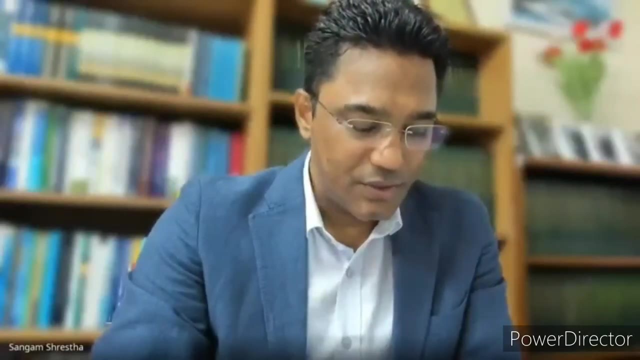 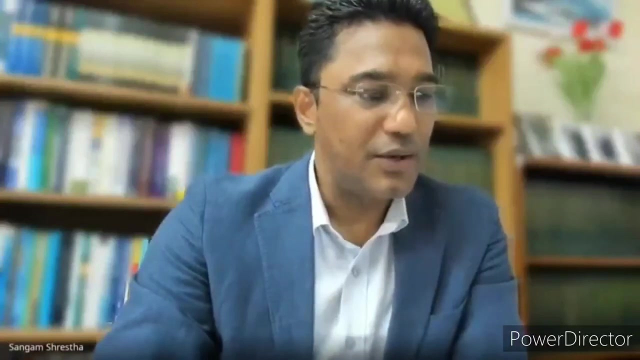 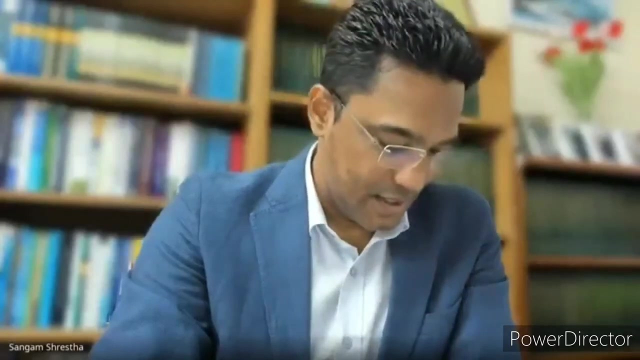 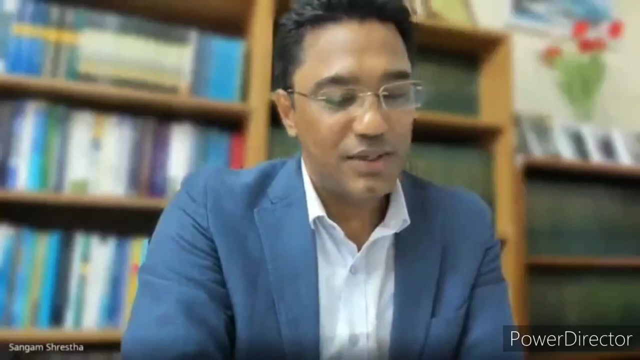 thank you. yes, so if I understand your question, you you are using this SWAT model to simulate the runoff in the urban area in the Bangalore, right, and you do not have streamflow data, right? yes, yeah, okay, you know the. the essence of the physical, the essence of the physical based ideological model is that we we use as 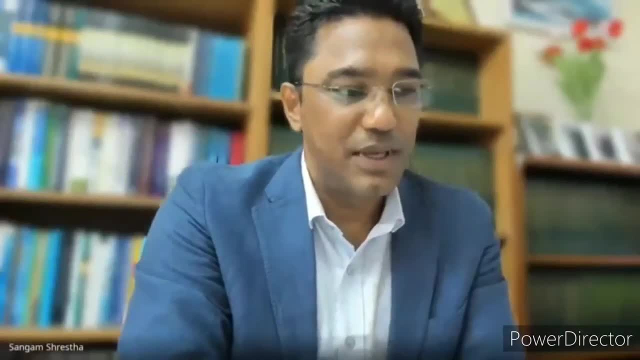 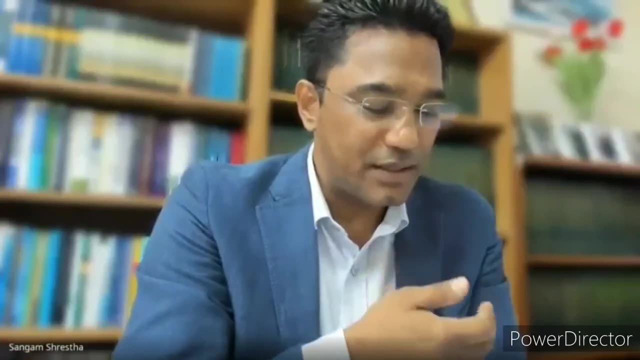 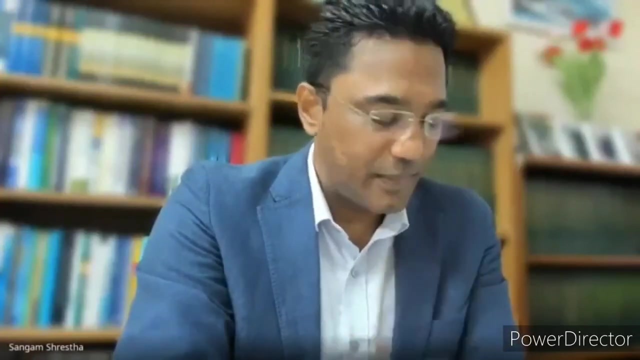 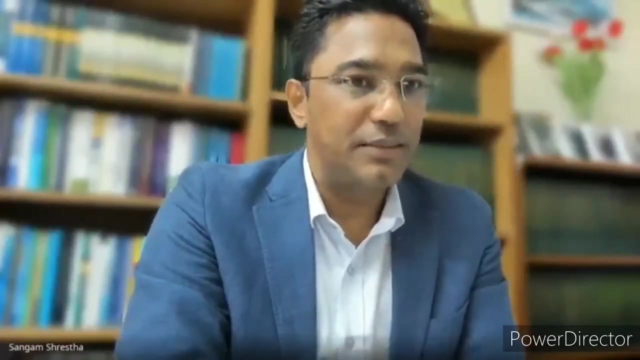 many as as less number of parameters as possible, because these are the physically based model, right? so there are several equations which are based on the physics, right? so rainfall, runoff processes, you know, groundwater recharge processes, evaporation and evapotranspiration processes, so it is on the physical process. so we, yeah, the essence of development of this kind of 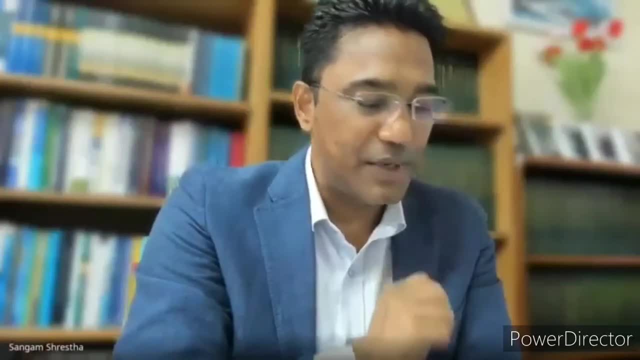 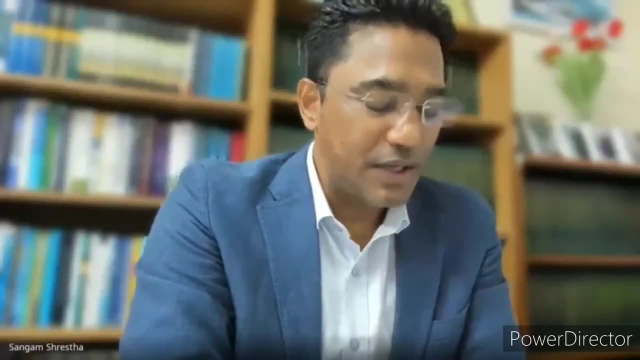 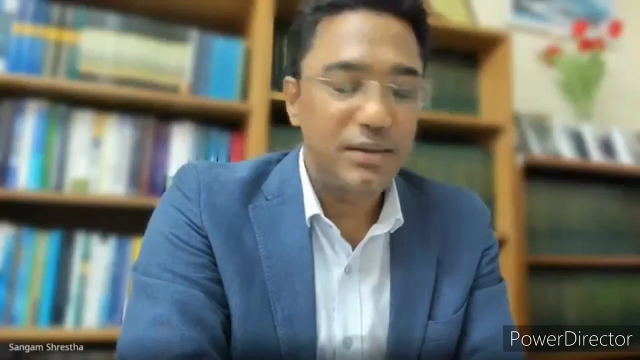 models are. we use as less number of parameters or data as possible, but at the same time, you know if you do not have these runoff to calibrate the model, one of the ways is to calibrate the other component of the water balance. okay, so you can. you can see how well the SWAT model can simulate the evapotranspiration. 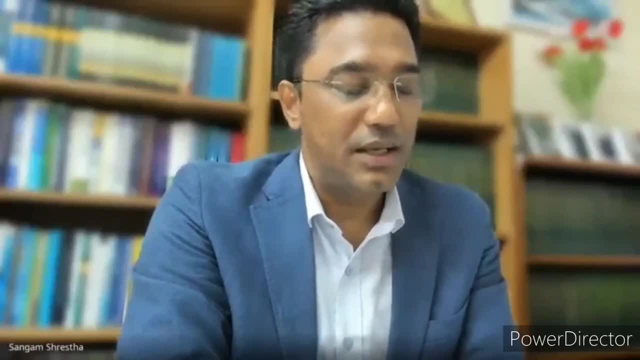 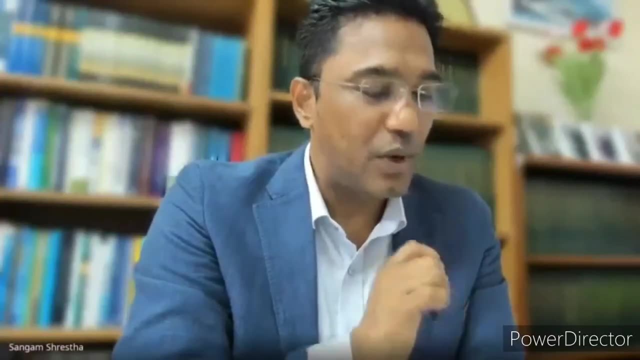 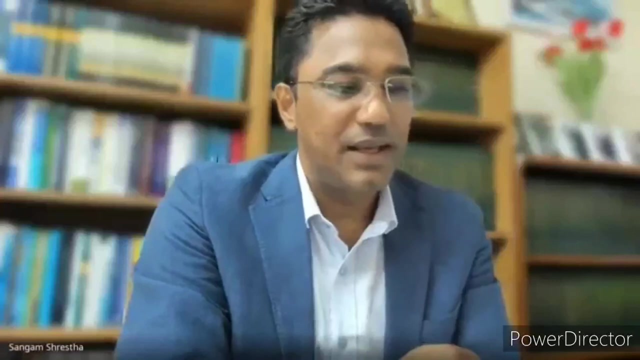 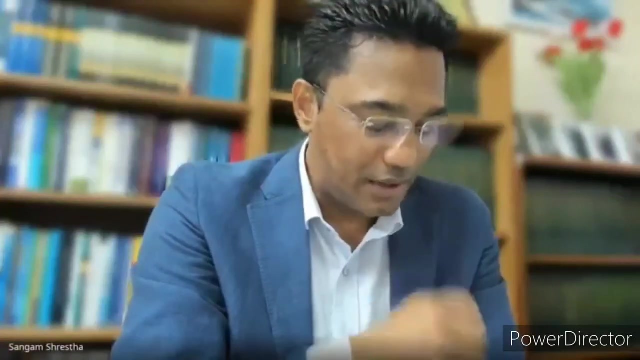 or evaporation, right. so nowadays it's it's getting popular that we also calibrate the model by using other water balance components like evapotranspiration. okay, so if there is no any other alternative, I think using this- you know- evapotranspiration parameter to calibrate the model also is is valid. 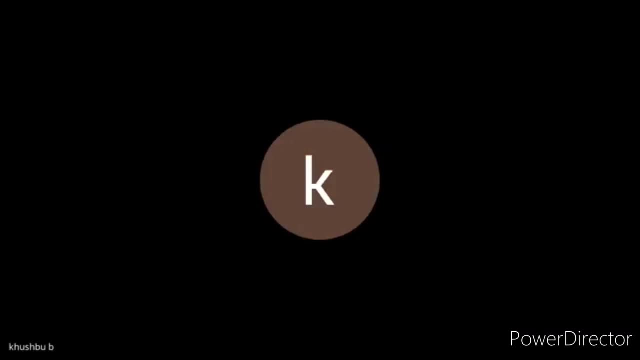 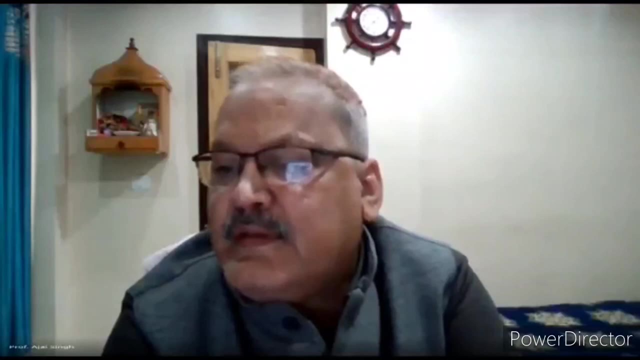 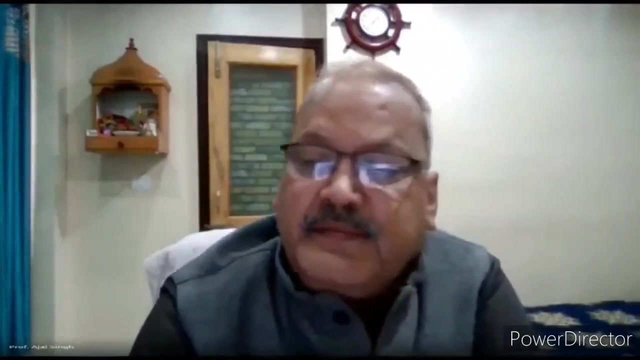 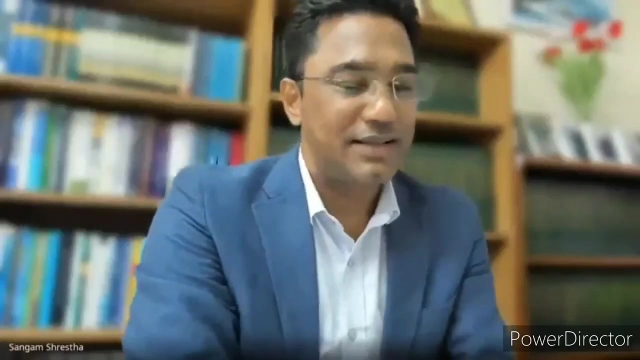 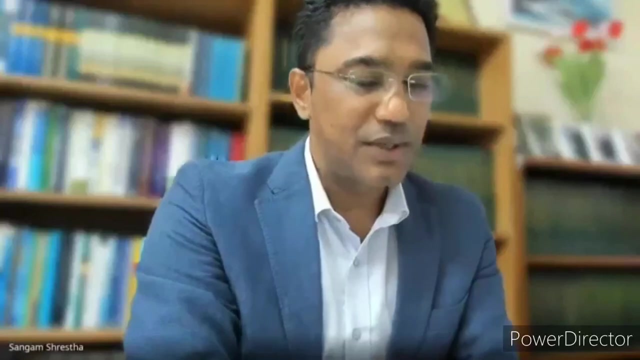 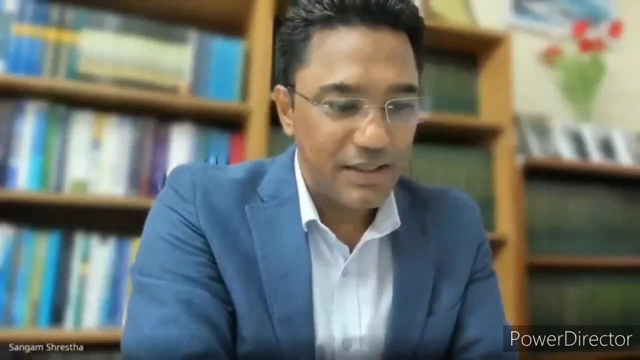 okay, so I think there is no more question. Shruti Verma has appreciated, okay, DR, I really enjoy the presentation and also the question-and-answer session. I think all the participants they are very, very, you know, impressive questions and they are very, very important questions and I'll be very happy to be. 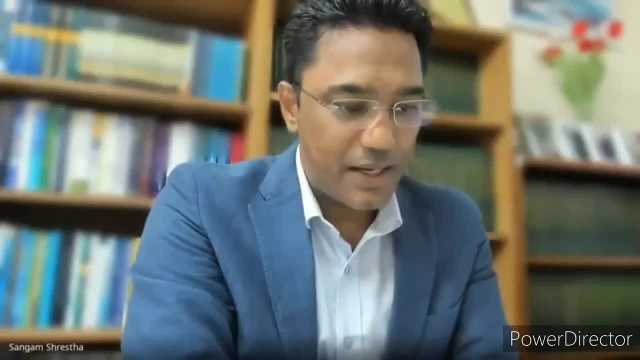 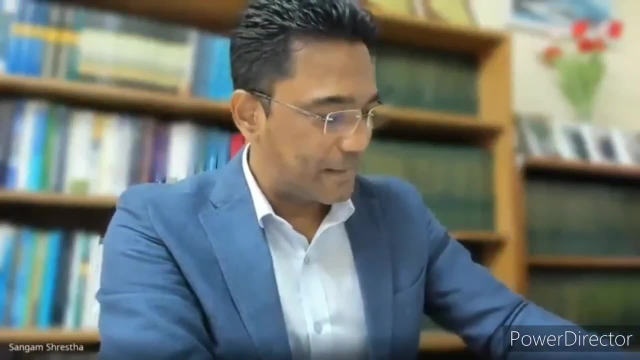 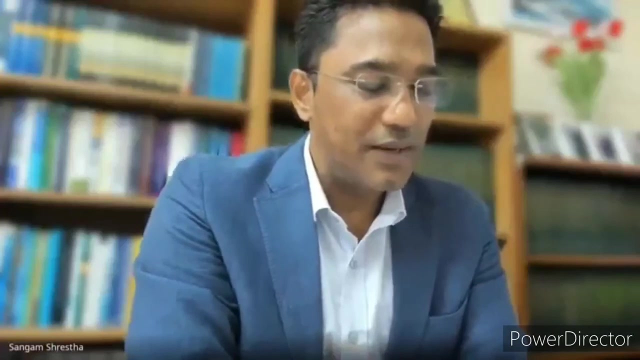 being touched with all of you. if you have any questions and also the other suggestions said want to take like to pursue your master's or PhD, I'll be very happy to help you And Professor Ajay, thank you very much for inviting me to this faculty development program. 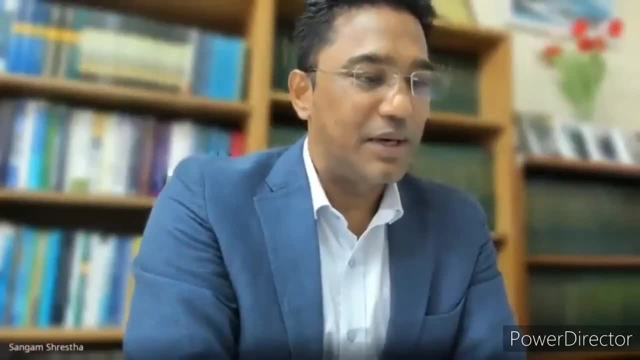 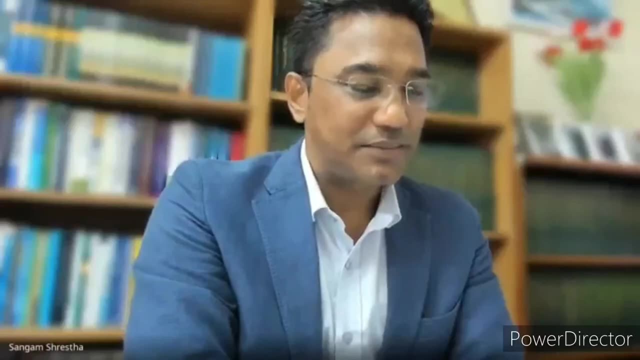 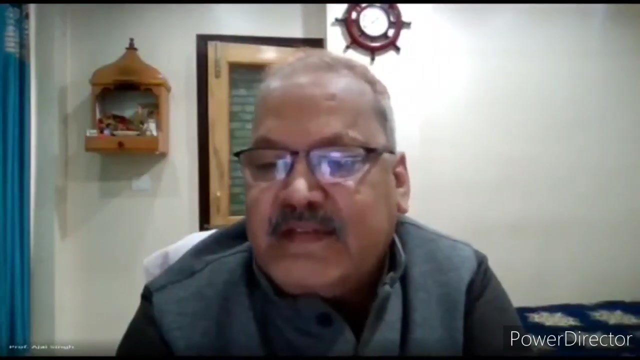 We communicate in email, but it's very nice to see you face to face. I'll be very happy to explore the collaboration opportunity. Yes, we have a wonderful session. This is our honor that you got involved with us And we hope that we will make some programs. 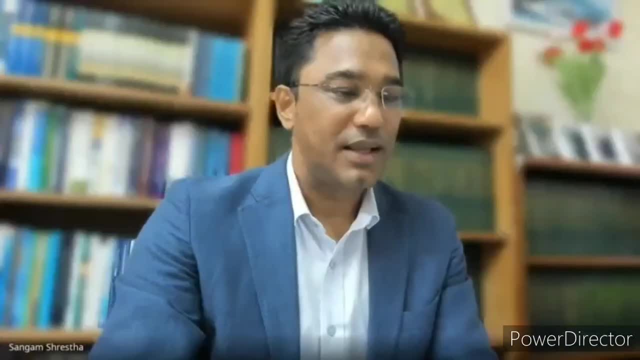 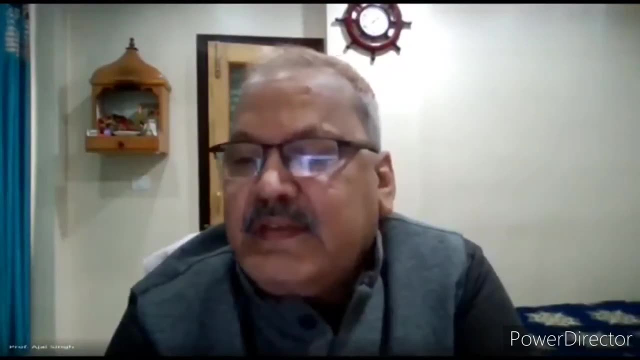 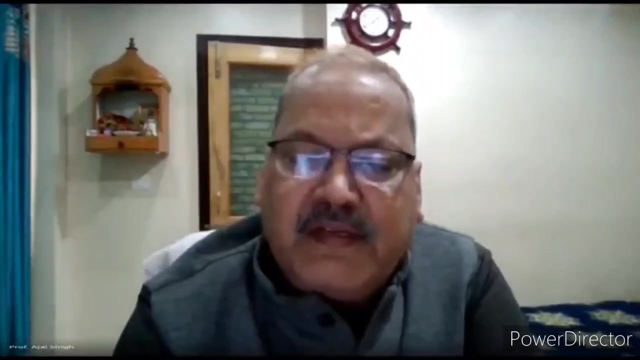 where you will be invited again. Yeah, thank you. Really, this is a wonderful group. I saw all the questions. They are not learners, They have worked on it. Many MTech and PhD students are there. That's why we have kept the hands-on on SWAT and HECRAS. 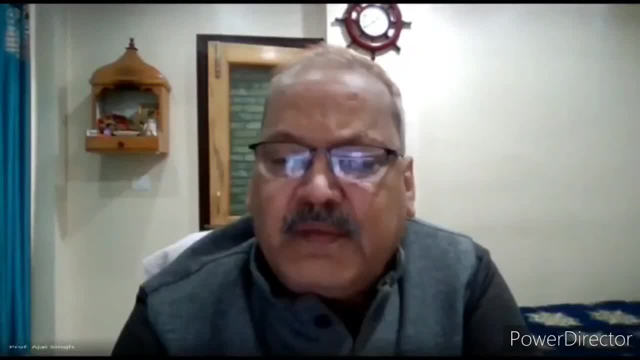 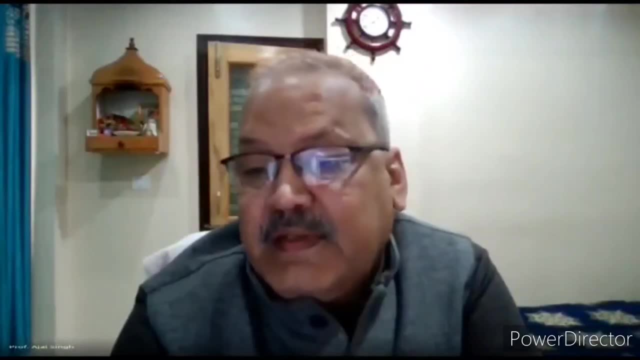 and WebModels They are. We will go very slowly. And some of the research scholars of the department they have been engaged because that hands-on will be delivered by them only. So they will not be able to do that. Yeah, that's right. 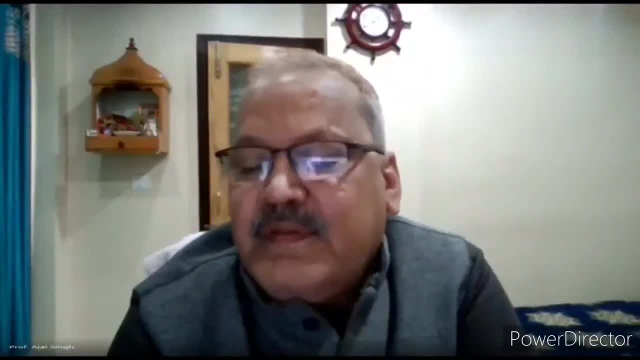 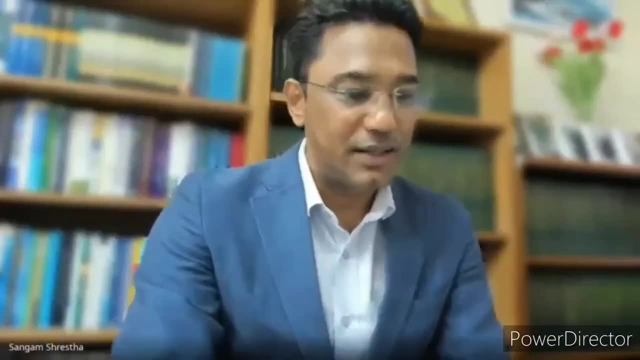 So I think, yes, many more things will come, And let us hope to get educated on this water resource modeling. Thank you very much, sir. Yeah, thank you, Professor Ajay, and thank you everyone.